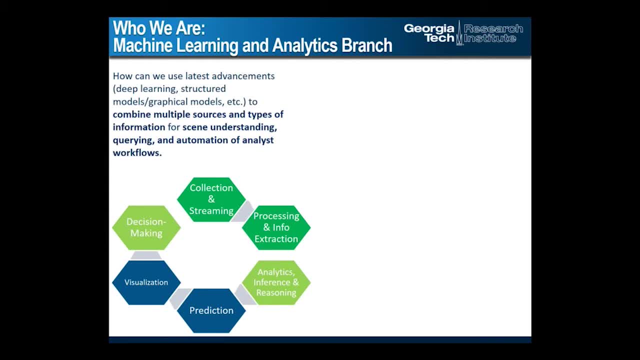 and streaming this information, processing and then extracting- or I guess collecting and streaming data really- and then processing to extract pieces of information or metadata, performing analytics and inference and reasoning to try to estimate something that you might want to actually infer from the actual information And then maybe future prediction And really. 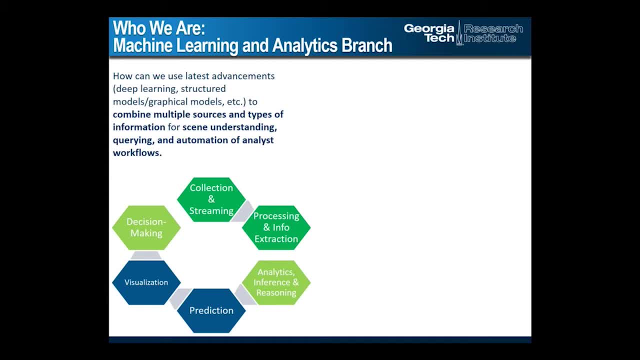 one of the things that are starting to come out. so there's a lot of machine learning and AI for perception, analyzing sensor data. We've all seen that with Google and Facebook and so on, But really everybody's turning also to decision making where you're not. 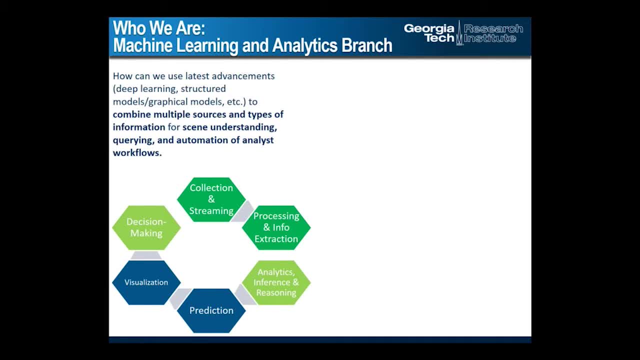 only processing data to extract pieces of information. you're also putting together those pieces of information and actually making real-world decisions, And I'll talk a little bit about that. This is some of the example of the work where we've done object detection really focused. 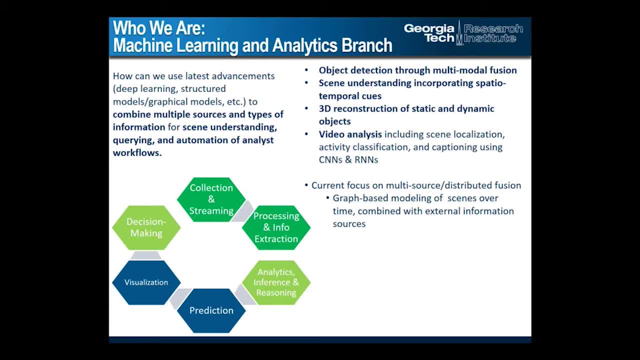 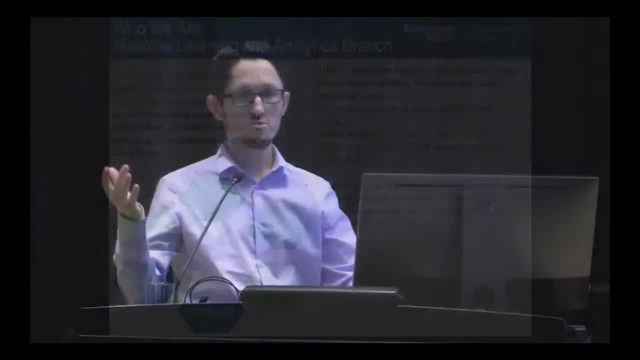 on combining multiple modalities. So these days you're never going to have one sensor. you're going to have lots of different sensors, At first maybe on one platform, but then eventually obviously distributed across the environment. And really, how can you fuse? 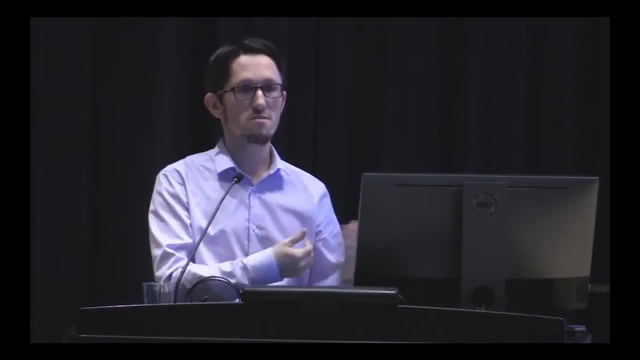 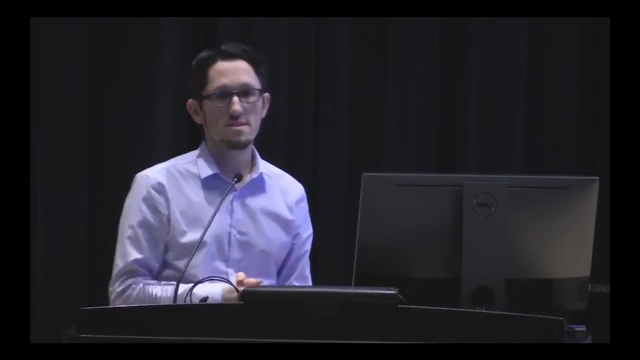 all that information to produce an understanding of what's out there in the environment in a coherent manner: 3D reconstruction, video analysis- so how can you do that? And then you detect activities that people are doing for videos and so on, And really again, we're. 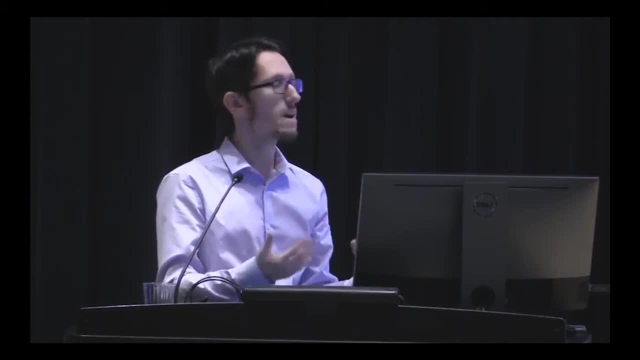 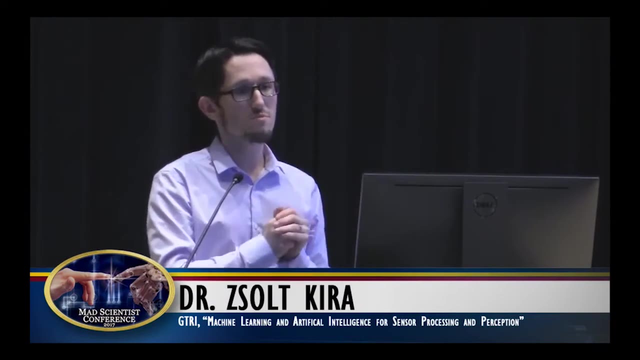 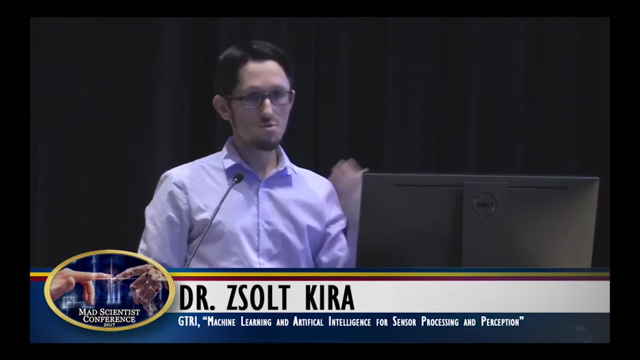 currently focused on this multi-source and distributed kind of applications where you don't have just one source of data. You have sensor data from the field. You have multiple sets of sensor data from the field in different locations. You have online data. You have 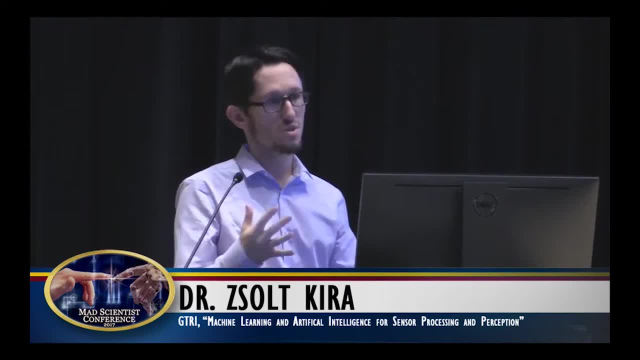 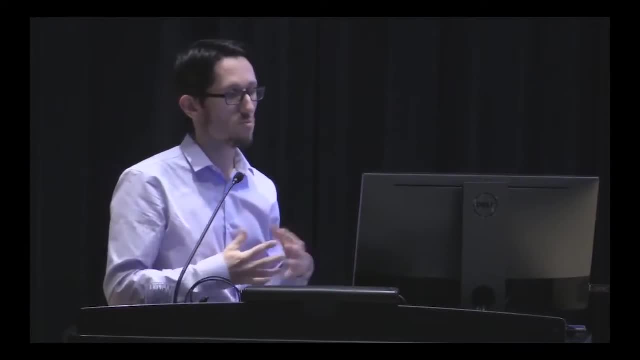 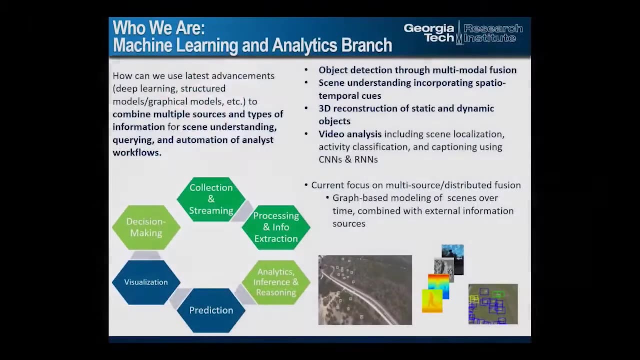 reports, You have historical data, You have all sorts of data, And how can you put it all together to perform some task that you are interested in? And really, again, key focus is multiple modalities, ranging from 2D, EOIR, 3D sensors such as LIDAR. 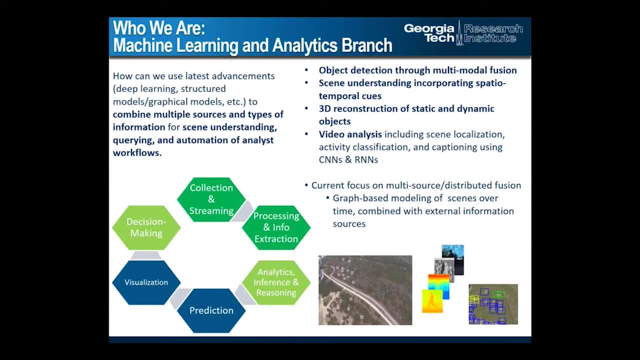 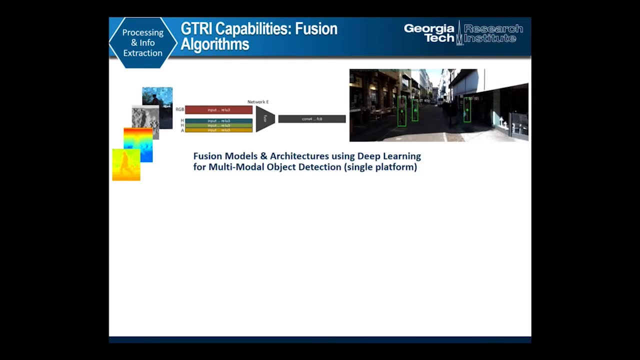 or kind of for indoor use, some of the structured light approaches and then synthetic aperture radar and kind of some of those more sort of modalities that have really been addressed by industry, which are really DOD-relevant sensors. I'll go through quickly some of the things that we've done. This is showing some object. 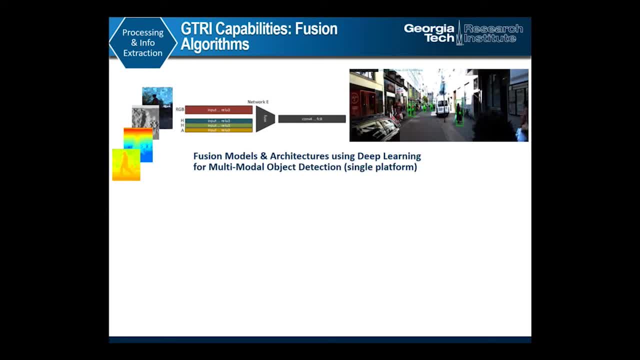 detection, pedestrian detection and difficult clutter environments. And really the key is- I'm not showing this, but we're actually fusing LIDAR and imagery to do better than just individual sensor And really we perform the research on where exactly do you fuse? 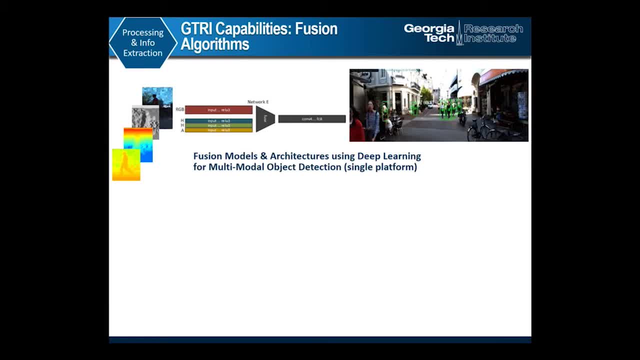 this information? Do you do some processing on each modality first and then extract some kind of mid-level information that's abstracted already- that's not raw sensor data- and then fuse it, which actually turns out to be the case for us? 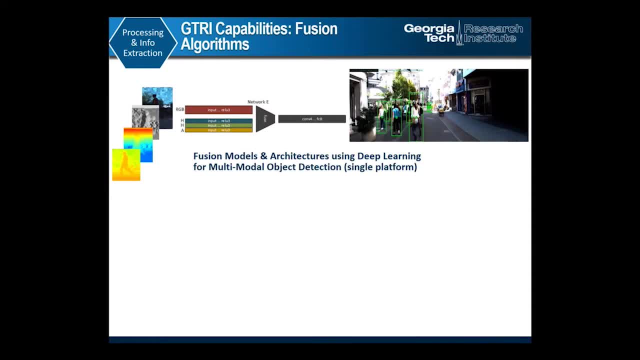 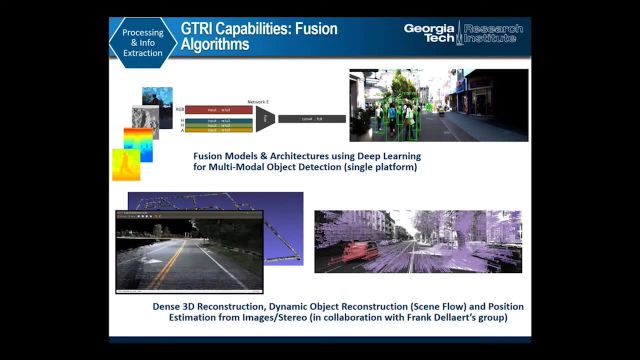 Thank you, Great thank you. So, basically addressing: where should we fuse these types of information? We've also done 3D reconstruction, So this is not a movie. It's actually a billion-point point cloud that we built from a trajectory in Atlanta. 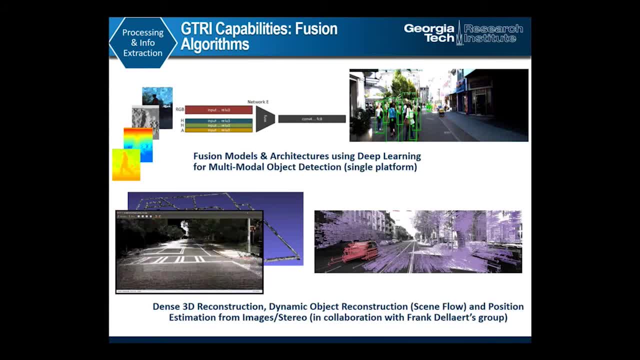 So we had a stereo camera driving through Atlanta- And this is in collaboration with Frank Deller's group at the College of Computing- And we built a billion-point point cloud. And now the question is: what can you do with it? Can you detect objects? 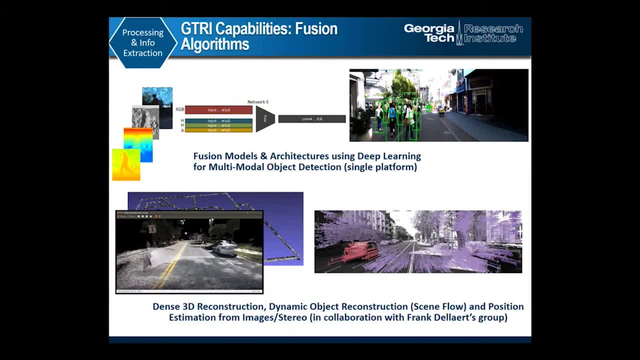 Can you automatically find anomalous objects that maybe aren't repeated Through the environment and so on? And then on the right, we're showing how can we model not just a static scene that exists, but also a dynamic object. So how can we model things that are moving at us? 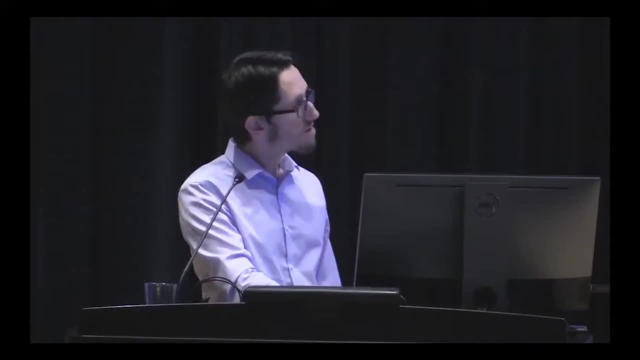 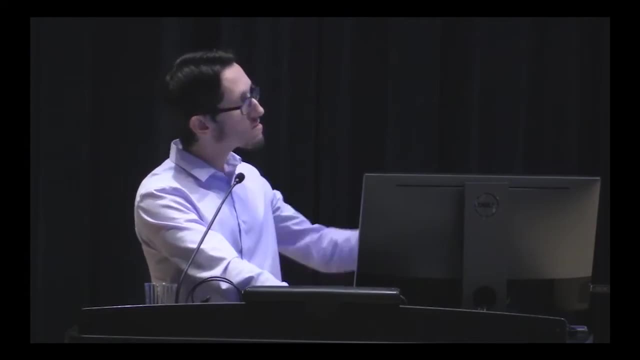 both estimate their 3D structure as well as their motion through time. Very difficult problems, And a lot of these have limitations, of still processing time, for example. But a lot of headway has been made And all of this is using some form of machine learning to perform. 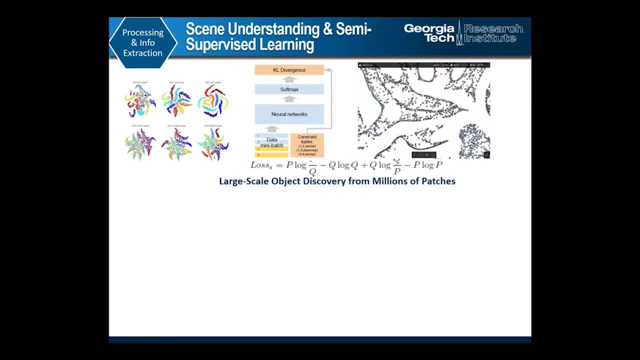 We've also done a little bit more Basic research of not, let's say, you don't have a lot of data. So all the previous examples had examples of these objects that we're interested in, Sometimes thousands of them. And the question is: well, let's say you have a data set that you don't have any labeled objects. 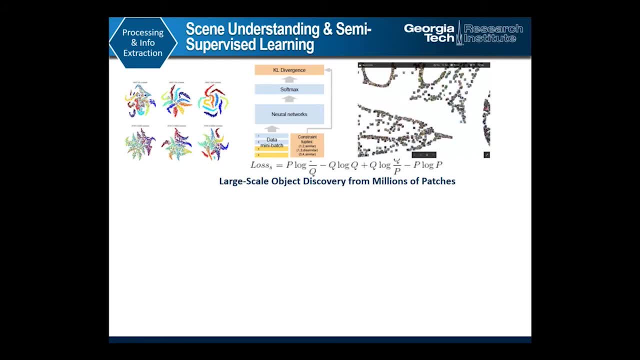 How can you automatically discover what object categories are there in the environment without having any labels? And that's kind of a key pertinent issue, for example for SAR applications, where we can barely get our hands on unlabeled data, let alone have someone label it where you know. 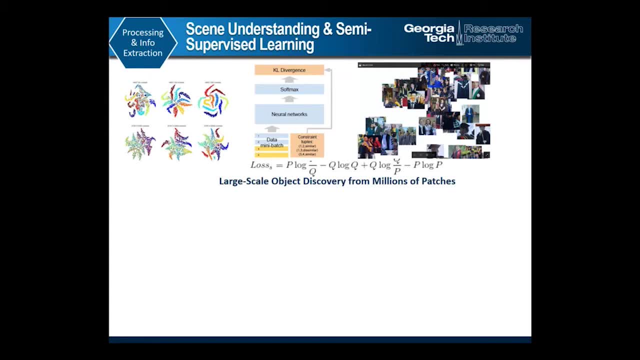 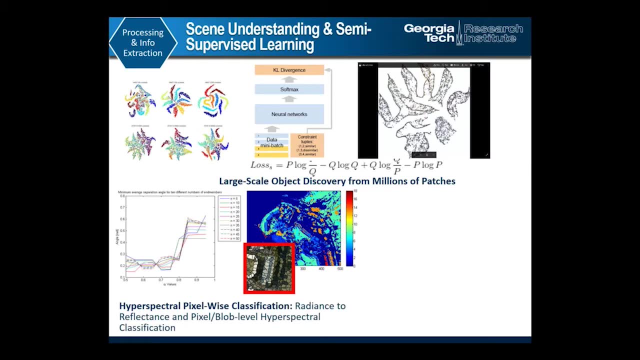 it's really difficult unless you have some images on the same environment that was collected with SAR, It's really hard to actually ground truth, the SAR data. We've also done hyperspectral processing, where you're not just. you sort of have 120 bands and you're trying to extract material classification and so on. 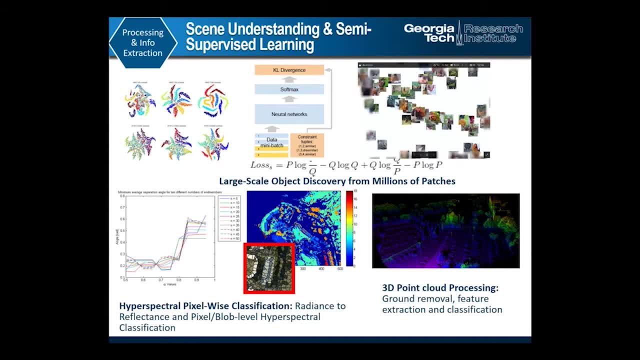 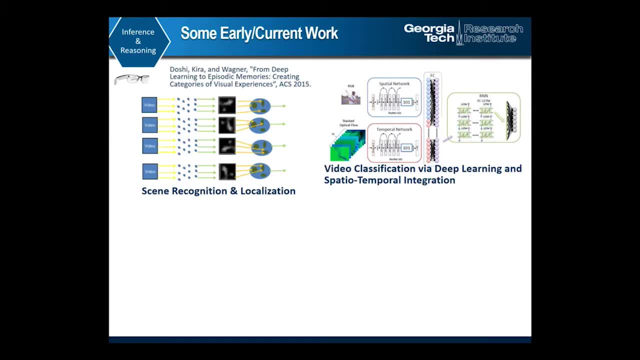 And then full 3D models built from sophisticated LIDAR sensors that we have. We've also done video processing. again activity classification of you have a video people doing or people are doing things. in those videos, What are they doing And what is not just the activity that they're doing now, but maybe predictions on what they're gonna be doing? 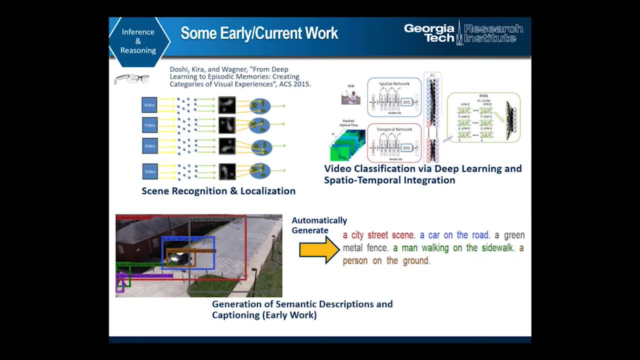 And one interesting case is also captioning. So we have, you know, petabytes of video data these days. The question is, how does someone search through it, And one approach is to convert it to text, which is something that we've been doing for a long time. 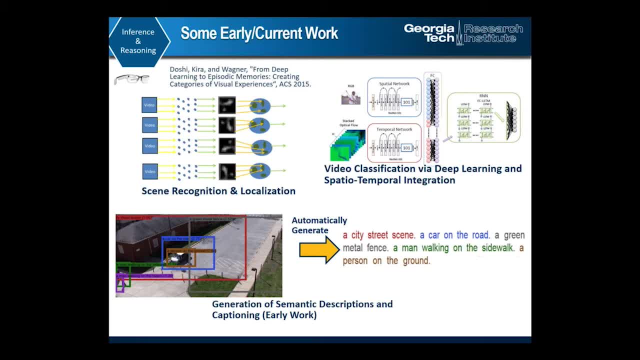 which is something that we've been doing for a long time, Which is something that's very searchable, obviously, as you know, from Google, And so what we do is we automatically take the video and generate automatically a set of text that describes the video. 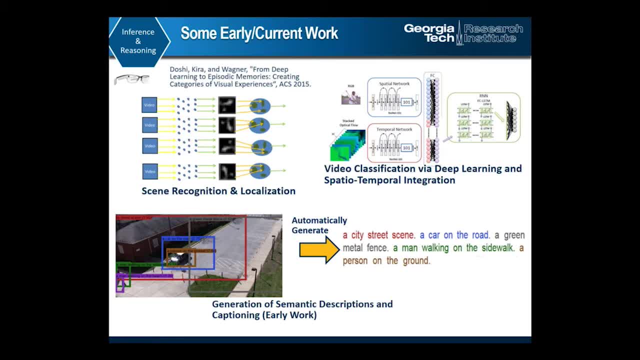 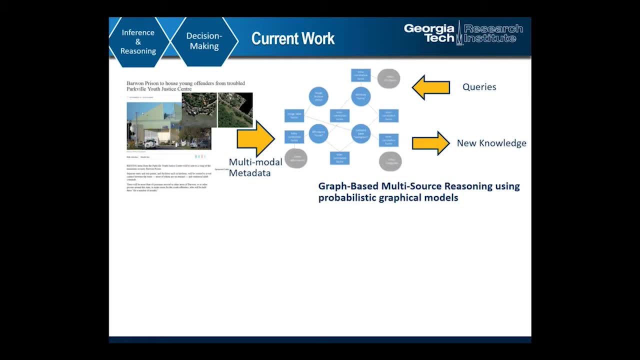 And so now, once we have all the videos cataloged via text, somebody can more easily search through it. And then finally, this application. so where we have not just one source of information, but here on the left you can kind of see it, but it's a news article, it's got text, it's got images. 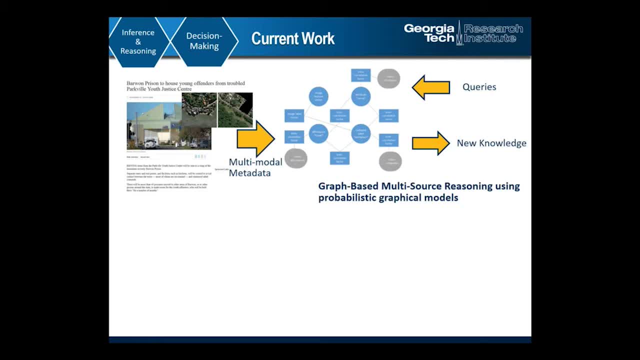 we can extract satellite imagery from it. How can we combine all that information into one representation- In this case a graph representation, leveraging probabilistic models, And how can we infer something about, for example, whether this is fake news or somehow has incorrect information, based on all the different modalities of information you have? 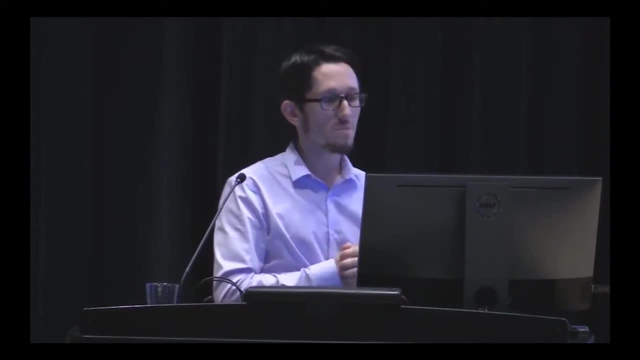 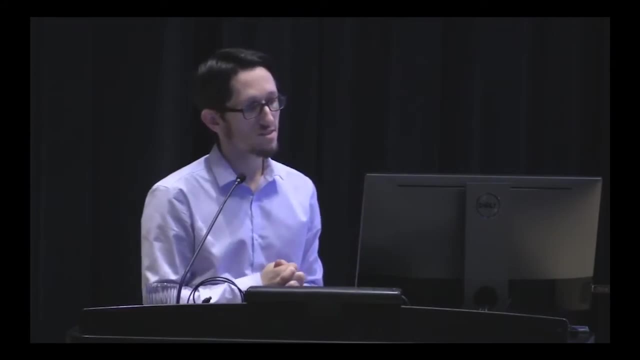 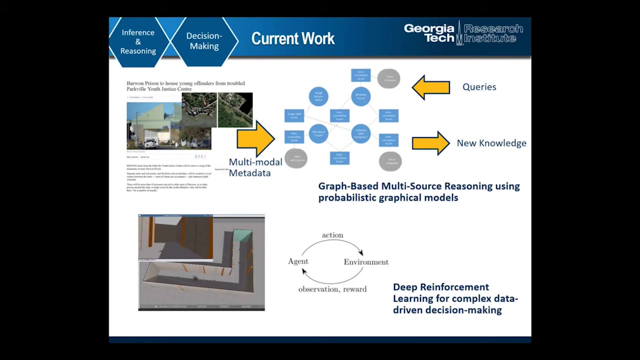 And obviously you can also extract information from the web, like Wikipedia and so on as well, And then finally Like decision making. this is still in simulation. it's a little bit more basic research at this point, but a lot of groups are working on how can a robotic platform use learning to directly. 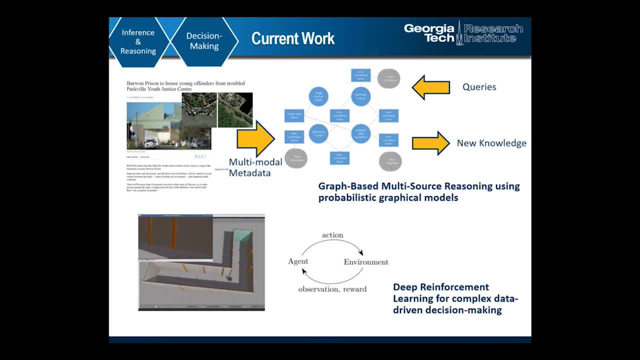 process raw sensory data and go directly from that raw sensory data through machine learning, to a decision of how to actually act for a particular task. And a lot of the techniques we're using is very similar to, for example, Google's techniques that are used for Go, to beat the human players in Go, and so on as well. 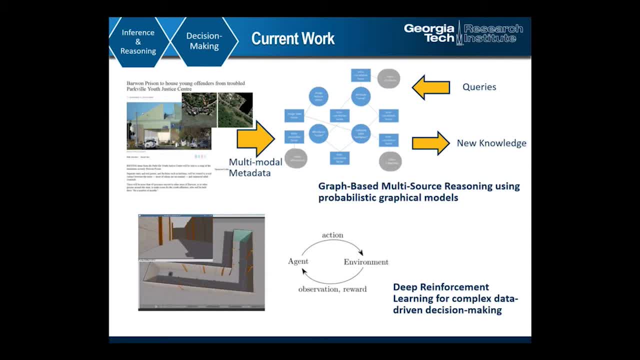 So that's kind of the if you get nothing outside of this talk, it's that really. learning has been a lot of has already dominated sensor processing. however, it's really starting to push into actual decision making, such that you can actually have AI agents all over the. 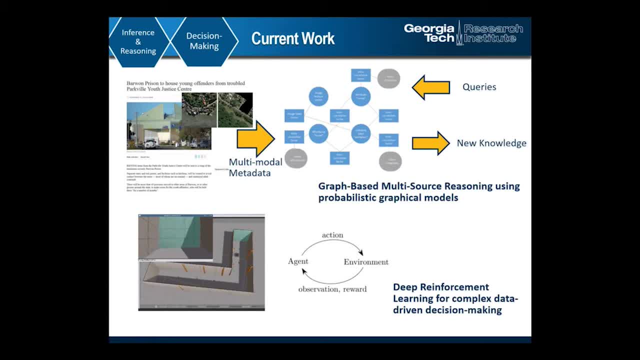 place analyzing and sorting through information and data and actually making some form of decisions, And those are some of the things that we're working on right now. Those decisions can be: how can a robot move through the environment? but those decisions can also be, for example, from Google's example, how to optimize a server infrastructure to 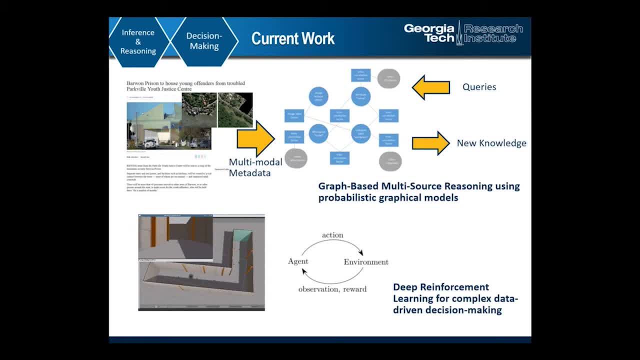 reduce power consumption? Or it could be: how can an IC analyst make decisions in terms of, for example, what source of information I want to grab next? So that's a decision that you can actually automate. So basically automating key decision points that, again, don't replace the human at this. 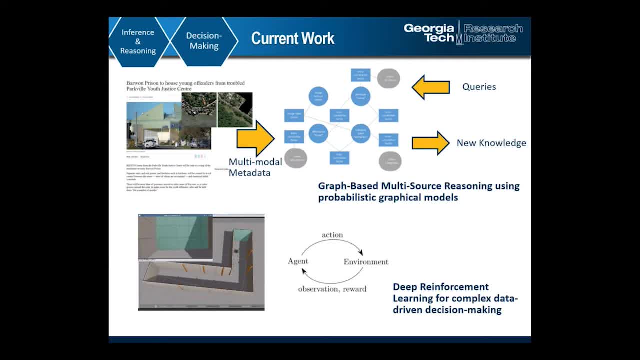 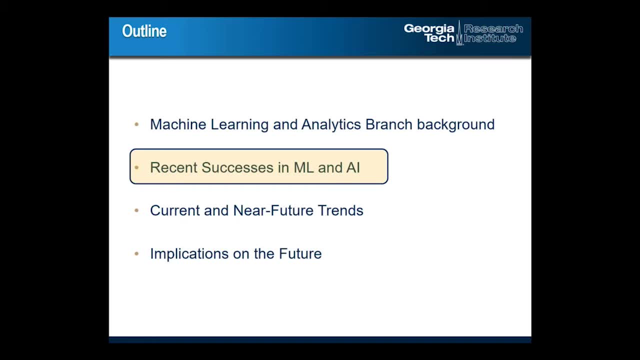 point, but really augment or aid, And I think that's a really important part of the work that we do. So those are kind of the work that we do. I'm going to talk a lot about some of the other advances that have been made, some of. 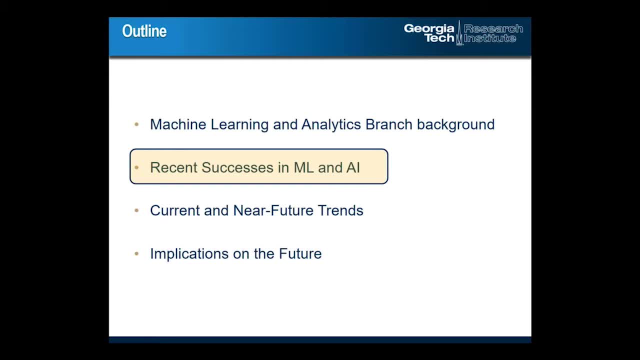 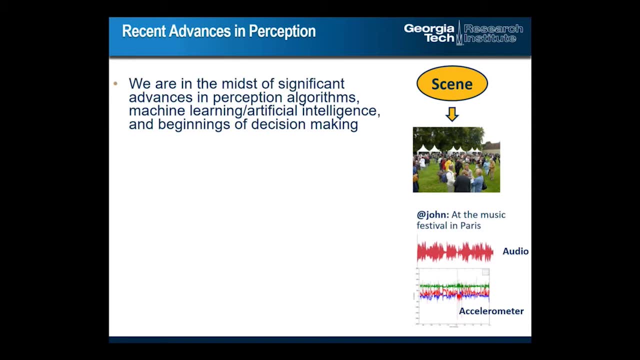 which are in other universities and academic institutions, Just to give you a more broader understanding of all the different advances that have been made in machine learning and artificial intelligence. So the key thing here to understand is we are in the midst of significant advances and these advances are again very, very important to understand. 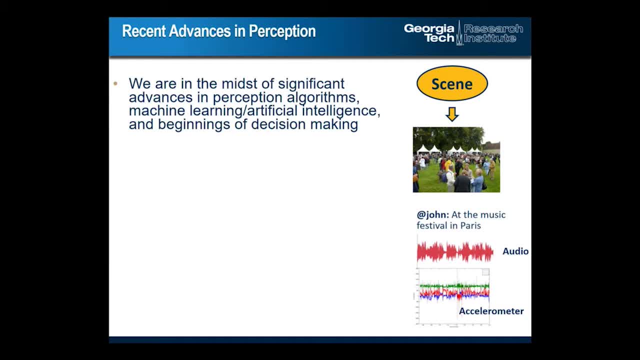 So I think I have said before five, ten years ago I would not have predicted the resurgence of deep learning, specifically neural networks, which I won't go into, but sort of a class of machine learning methods that have existed since the 80s and 90s. 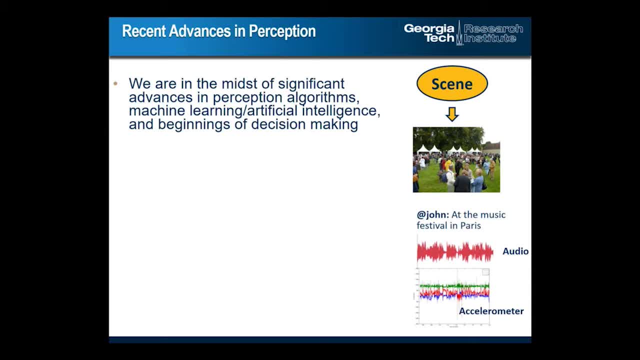 But only now have we figured out how to actually properly use them, And one of the revolutionary things about it is it's not linked to any one modality of data. The same class of techniques have now, across all the conferences, dominated computer vision. 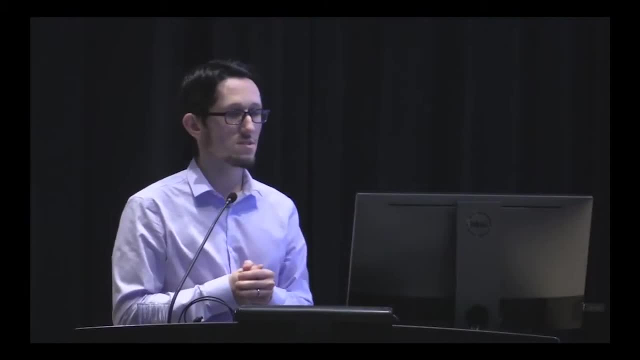 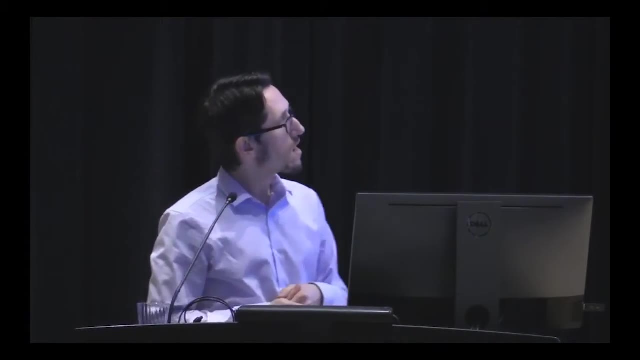 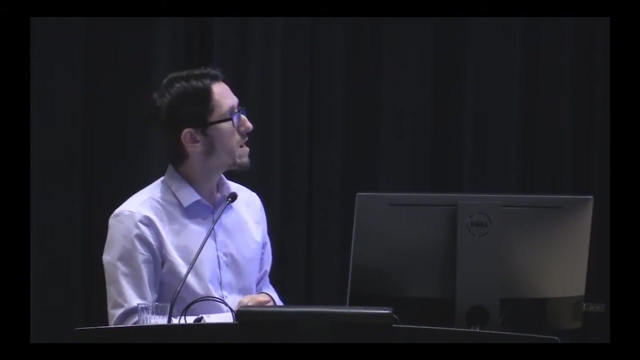 have dominated speech and audio processing, So Google is using this all for your phone to recognize what you're saying, Translation of text from one language to another, Even dealing with time series data if you have accelerometers or other sensors that you may have on a robot. 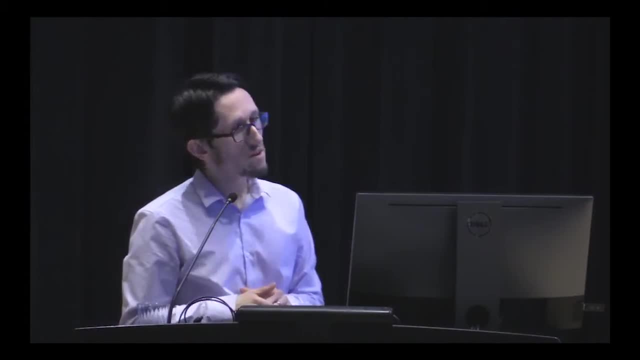 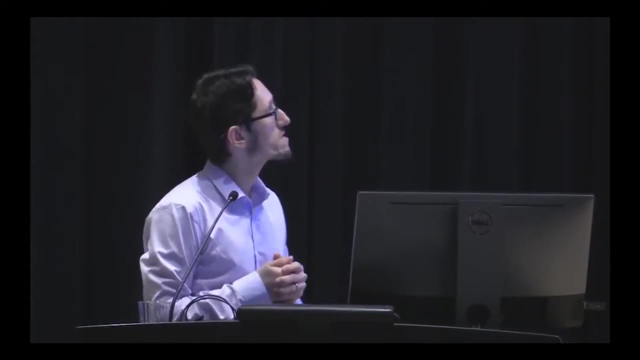 And what's really nice is that they're very complex. They're very complex, They're very computationally light in the sense that we can actually now have them onboard an embedded device which actually we have next door at the petting zoo performing not. 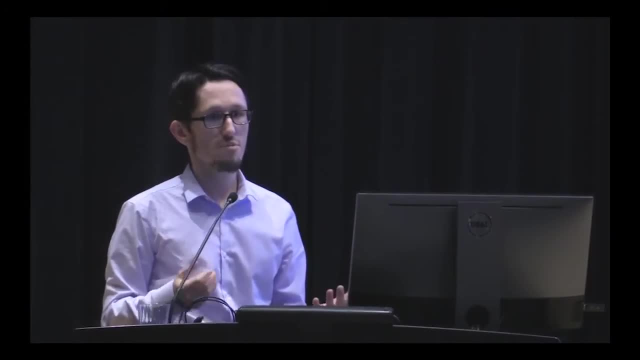 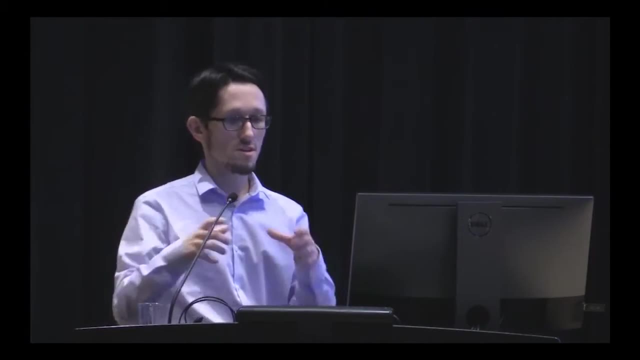 real time at this point, but near about one hertz. for example, object detection across a thousand or more object classes all in one hertz on a really small embedded device that we can actually throw up on a quadrotor or octrotor. 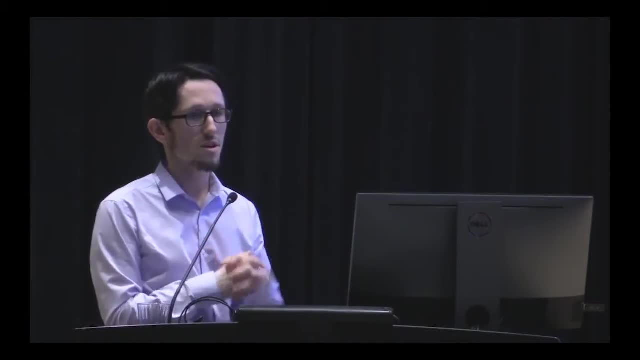 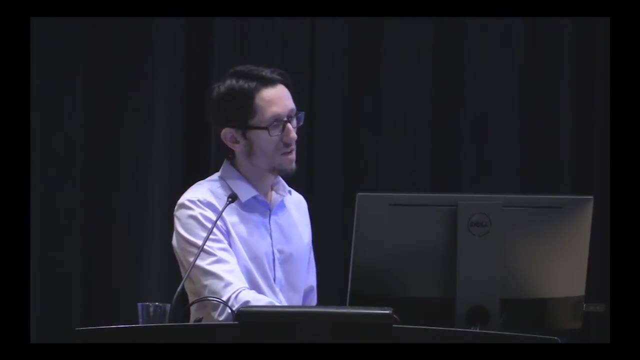 And so that's kind of. one of the advances is that it's not only good across many modalities, it's supercomputational, It's computationally efficient, especially using GPUs that we use, And, again, it also can deal with 3D data as well. 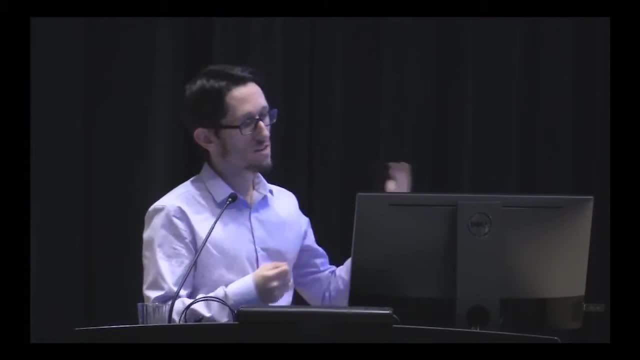 So, basically, all the modalities that you see will be taken over by these methods, if they haven't already. Really, there's still some limitations, which is the amount of data we need, And I'll talk about that later when I talk about the future. 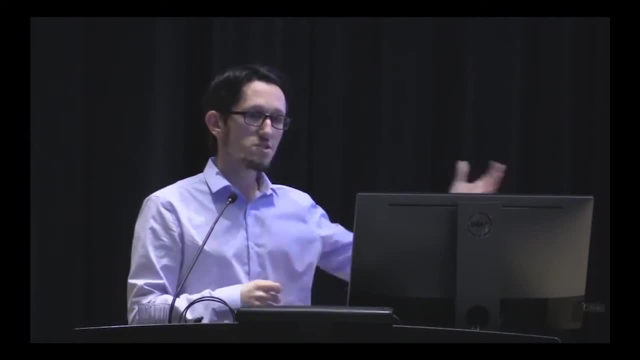 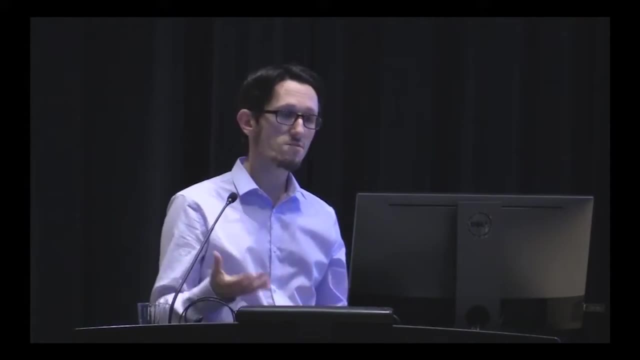 And one other thing is: not only does it deal with individual modalities, It also deals with data. As I showed in that object detection example, where we combined images and LIDAR, you can actually use these methods to automatically optimize for a particular task by combining. 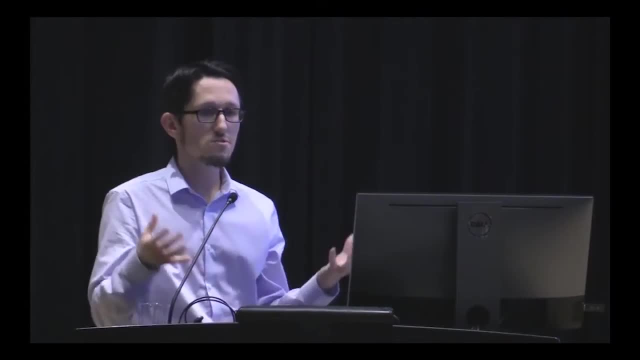 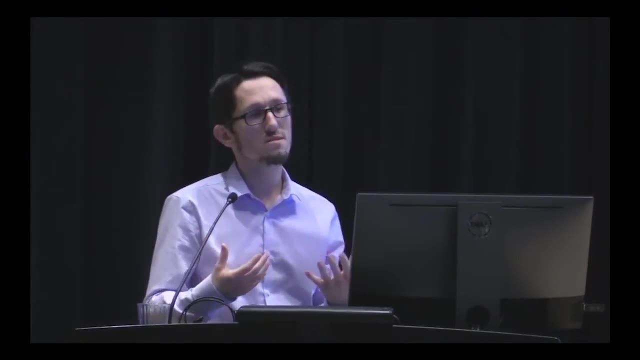 multiple modalities together, So you can transfer, for example, extract semantic information from LIDAR and images and basically relate them and somehow represent the data in a way such that it's parsable both in terms of LIDAR or in terms of images. 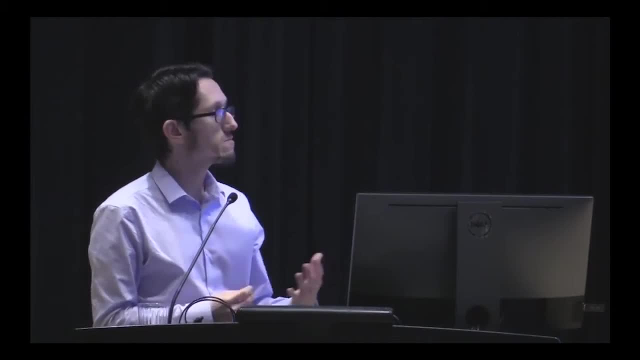 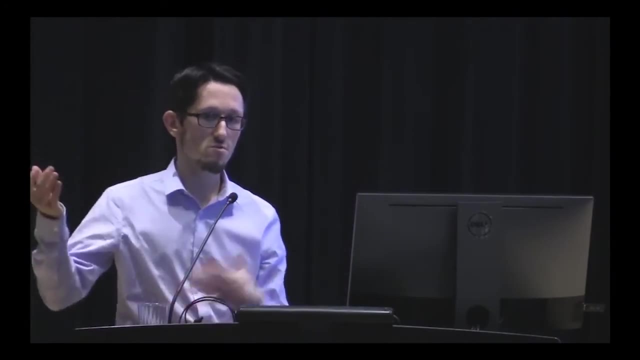 And so this is really a great way to do that. So this is really a really good thing because, for example, you can use text to query images, or you can use images to query audio. So you can go across modalities in terms of what you process and what a person maybe. 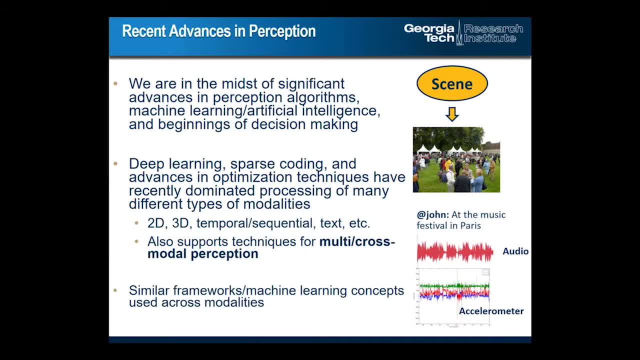 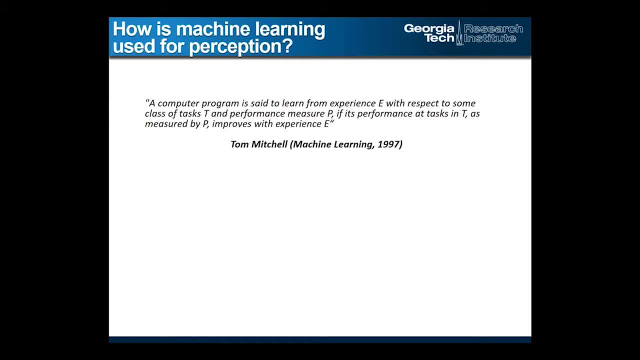 if he or she is looking for something, how that person queries. So I won't go too much into machine learning, but really the key to learning is having some form of experience. In our case it's typically data or sensor data. We have a set of tasks. 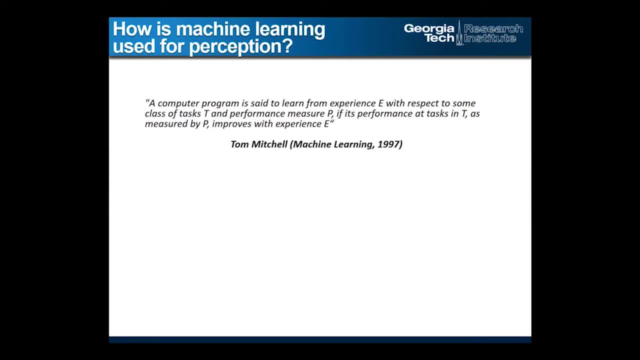 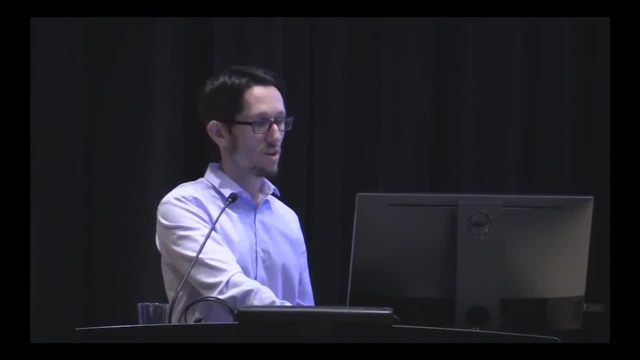 For example, I want to identify all the objects in this image. I have some performance measure of how well I'm doing And then basically I update my machine learning model to do better and better as I get more and more data. And one thing: that's a little bit of a limitation now, but in the past two years people have 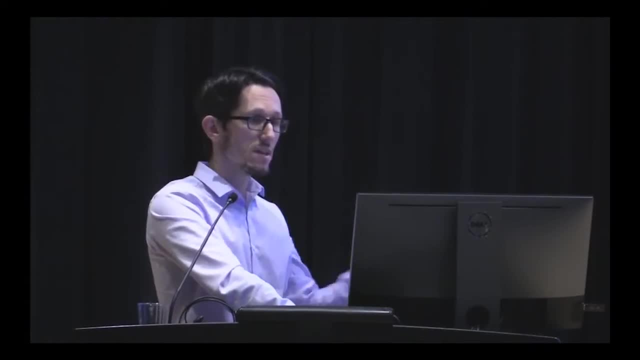 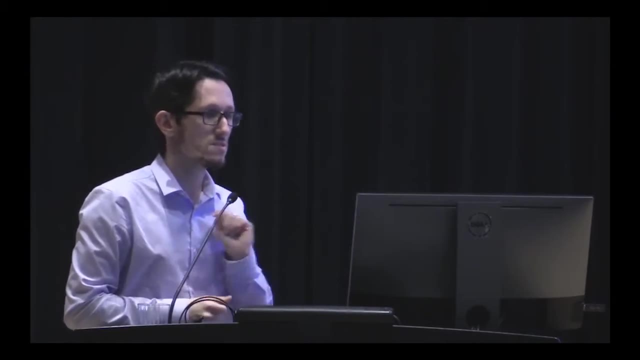 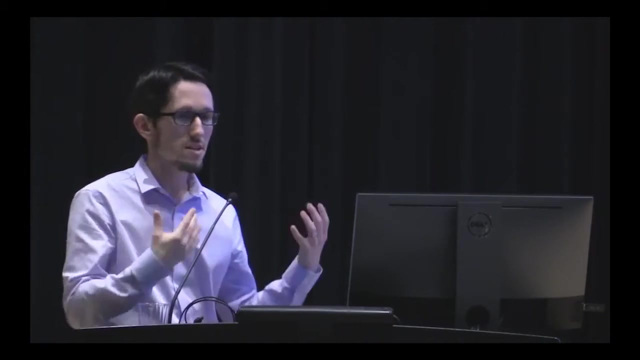 been working on addressing is that we not only need data, but we need label data. We need data such that it's images that have bounding boxes that says this is a person a thousand times. So very tedious data to collect, But people are working on methods that can just literally take unlabeled data and extract. 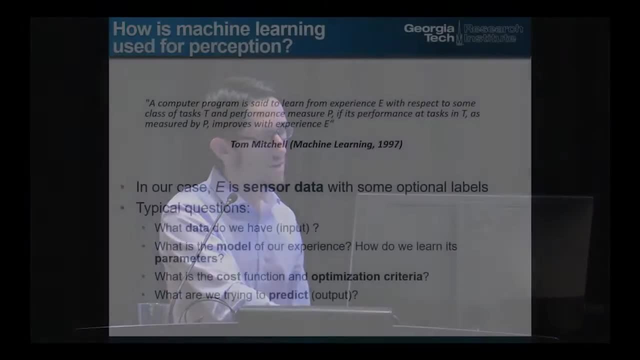 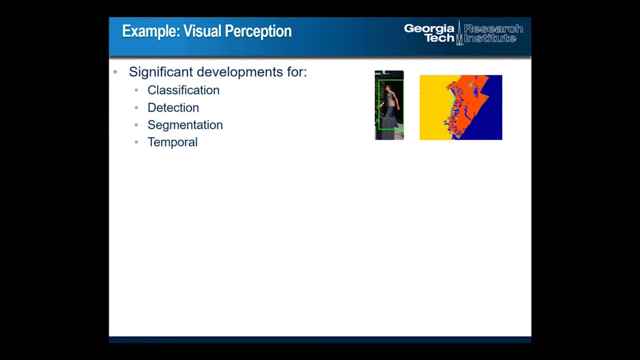 some patterns or meaning from it as well. I'll go through that. So, similar to how it's used across different modalities of data, it's also used across for different tasks. So the task can be literally just put a bounding box on a person or the task can be for each. 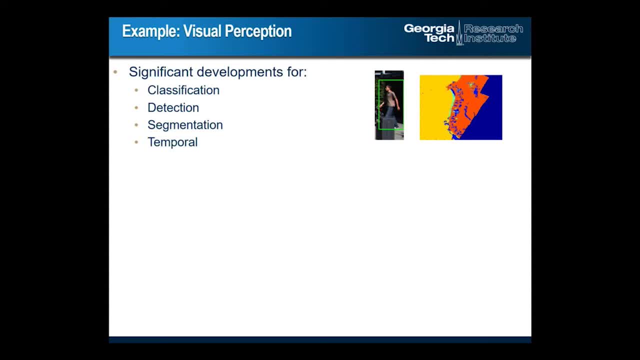 pixel give me what that object is. Okay, And these methods are equally applicable to those two tasks. They're also applicable to temporal data, all those kinds of things, different things. I can show one example. okay, You've seen in one of the videos with the object detection, but we can also do segmentation. 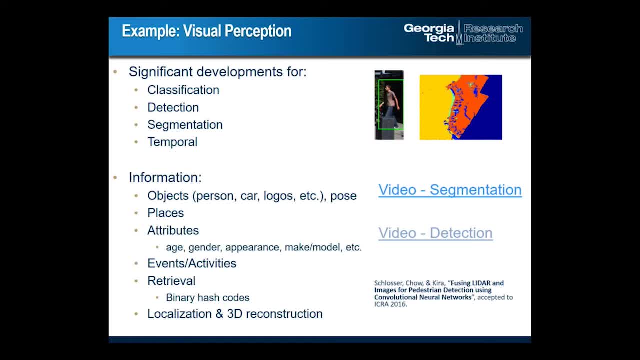 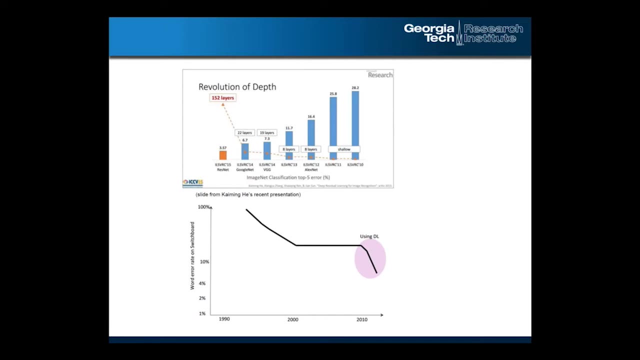 as well. And in the video we also show, for example, age and gender classification. So, given a person that you've detected, can you estimate attributes about that person or make a model of a car and so on. And really there is a lot of hype in the media about AI and machine learning. there's 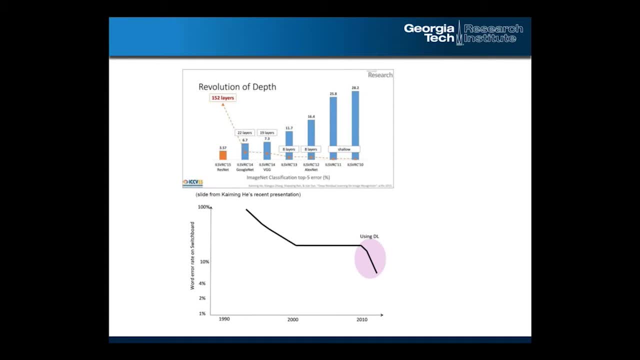 no question. However, we have made significant quantitative gains in the accuracy of these things. So, on the top, it shows basically the error rates from about 2010,. before deep learning or neural networks came back into rage. Okay, So where we had 28%, and this is actually top five error where you only have to get 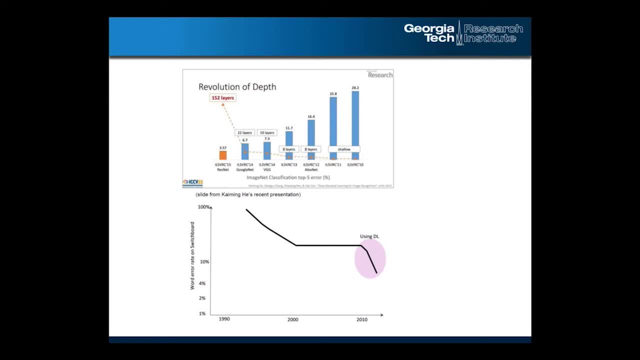 it within the top five guesses. so 30% error, which is pretty high, all the way down to less than 3%, which is actually a little bit human level. Of course, it's a hard task for humans because there's a thousand different object categories. 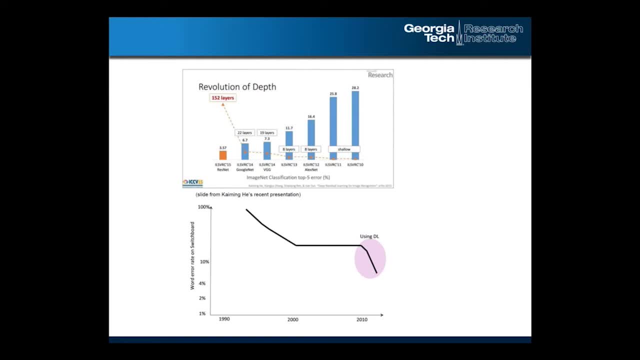 And similar for audio for a long time, since 2000,. we were kind of plateaued. our machine learning methods plateaued- Okay. So that's a lot of hype in the media about 2010,, 2012,- that deep learning has made significant. 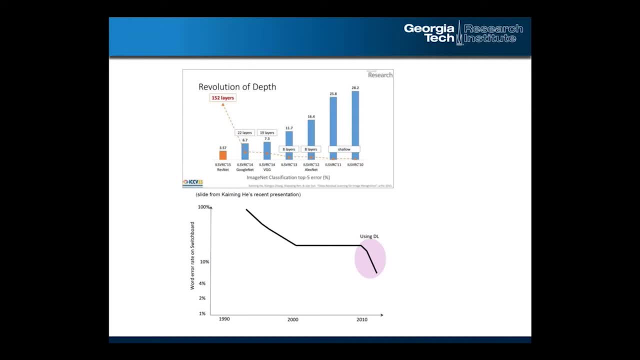 contributions. So while there is a lot of hype, there's also a lot of quantitative improvements that have been made in the past five years And again these quantitative improvements make it so that we can actually use it, for example, to be a human player in Go. 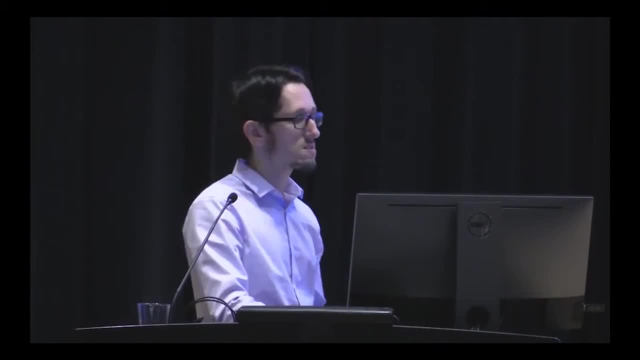 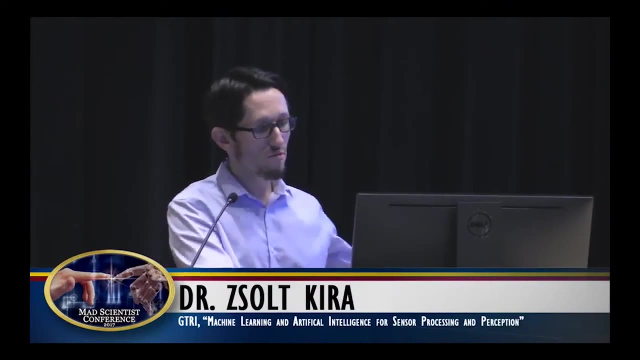 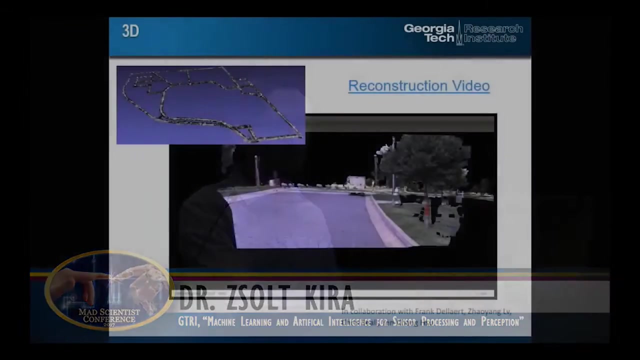 So it's still not perfect by any means. it's still not as good as a human for more complicated tasks or multiple tasks at once, But very useful for doing actual things in the real world. This I showed already, but we can do also 3D processing. 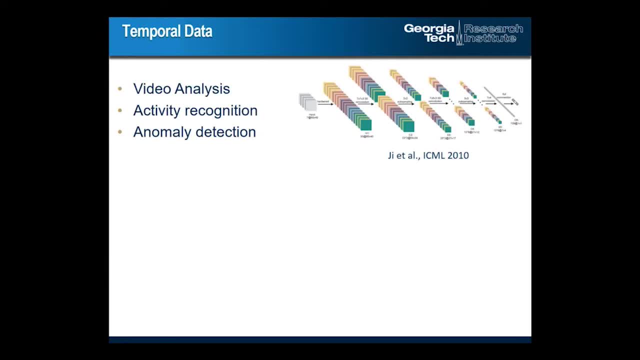 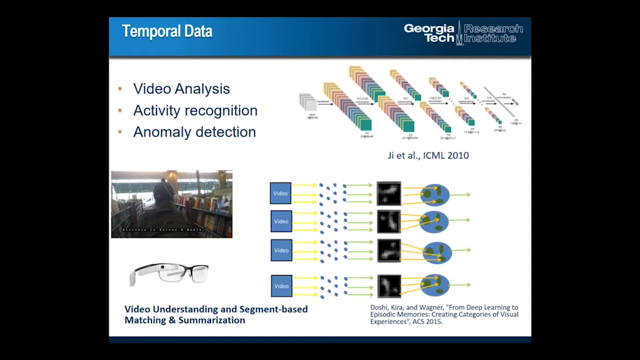 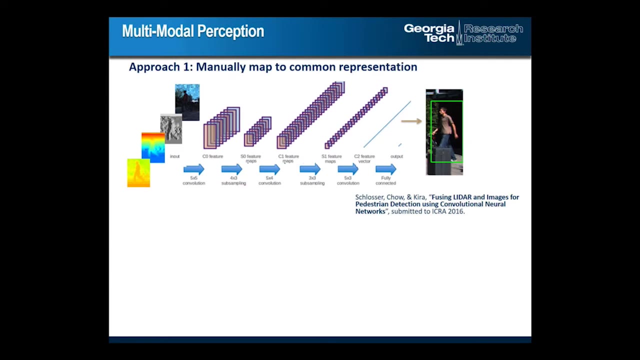 This shows kind of audio processing that we can do as well, And I'll go through these quickly just to highlight some of the things We can do: video analysis: activity recognition, anomaly detection, all those different things from video understanding. We can do multimodal perception, where you're combining not just the images up here but 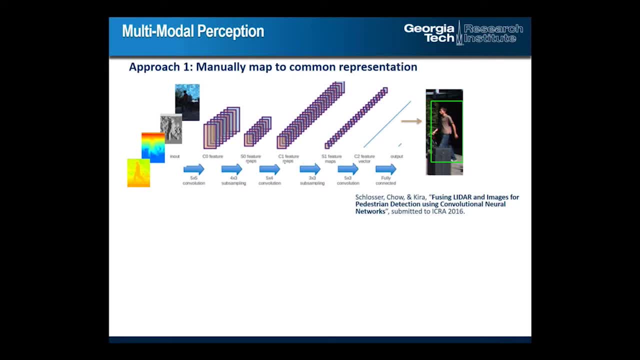 you're actually combining 3D information as well. And again the key is: it's literally all data driven. You just give it the same inputs and outputs, except you add a modality. So we added 3D information here. We still gave it the same box that just says the person. 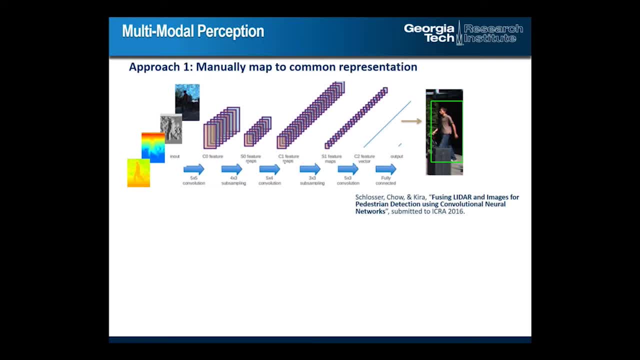 And literally, we don't do any modification to the machine learning or features that it's extracting. In the past, people have spent decades and decades of PhD time to literally say: I want to detect a person, I want to detect an image. 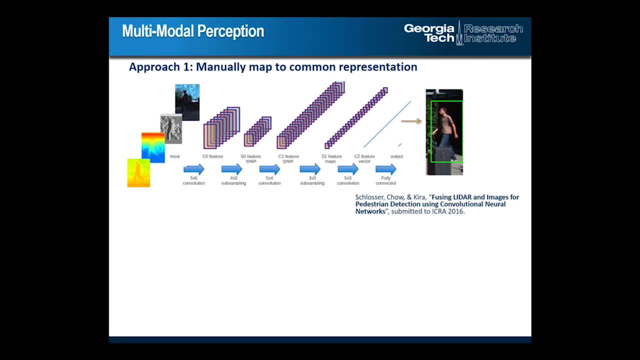 What features are good for that? I want to detect a person in stereo. What features are good for that? I want to detect more, different objects. What features are good for that? So, literally, that feature engineering approach has been replaced with. just give it some data. 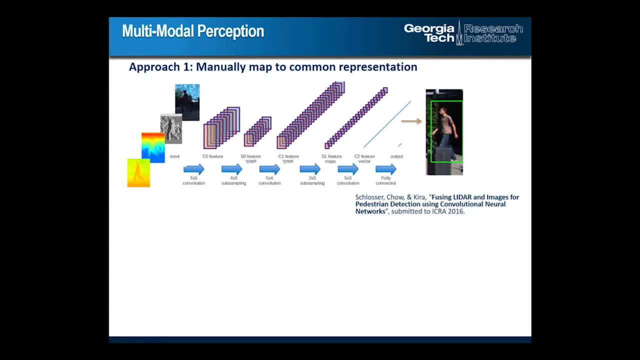 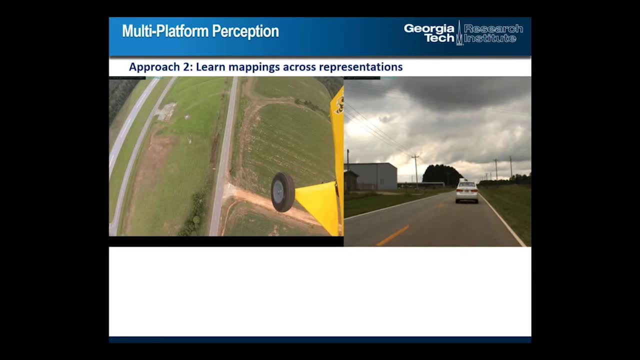 raw data. give it some labels at the end and it automatically learns what features are good for detecting those kinds of things. Also, you can map representations not just across different images, Again, modalities or sensors on one platform, but maybe across multiple platforms. 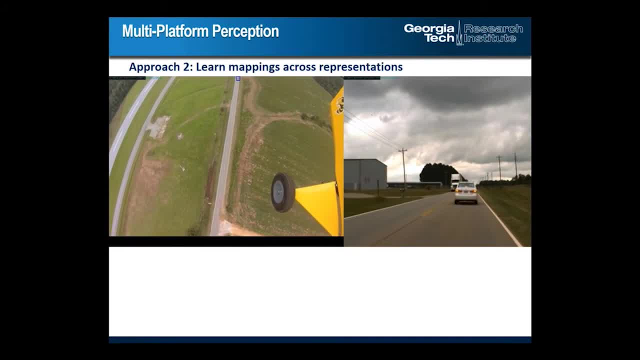 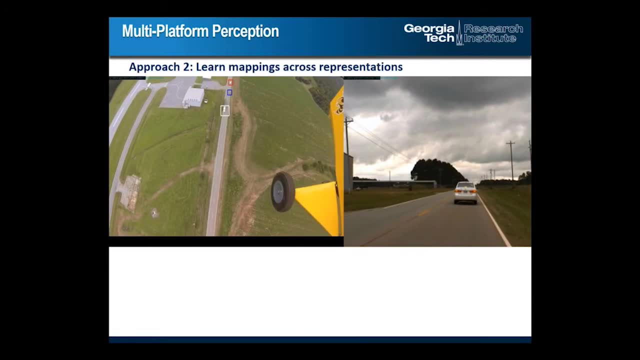 So this shows an example of detecting and building a machine learning model of the appearance of a particular target car in the white box, or actually in the blue box from the aerial vehicle, And then how can you transfer that machine learning model to a ground vehicle. 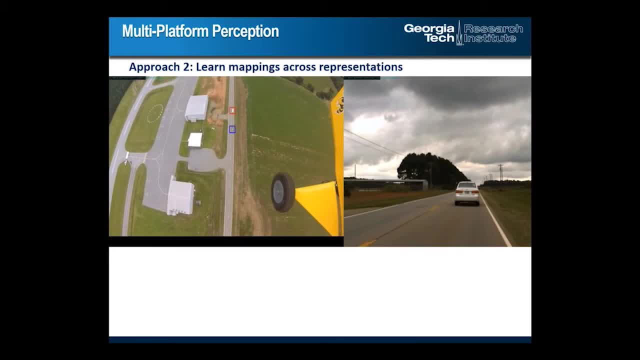 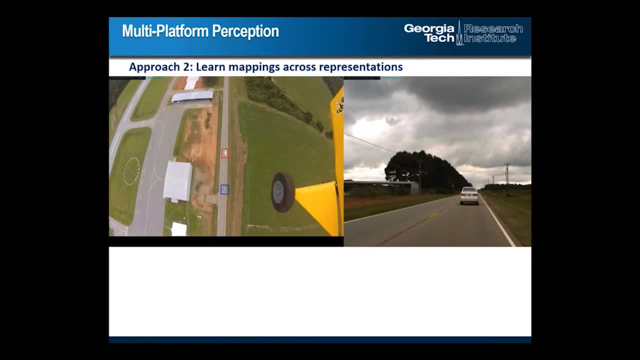 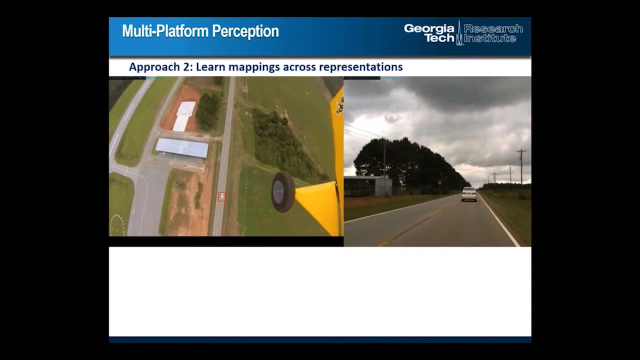 So this aspect that everybody's been alluding to so far, which is manned, unmanned teams, where you just have Not just aerial or ground, You have lots of different domains. We do have some work in how to transfer information across. We're not transferring raw sensor data because you're never going to have the bandwidth to. 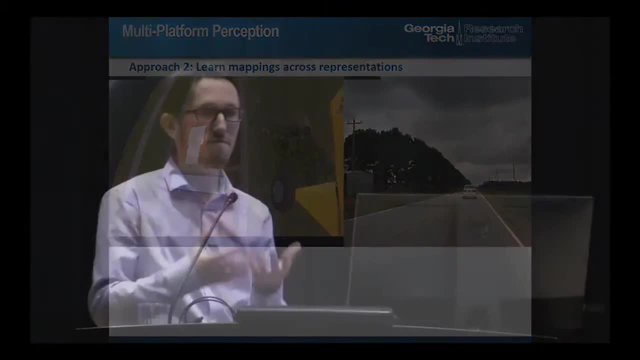 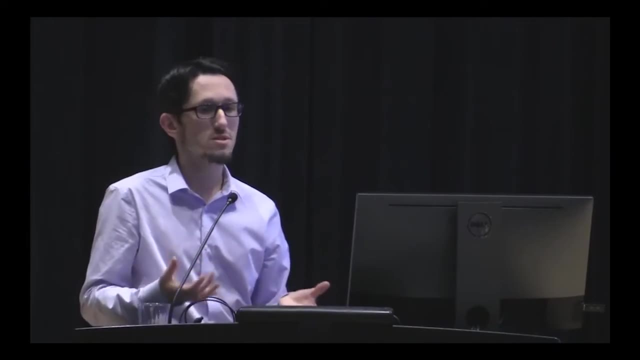 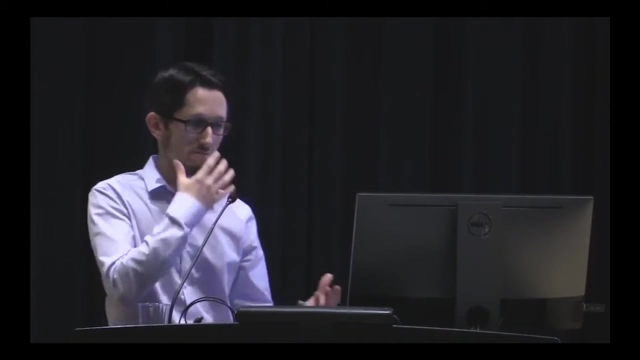 do that. What you want to do is do some onboard extraction of information from your raw sensor data into some semantically meaningful representations and then basically transmit that to other platforms as well. Of course, there's a lot of research questions of how you actually integrate all that information. 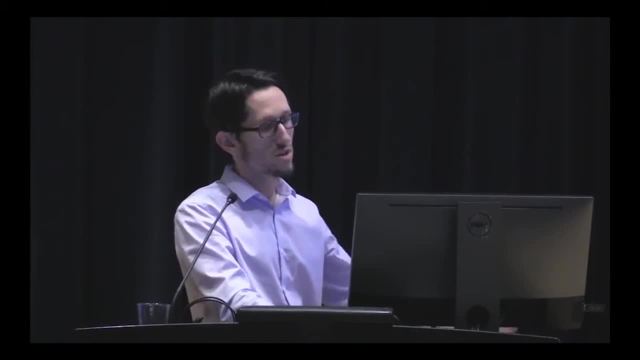 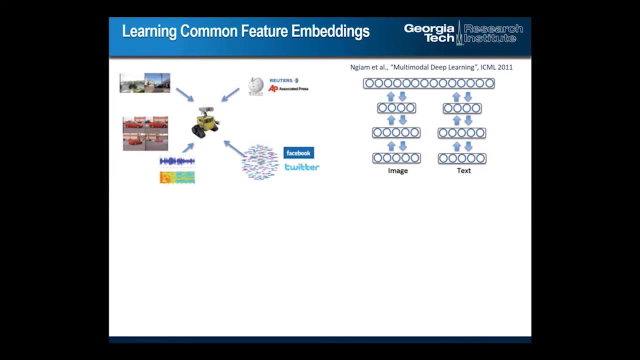 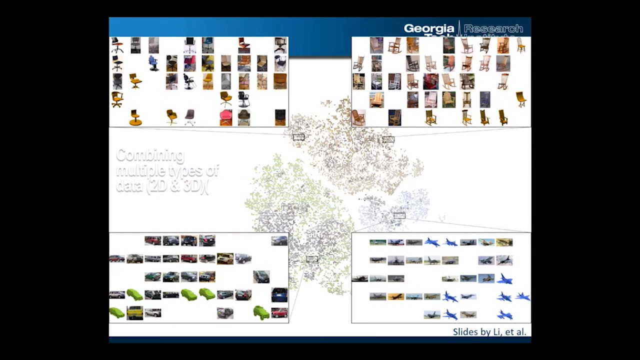 and so on, But there are methods and people are working on it, including us. There's also, again, this notion of learning feature representations that are geared across lots of different modalities, And I'll show you a cool example here where you literally can. 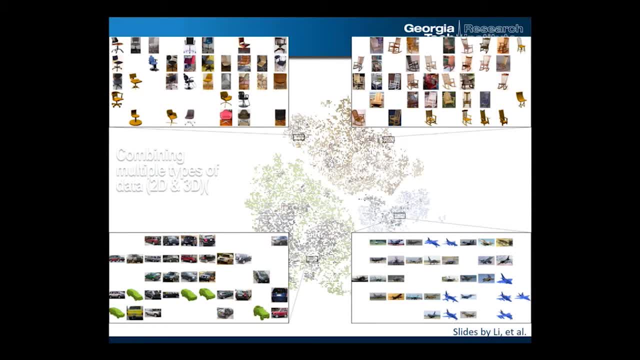 So each point here either represents an image or a 3D model. so an image of an airplane or a 3D model of an airplane. And what's cool is You can learn, using machine learning, feature representations such that a point in the space 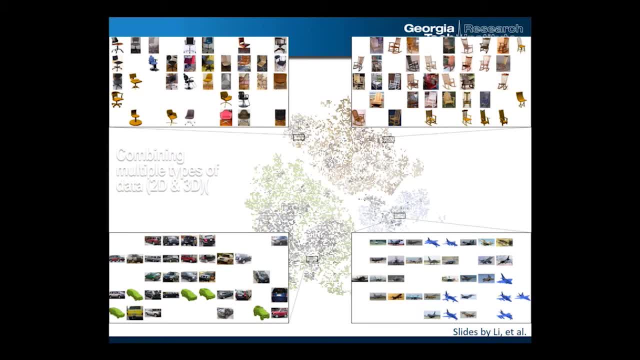 for example, for an image of an airplane is very close to the 3D model of an airplane. So what's cool is you can do queries So you can give it an image, or these days you can even literally just sketch stuff. 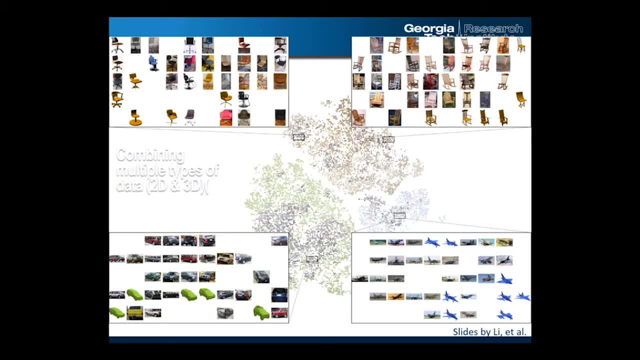 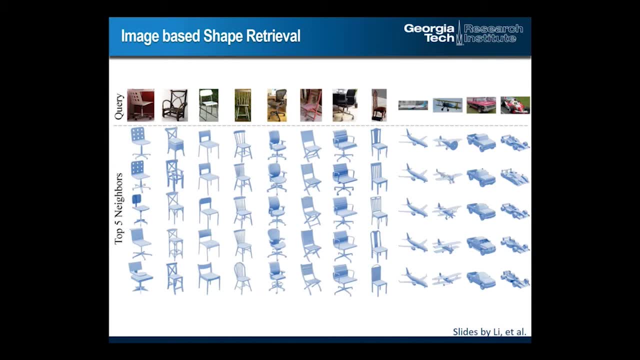 Do an outline sketch and it automatically queries this large database of information to give you back what you queried for. So very cool stuff. Again, this is using these kinds of objects, but obviously you can use your imagination. It's applicable to pretty much any target or object that you may want to use it for. 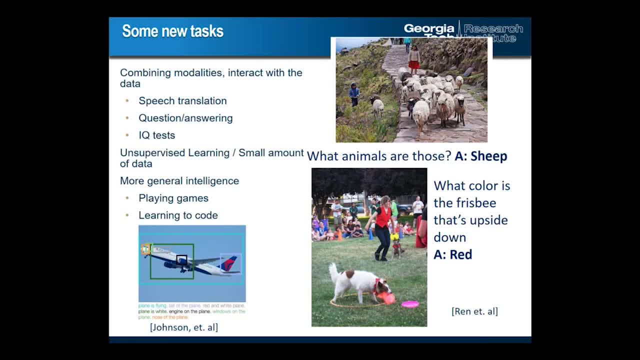 Some really interesting things that are coming out is not just fixed tasks like querying or detecting objects, but can you interact with your data, Can you talk to your data and ask it questions? So there's a field now of visual question answering. actually, Georgia Tech just hired. 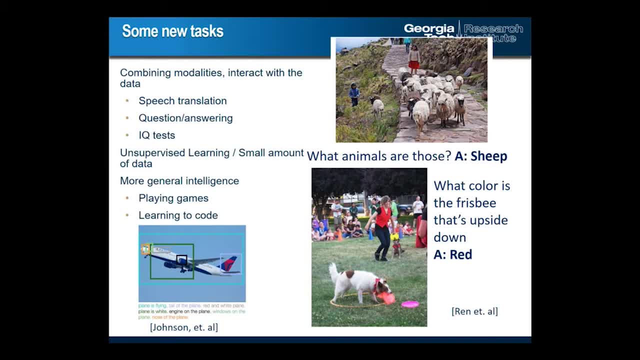 someone in that area, A faculty member, A faculty in that area, So you can literally take an image. it could say what animals are those and the AI gives you back sheet Or down there it says what color is the Frisbee? that's upside down. 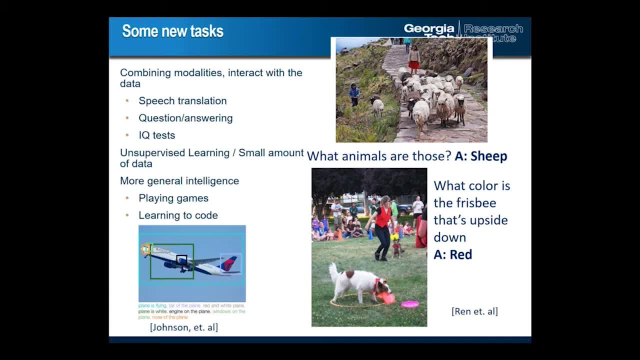 Here it says red and notice it's actually incorrect. so it's not perfect. I do want to emphasize: none of these methods are perfect. None of these methods- especially the more complicated tasks like visual question answering humans- are better, But we've made significant, significant advances in getting these systems to actually do this. 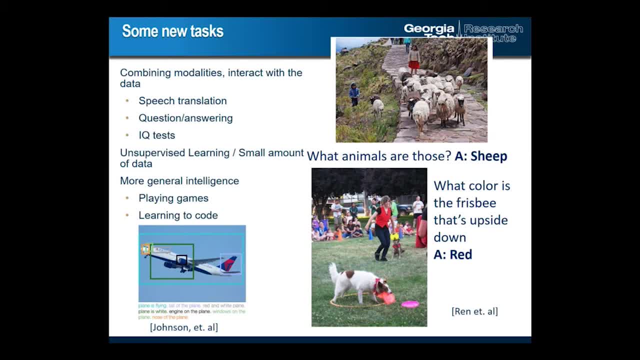 And then also again generating textual data. So, literally, you have an image of an airplane, lots of different parts of the airplane, and it can generate text saying the plane is flying. the tail of the plane is here, it's a red. 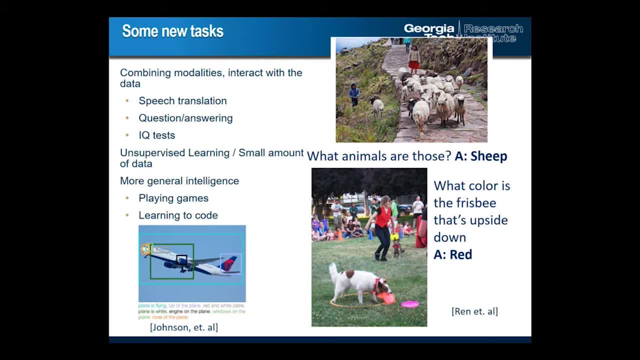 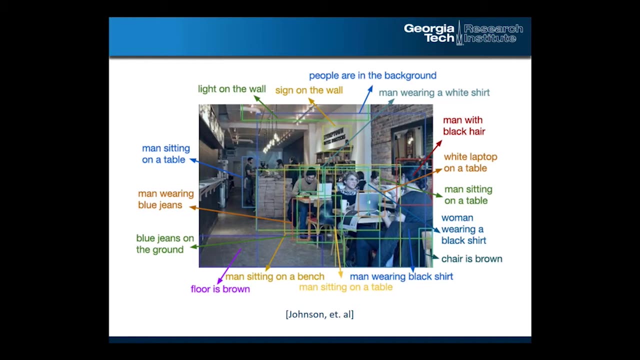 and white plane. the engine is on the plane, the window is on the plane right there, So it can really tell you fine grained information about your data, not just that it's an object. This shows another example. You have a very complex scene and you have a whole set of different descriptions. 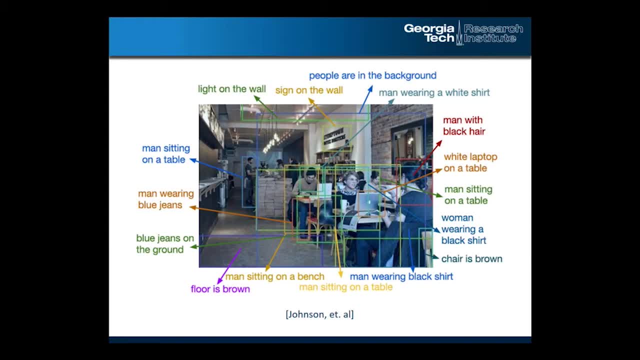 And again, this is not my work, this is work from Stanford- but very complex descriptions of images and what is in those images. And again, I show a lot of images because that's what my field is a lot of. but you can use your imagination to do these kinds of things across audio, across hyperspectral. 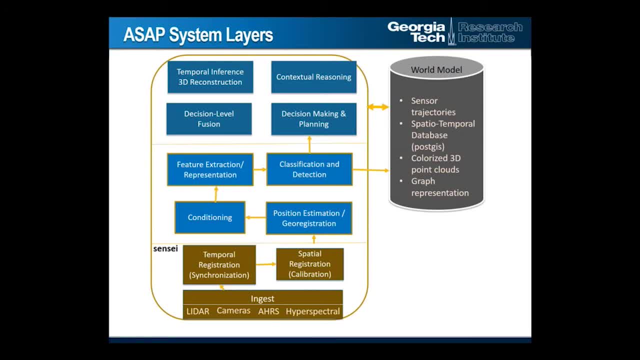 across SAR, which we are looking at as well. I'm going to show one example that kind of integrates this. So, with respect to robotics, now we can take all those pieces of information that we're collecting using machine learning and put it together to actually perform some kind. 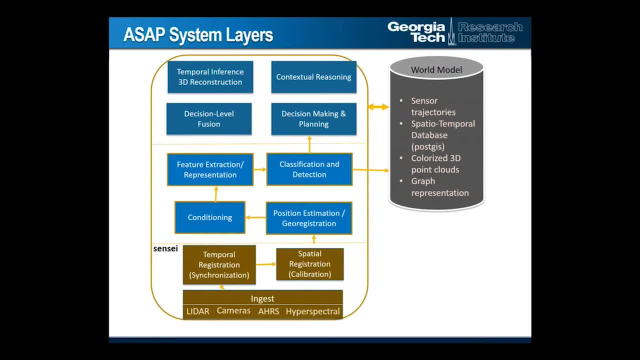 of task, And so we're really moving up the entire chain where we're ingesting raw sensor data of multiple modalities, We're synchronizing them and registering them spatially, We can estimate their position, we can extract features, we can classify everything and detect. 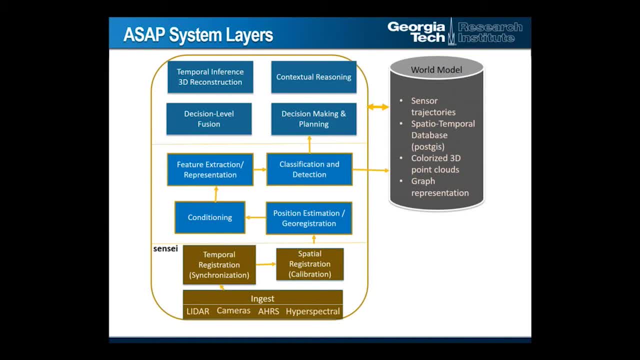 and track objects And then, at the higher level, we can start making actual decisions for them. And then, at the higher level, we can start making actual decisions for them. And then, at the higher level, we can start making actual decisions for them. 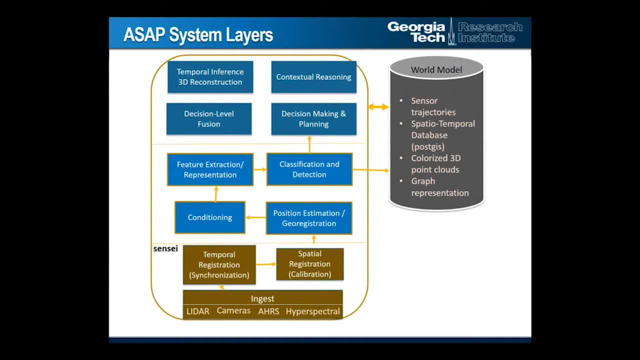 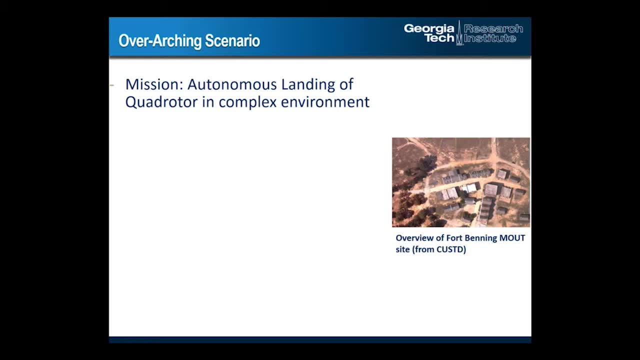 We can start making actual decisions for them After that, for example in a mission for a quadrotor. And the particular mission that we're actually looking at is some kind of, let's say, you have some kind of compound that's actually Fort Benning where we do a lot of robotics. 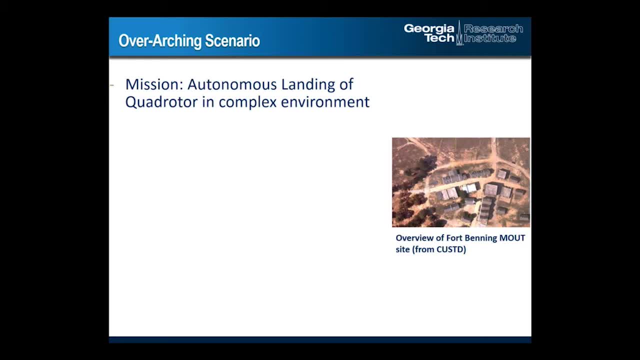 tests where you can understand the scene, look at everything that's in it, all the static and dynamic objects in it, And then you can essentially extract those pieces of information over time, For example, estimating temporal patterns of where people tend to be. we actually extract. 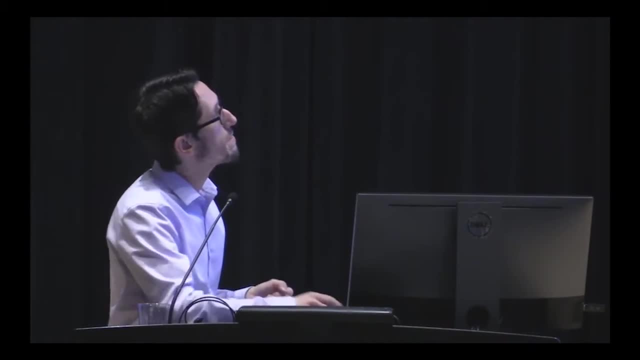 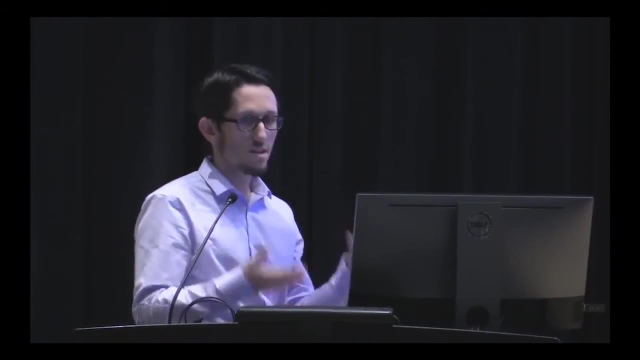 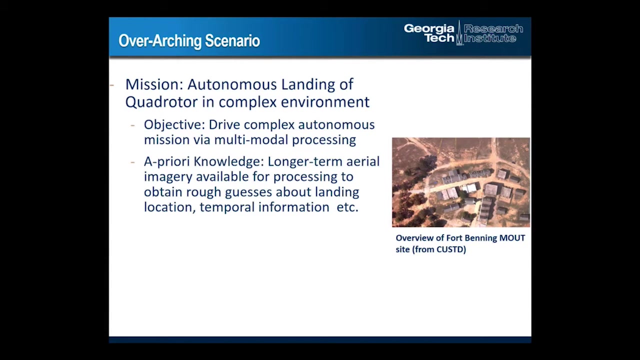 maps of where activity tends to be in this place and then we can use that to actually drive a mission. and we actually have two modes, kind of what we call a mother-daughter scenario, where we gather a priori information. so some of the sensors. obviously we can't put on small UAVs at this point, so for example, we 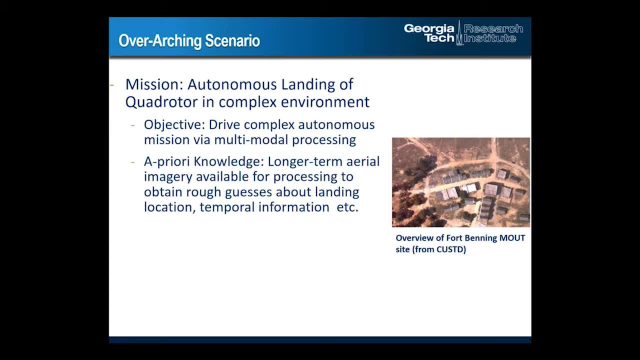 have a very sophisticated light, our sensor. we have hyper spectral, long wave, shortwave, mid wave, IR. all those sensors- not all of them- can be on a UAV. so what we do is essentially have an overhead kind of monitoring of the scene, understand what is going on in the environment, and then we use that to 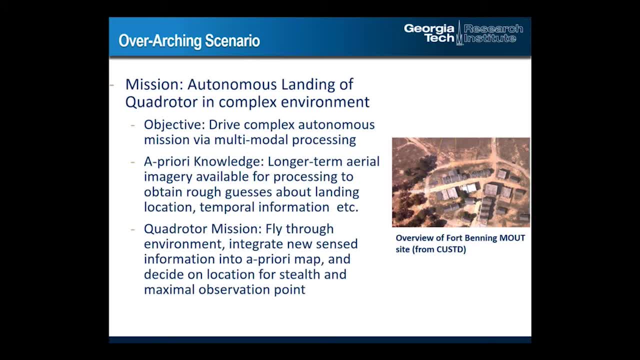 drive a robotic mission. but what's cool is the robot also has its own sensors, maybe less sophisticated, maybe somebody showed the velodyne lidar, which gives you 3d information. there's actually one that's actually next door. you can see it, you know. it's $8,000. 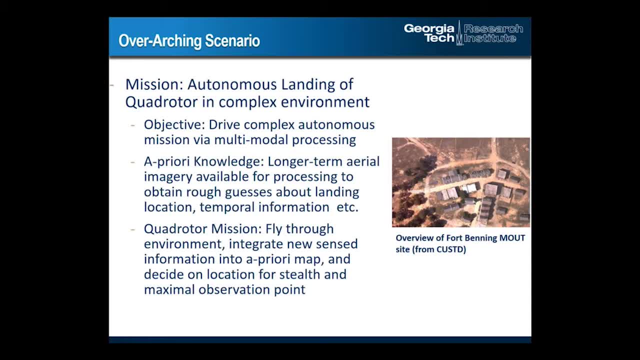 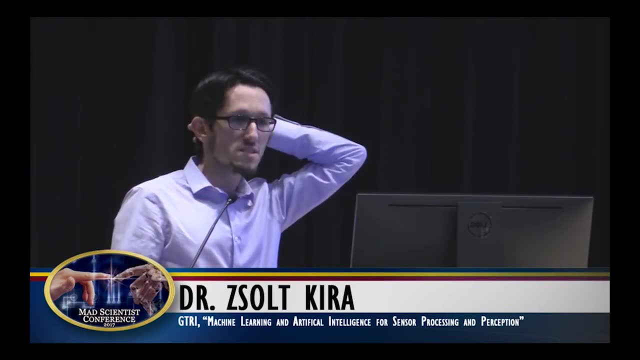 and gives you 16 layers of planes of 3d information, lidar, and you know you can extract, you can do all sorts of different things like obstacle avoidance, object detection and so on, and so the actual robotic system can take the plans that were generated using the more sophisticated sensors and then update. 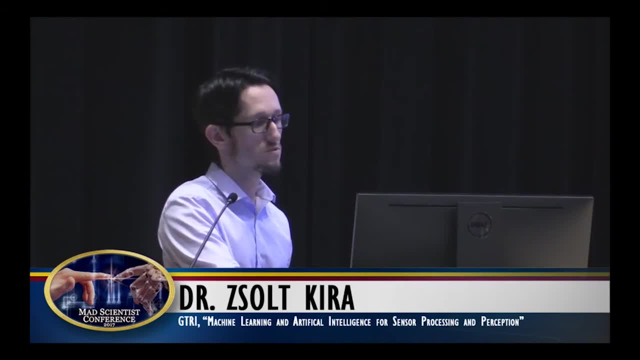 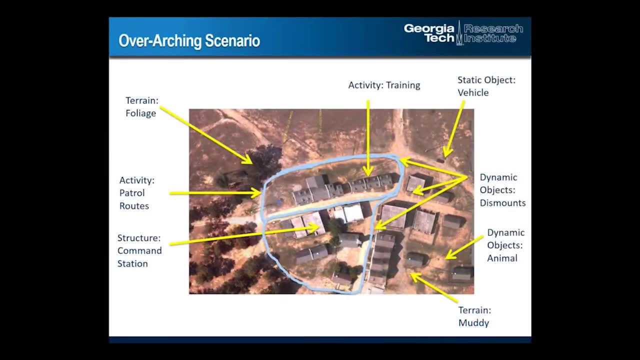 the plan depending on what it actually sees in the field. so this shows some examples of things you might want to actually detect: terrain type where our landing zones, for example. so we're doing some landing zone automated landing zone determination activities, patrol routes and so on. so we actually did a cool data. 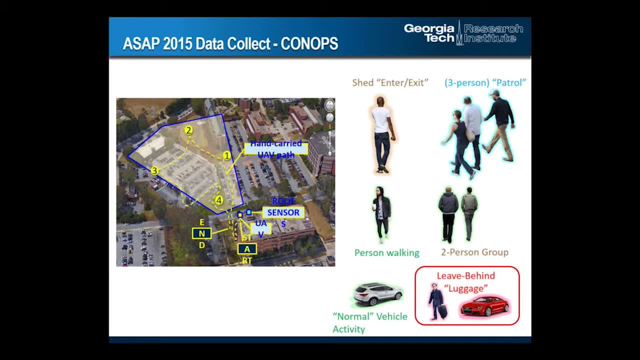 collect that or detect. so one of the limitations of doing multimodal research is that there's not a lot of data sets for individual modalities. for some of these there's about zero data sets that I can get access to anyway. for multimodal large collects- where you're, you know how the different sensors are. 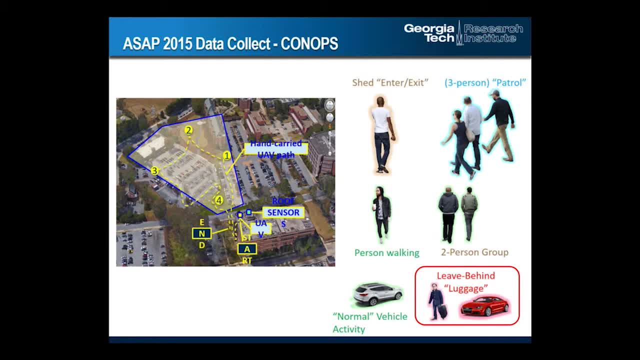 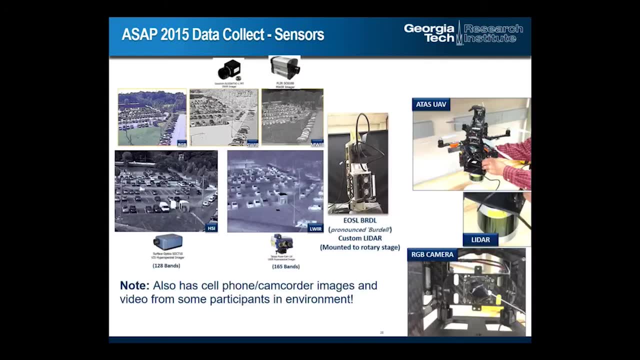 registered and where they- um, you know what it does- like I think they're actually are in space and time such that you can actually register them to extract more information. so we collected our own and drew detect from a rooftop. actually, for the more sophisticated sensors and these, this shows some of the different sensors. 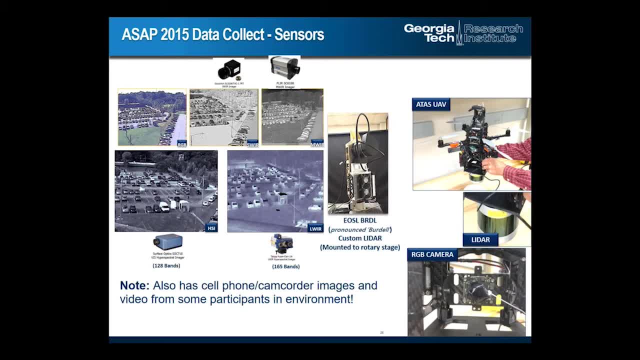 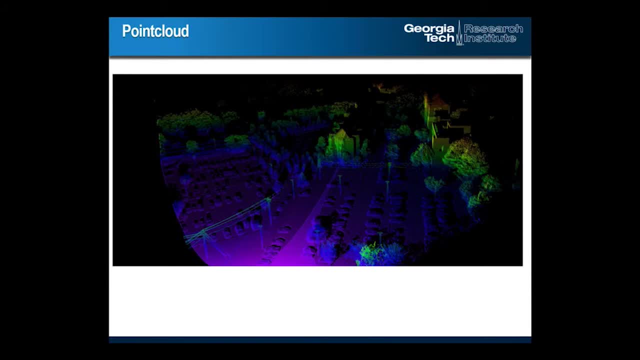 that. and then we also had sensors. this shows the velodyne. that little puck on the right is the velodyne lidar, very small and you can actually put on a UAV. this shows the point cloud that we generated from 3d information from the 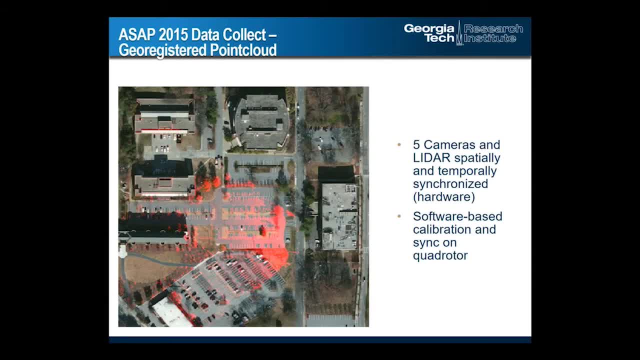 lidar. this shows the imagery registered on the point cloud. you can project it onto ortho photos to make sure. so really, what's cool is you can extract a whole lot of different information- and I'll show some other examples- and then generate a mission for a quadrotor, for example, and then have that quadrotor use. 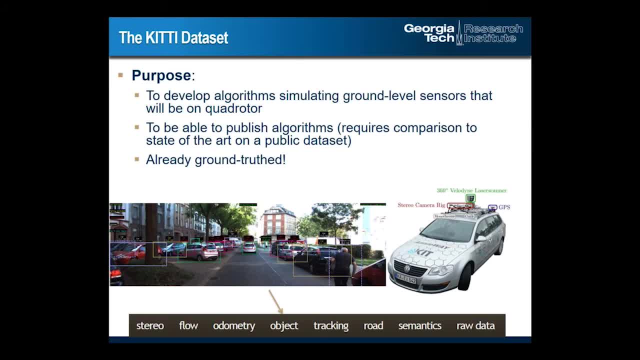 its local sensing to update that mission. so one of the examples again that I already showed is this object detected from the quadrotors perspective. now we have Nappa at the Earth kind of data. this is using public data so we can publish papers, but we're also 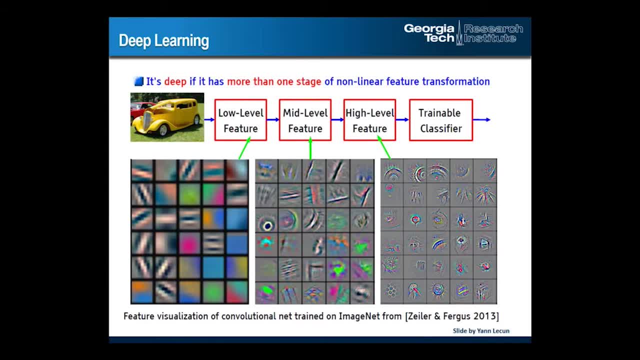 putting it on the actual vehicle. and again, the key innovation here is deep learning, where we- this may not mean a lot to you, but it's actually learning these features, so we initialize features randomly and then it's actually learning what to detect, what patterns to detect in your data, such that it can finally 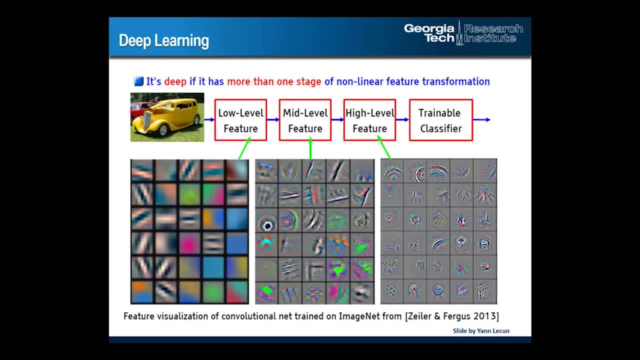 tell you what is the object in there. and actually at the low level it's typically these kind of edges or lines that you see, and actually similar patterns have been observed in the v1 system of the brain and then, kind of after that, it gets more of shapes and 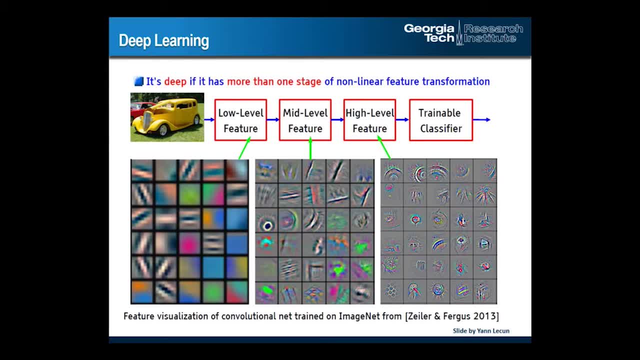 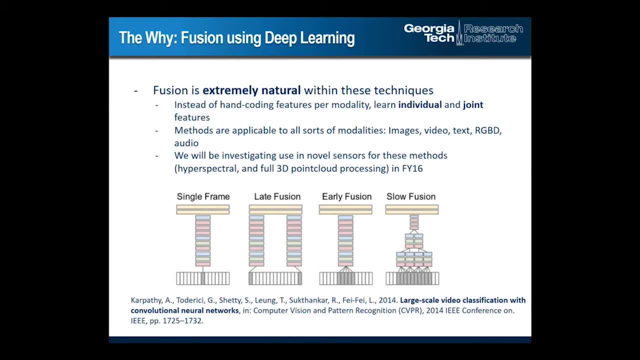 object, parts and entire objects, and again, all that is just learned from data. all I give it is lots of data and then labels at the end, and what's cool about that is, since you're learning everything, all the features. there's a question of what features should you learn from one modality versus the other, and when? 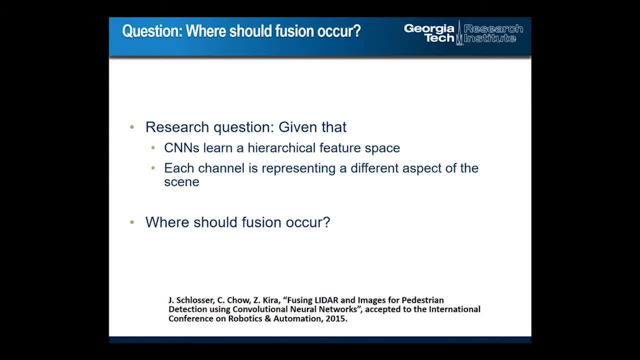 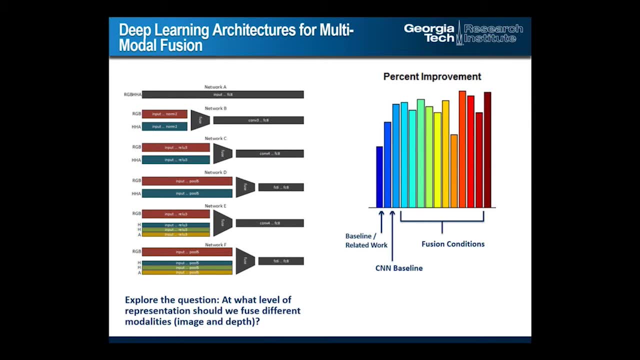 should you actually fuse it together? so that's actually a really good question what we explored and we have different fusion architecture. so basically, these lines on the left you can see our processing images. on the bottom it's kind of for the same architecture. it's processing LiDAR 3d information and we 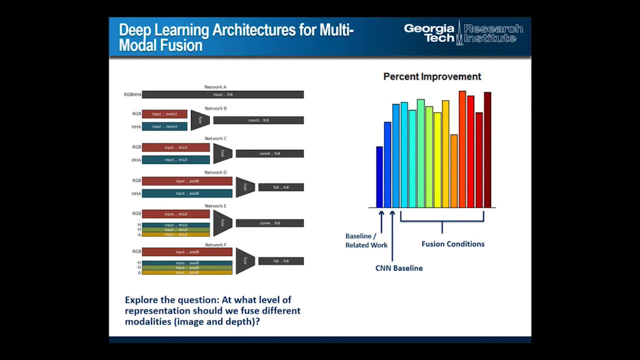 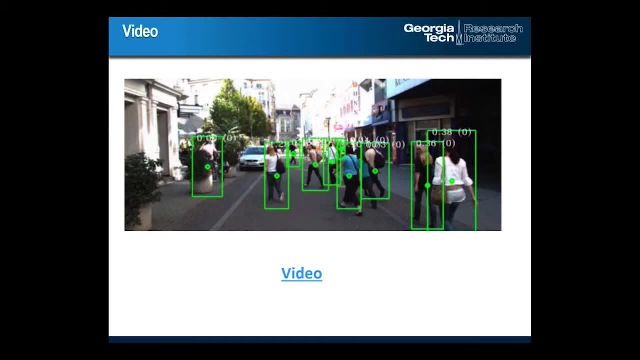 can fuse it at different points. we can fuse it in the beginning, we can fuse it in the middle, we can fuse it at the end, and it turns out actually if you get in the middle gets you the best performance, and that was what resulted in that video. 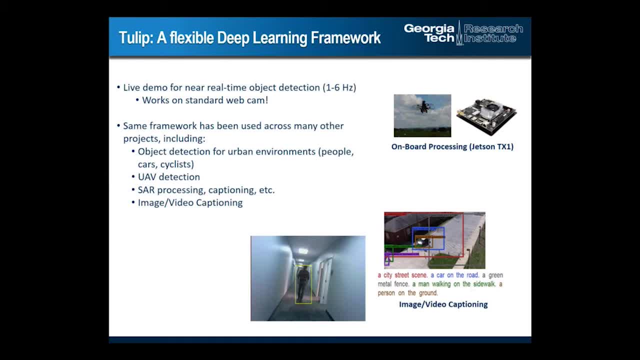 that I showed and we have our own kind of architecture. that what's again? what's nice about this is that we have a lot of information and we have a lot of data. so what's nice, is it? the same techniques are for multiple types of data, so we use the same techniques for detecting things in SAR detecting UAVs. 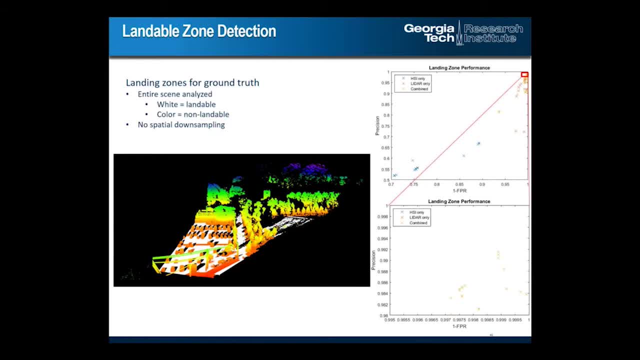 and so on. we thought we've also done high perceptual classification, landing zone determination- this is the ground truth, landing zones. and then we have precision and recall curves and we are doing really well at determining which parts are landable in this 3d data for a quad rotor. and then actually we're going. 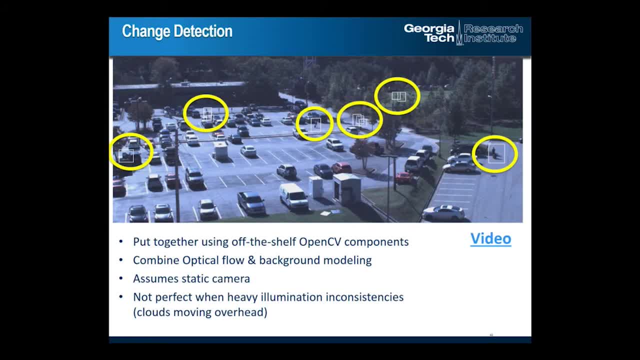 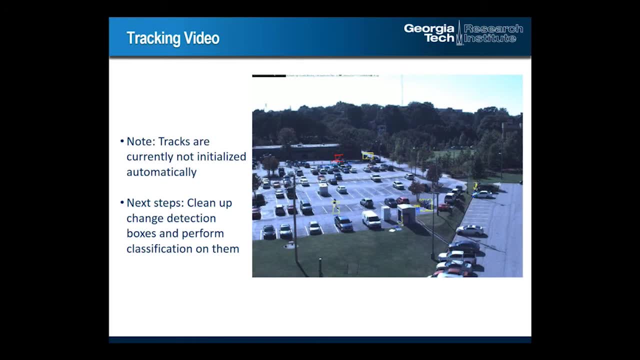 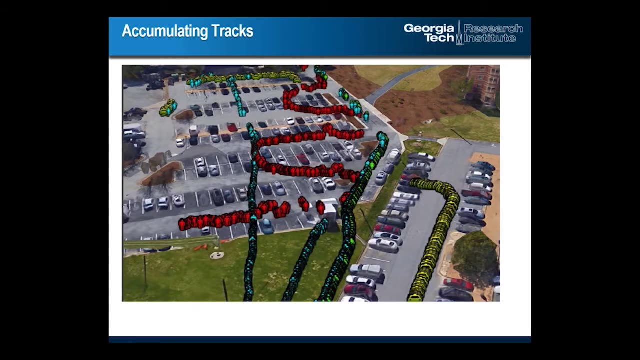 to validate that using a physics engine at some point as well. we've done change the scene, we've done tracking- so I don't know why this movie is super sped up- but basically tracking all different objects across our entire data set automatically, and then we're generating these 3d tracks because we have lidar data. we 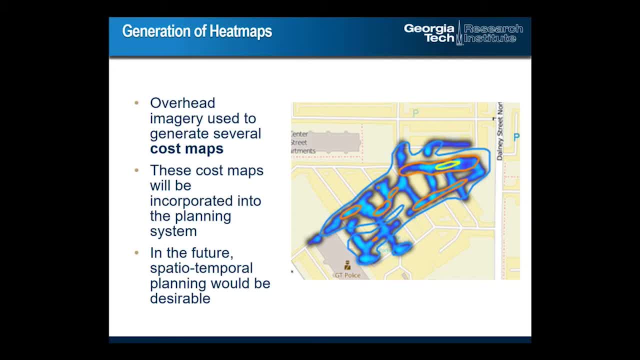 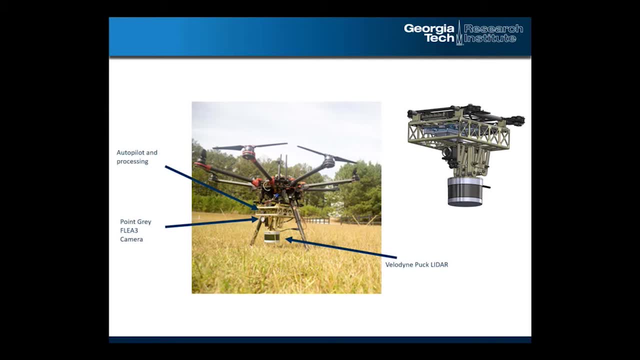 know where, exactly where these tracks are, and then we can generate heat map. so where is their activity in this kind of environment? and this is the actual off-roader that's next door that you can see that we're planning to fly this mission sometime this year or early next year, and this is some images of it. 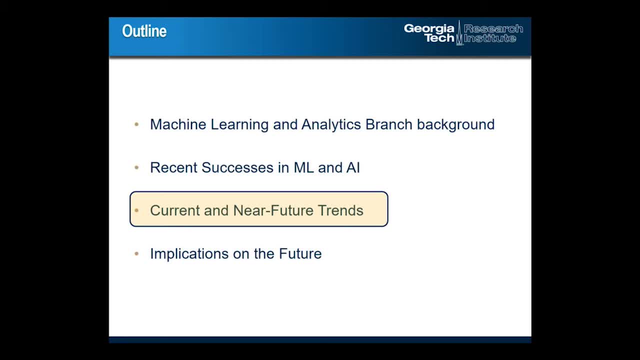 falling. so basically, that's kind of just to give you a very fast, very firehose like idea of lots and lots of progress has been made just in the past five years for processing all sorts of modalities of data. there's a lot of interesting things that have only come out in the past year or two. one is 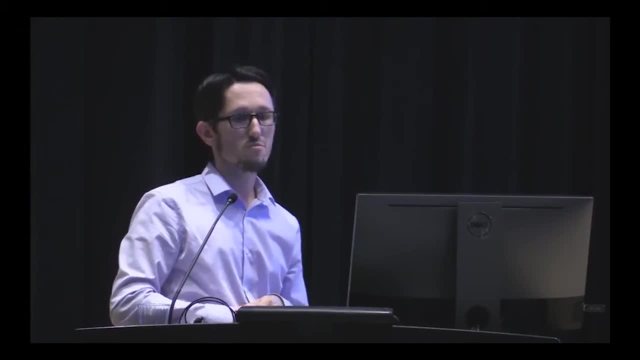 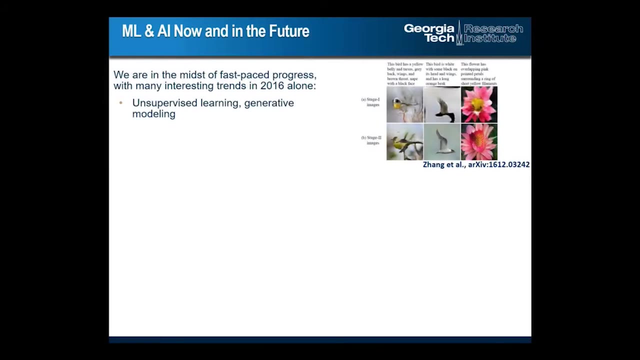 what's called unsupervised learning, which again I referred to the problem that somebody mentioned this as well in the DoD you don't have, you know the web where you can just crawl a million images and have four students label them. all you have is literally SAR data, maybe a little bit of it. you have hyperspectral data, maybe a. 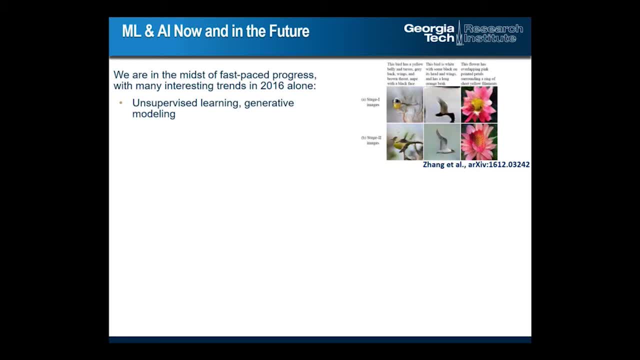 little bit more than SAR, and then maybe some labels, but not a lot, definitely not in the thousands or tens of thousands, definitely not in the millions. and so there's a whole trend of how can we learn from just data itself without somebody actually telling us what is in that data? there's this new class of 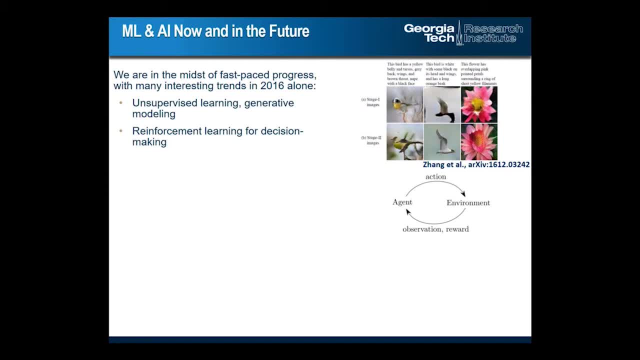 machine learning called reinforcement learning, and that's literally learning from reward, so you can process your sensory data, understand what's in the environment. and then you do some action and somebody tells you that action was bad or good and how bad or good that was, and based on that you actually update. 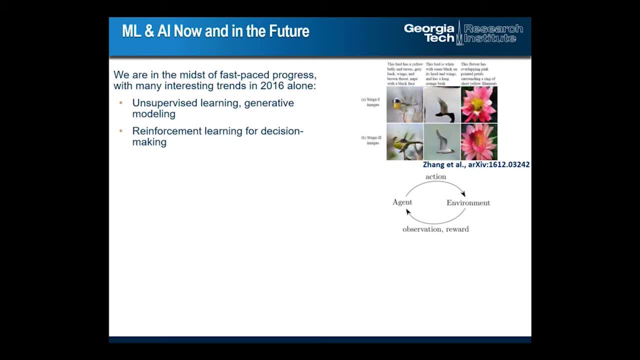 your decision making of how to actually perform that action. there's multitask, so. So one thing that all the hype doesn't show you is that even when it's kind of superhuman where we can detect a thousand objects better than a person, it's really just one task. 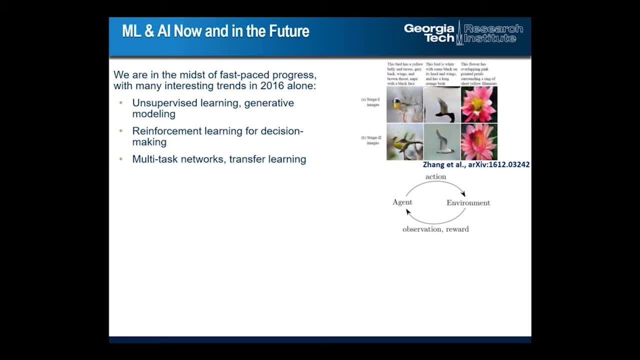 Literally, we take machine learning, we take lots of data and we train it for about six days on GPUs and it does really really well on that one task. Humans are obviously much better at lots of different things. right, You can take the same person. you can have that person do all sorts of different things. 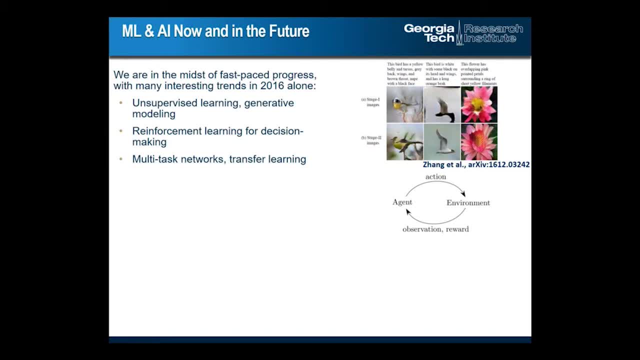 at the same time, involving perception, involving action, decision-making, all sorts of different things. We're not at a state by any means for AI and machine learning, So people are starting to look at how do you, for example, learn how to navigate through? 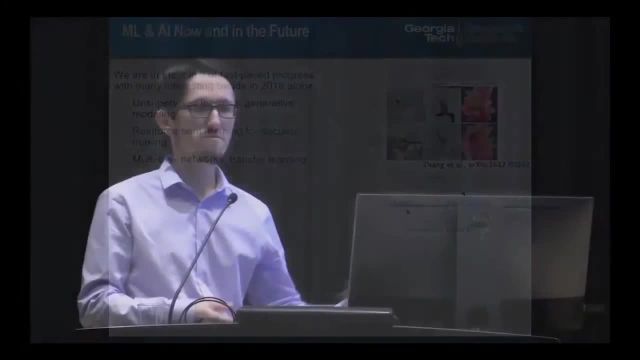 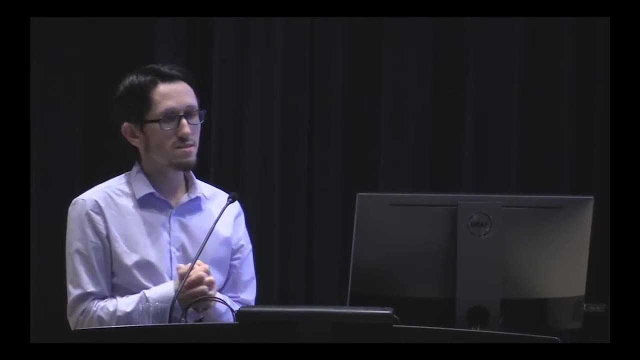 a hallway for a quadrotor. and, given what you've learned, transfer that to a different kind of task, Maybe following someone. So there's lots of different kind of cross-task transfer and obviously humans have a lot of stuff in their brain such that, given a new task, if you give me a new game, I never 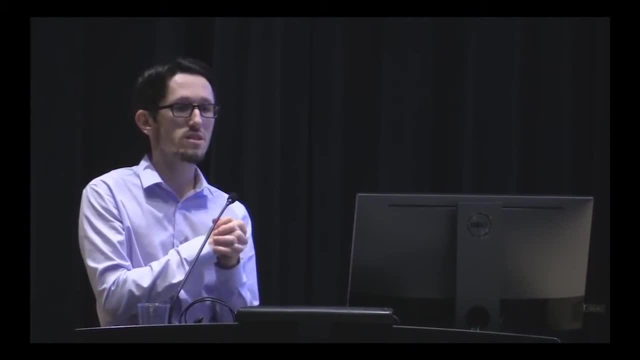 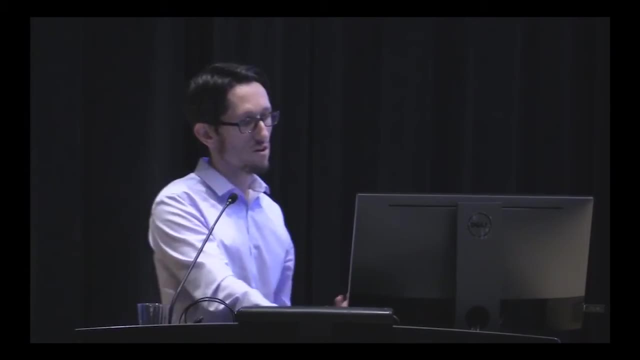 played Go. so if you show me Go, I can learn that task really quickly because I have a lot of knowledge and a lot of stuff that I've learned beforehand. So people are thinking about that- not very far along, but starting to think about that. 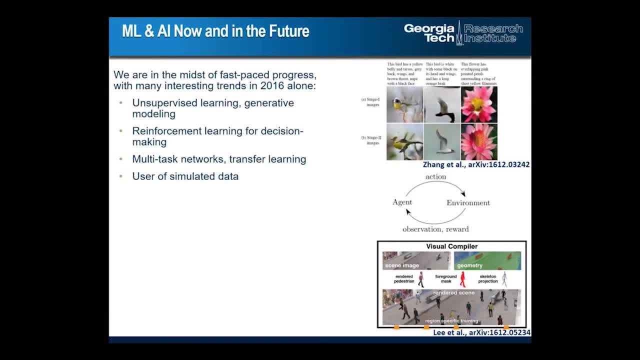 One interesting thing that you can also do that has come up In the past year or two, is we can use synthetic data to train these systems. So again, in some cases we may not have data such as SAR, however we know, we understand. 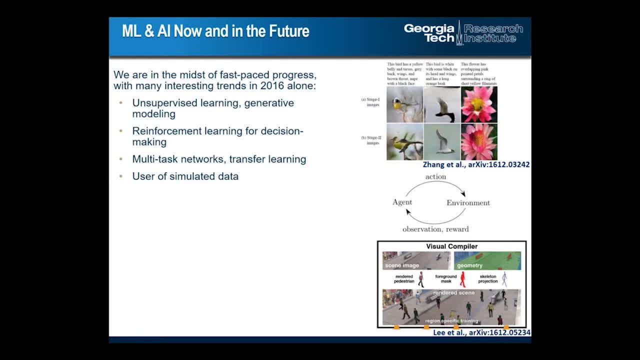 some physics for SAR, We can generate some simulated data. Of course, often the processing time for that is heavy, but that's okay. And then basically we can train our machine learning on that simulated data and synthetic data And it turns out for some tasks you can actually literally train it on synthetic data and throw. 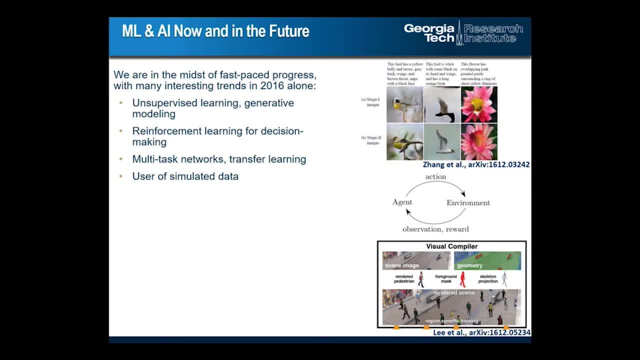 it into the real world and it does really well. A lot of that is dependent, of course, on how good your simulation is. So, for things like rendering of images, the game industry has done a lot of work for us in rendering 3D scenes really, really accurately and involving all sorts of complex lighting. 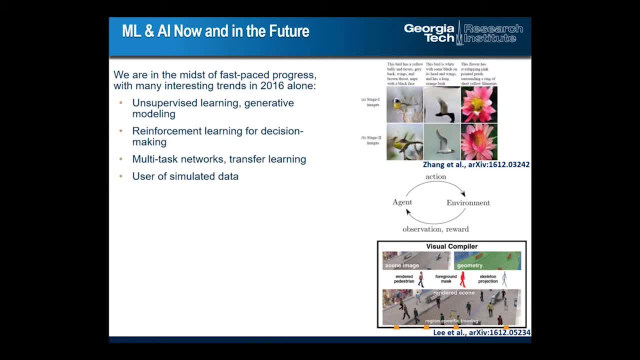 effects, water trees, all sorts of different things. So, thanks to all those graphics people, we can now take those renderings And actually train our machine learning on them, And really that's kind of these things that the machine learning and AI community is working. 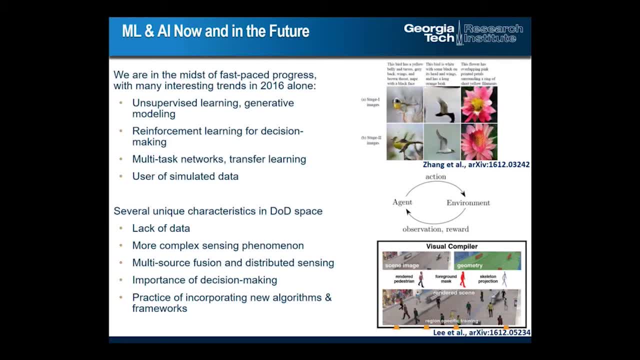 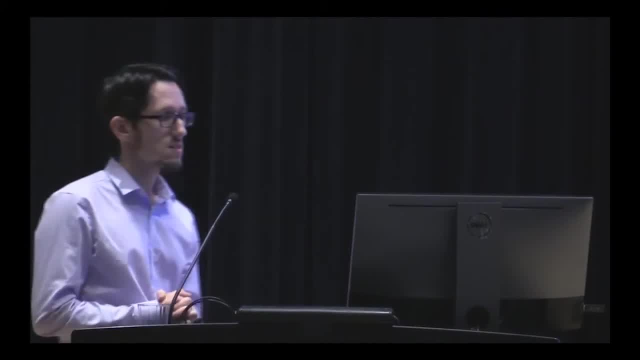 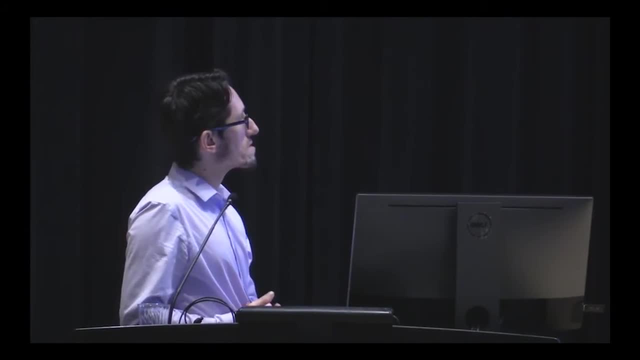 on right now, in the past year or two, is very well mapped to the problems in the DoD, as I mentioned: Lack of data. more complex sensing phenomenon, such as SAR or hyperspectral multi-source fusion and distributed sensing. the importance of decision making. 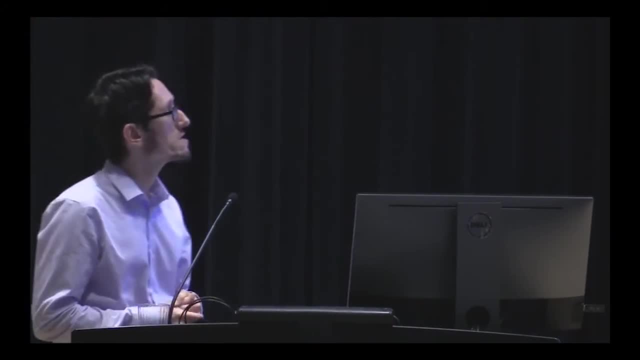 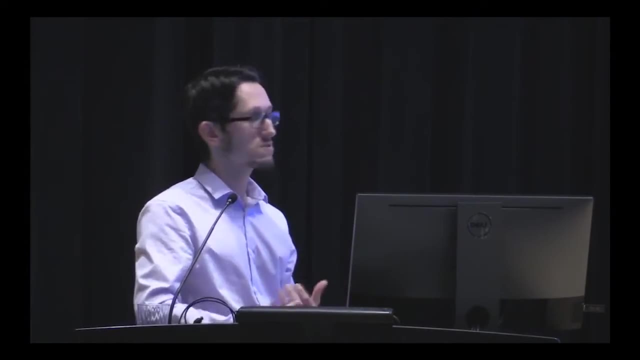 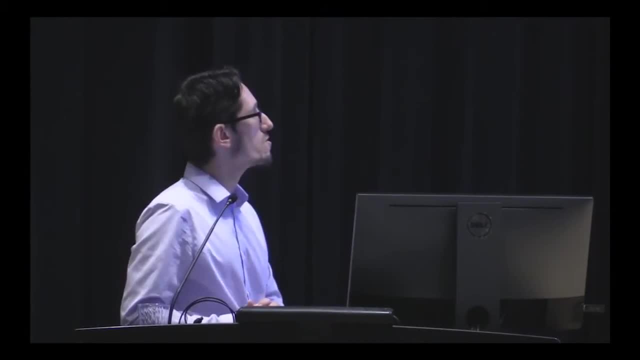 they're still going to be flooded by gigabytes of metadata, So really what we want to do is support them in making decisions and even maybe make some of the more mundane decisions that they have to do on a day-to-day basis. There's also lots of issues of bureaucracy and other things of how do we actually incorporate 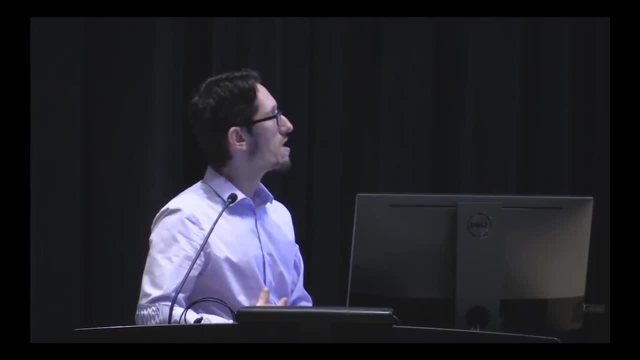 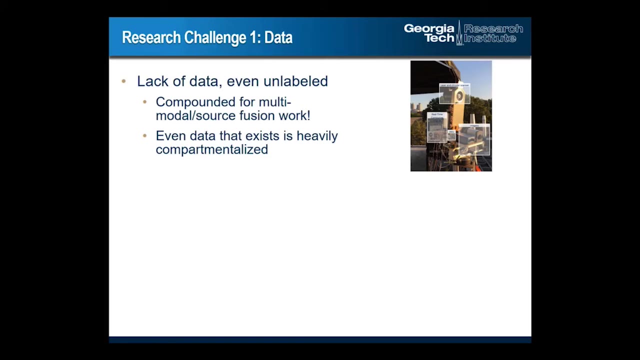 these algorithms, These algorithms and frameworks into real world systems. so there's a lot of issues there as well, So I'm going to go. I basically talked through these, so I'm just going to reemphasize them. Lack of data: we can use unsupervised approaches. 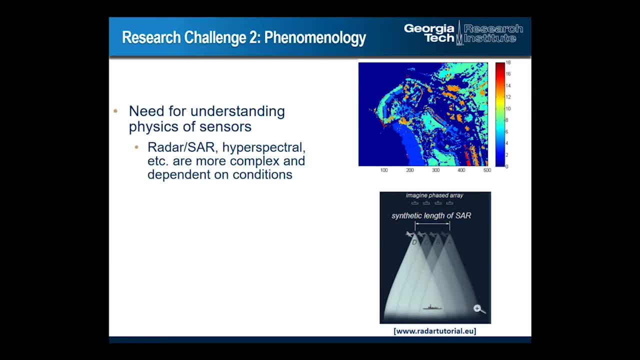 The need for understanding the physics of the actual sensors, as opposed to just images where we're just processing them without understanding the actual phenomenon For radar and other things. we have to actually understand that, And so we can actually design, And so we can actually design. 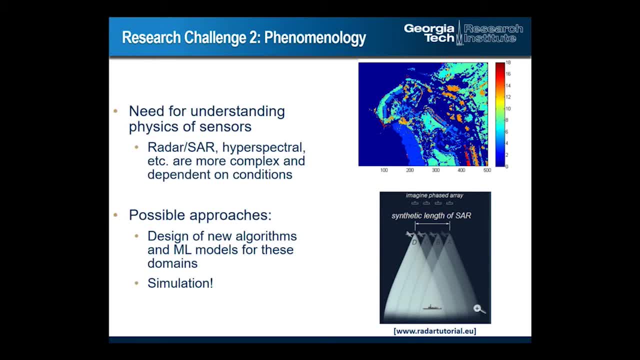 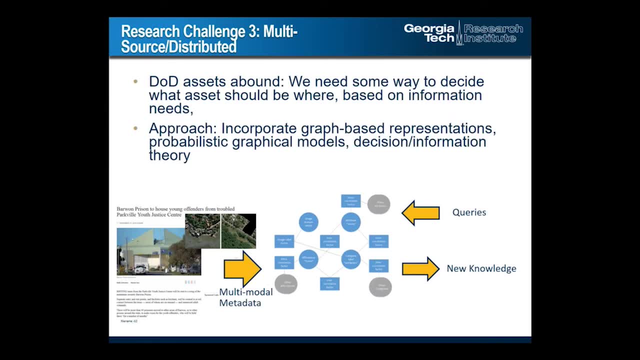 New algorithms and models that work on that kind of data- and we do as part of my research, And obviously simulation is a big part of that. where we don't have a lot of data, Multi-source and distributed is something that's been alluded to a lot here. 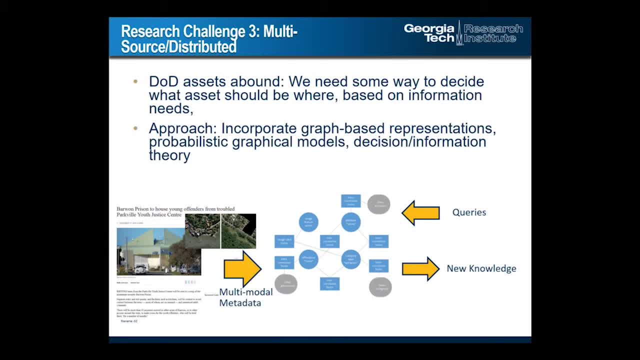 Obviously, you're not going to have one asset or sensor. you're going to have lots of different assets. You're going to have them distributed across an environment. And then there's the question of who talks to what and says: you know, transmit one information. 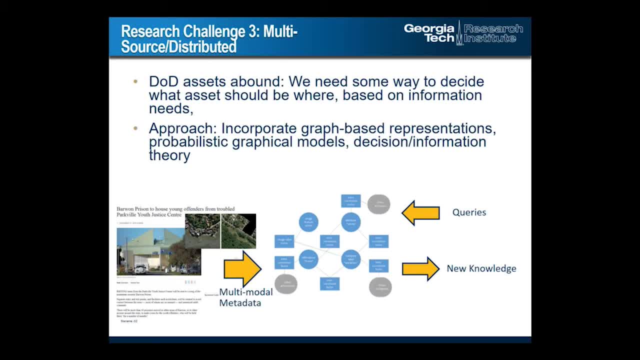 to generate a global, coherent picture of what is in the environment, And then also even decision making. So how can you automate the decisions of, for example, asset killing? or you know where to deploy these systems, which platform should go where to observe a particular type of thing? 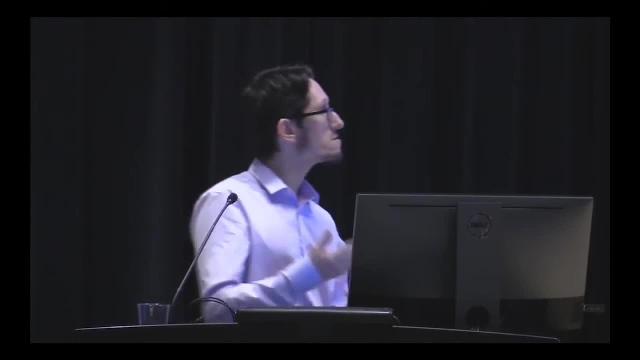 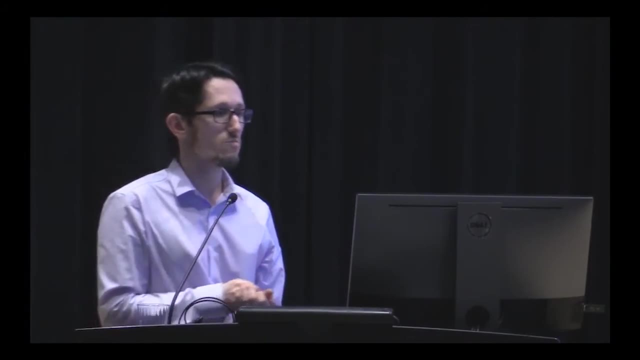 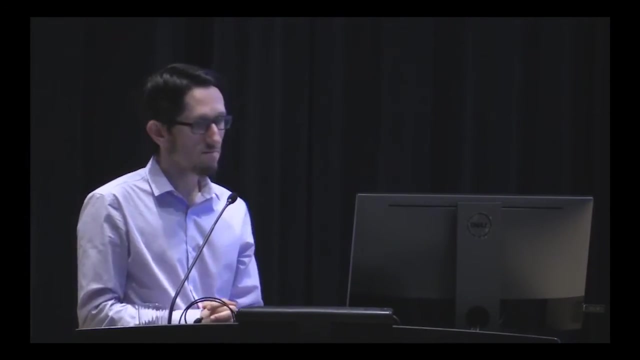 that you want to observe. So there's a lot of decisions there and I think eventually, definitely in the 30 year timeframe, these decisions are going to be automated, not some person. a person can't really, you know, understand, just like you know for normal flight traffic, you know. 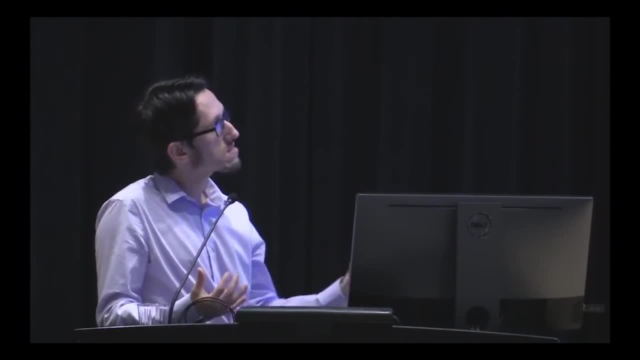 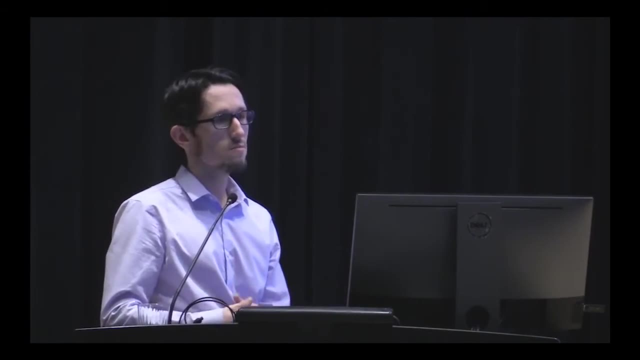 we have flight traffic controllers, but we have you know, once the complexity increases, such that you have different types of assets- air, ground, sea- you have different sensors on them, A person is going to have a hard time figuring out what asset to send where, and you also. 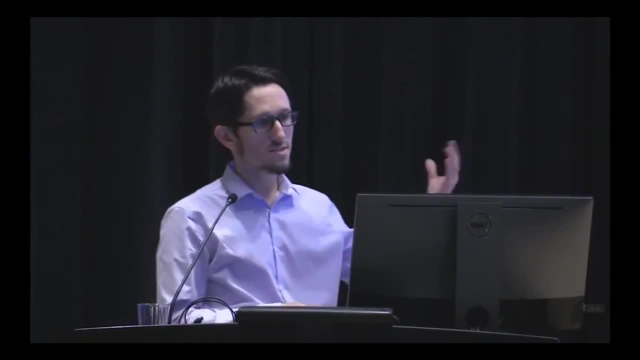 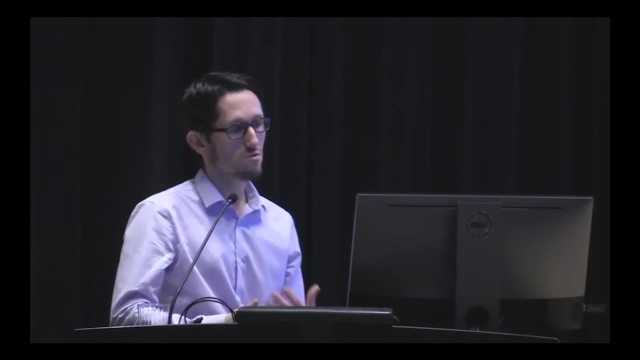 have resource management of. maybe one group wants these sensors, the other group wants the same sensors. How do you, How do you de-conflict that? So all of those decisions, I think eventually will be made automated in an automated way, And decision making. 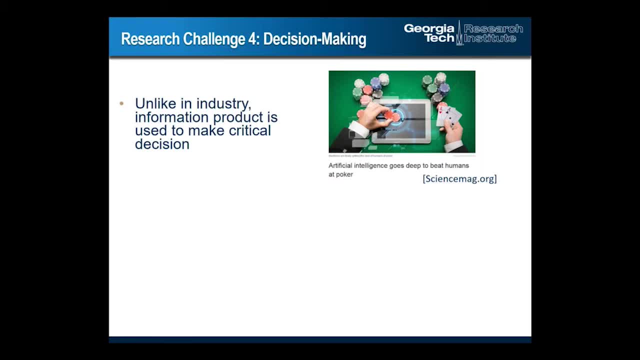 So there's a lot of things that you've seen in the news. Actually, just a few days ago, last week, somebody beat poker, So a computer was able to beat expert poker players, And what's really interesting about this game is, unlike chess and go, you don't have the 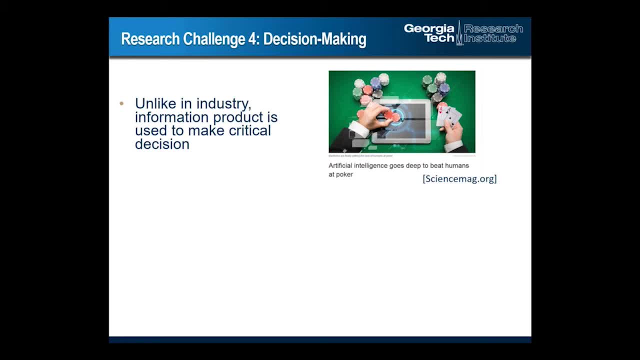 full state of the system. You don't see the whole board, You don't know what that person Has in terms of his hands, You don't know whether that person is bluffing or not, And so it was still able to incorporate imperfect information to do better than a human. 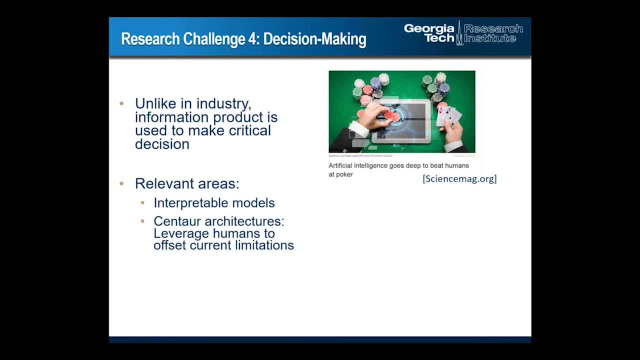 And so this was already mentioned, but this kind of sent our model where we essentially leverage humans to kind of offset the current limitations of these AI machine learning systems, of which there are many. I know again, there's a lot of hype. not none of these systems are perfect, but really. 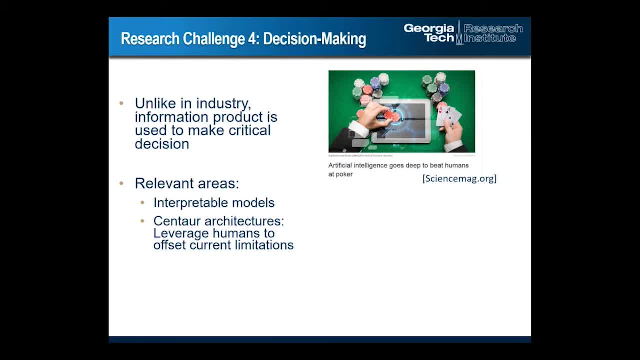 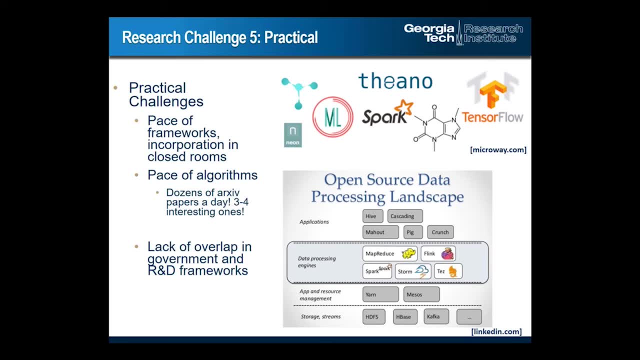 I think, Combination of humans, These systems can actually do a lot better than just the systems themselves. And then there's a lot of practical challenges. So even with respect to research, there's about 20 papers a day that come out 10 minutes. 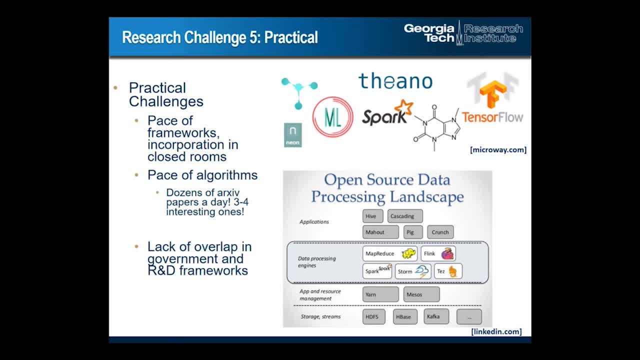 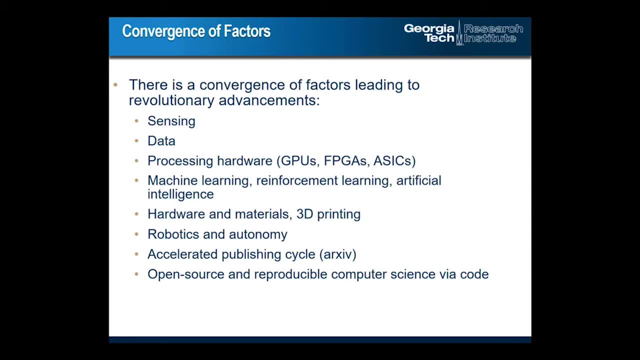 Okay, I'm going to skip this less interesting thing. There's a lot of practical issues of how to actually deploy this and do the pace Okay. Implications for the future. So clearly there's a convergence of a lot of different advances in sensing data processing. 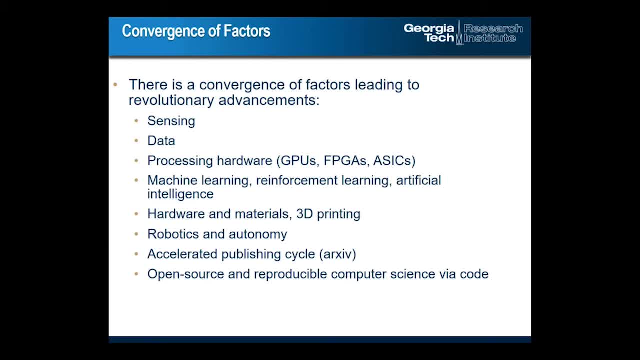 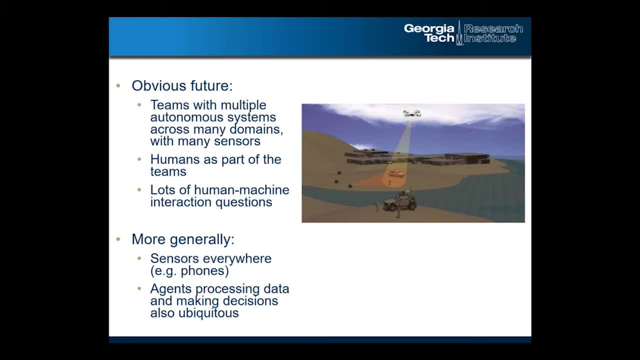 robotics and autonomy, hardware materials, 3D printing- all those things are all coming about and allowing us to have, for example, in the obvious case which a lot of people have also mentioned, we're going to have- multiple teams with different domains, different humans. 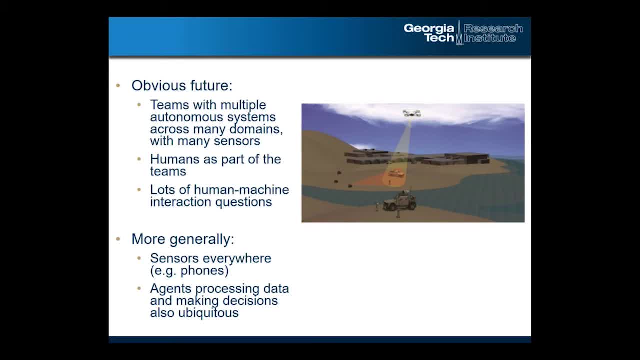 as well. Humans will be part of the team And then, more generally, we'll have sensors everywhere. So a lot of what we've talked about is actually DOD assets or things like that, but literally everybody has a phone that has 10 to a dozen sensors on them. 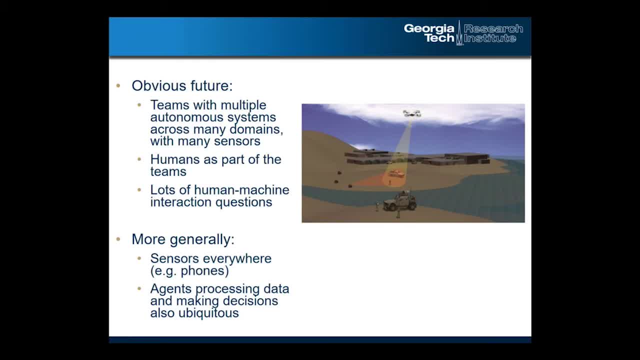 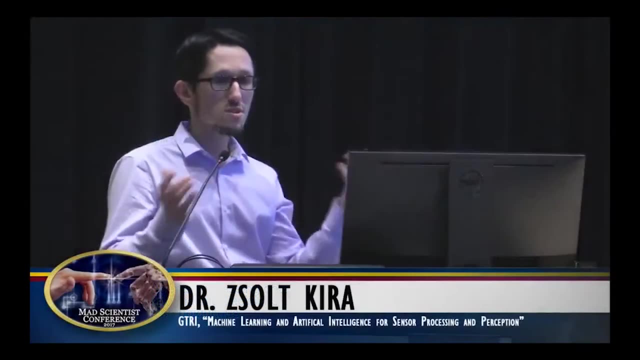 And really at some point with this internet of things, you'll have basically pieces of the environment across the whole world being observed by lots of different sensors, And there's a lot of question of how you process all this data. How do you answer a particular question that you're interested in using all this information? 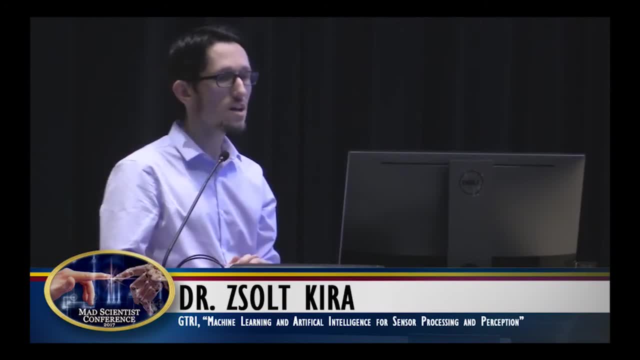 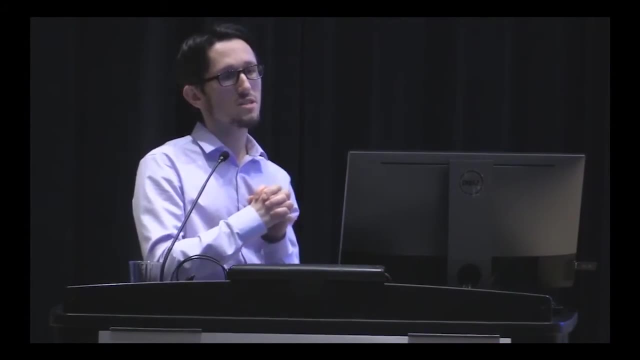 I envision basically a bunch of automated agents constantly processing all this data, indexing it, making decisions about which data to process and so on, And you literally give it some query and it can hopefully integrate all that information. If it doesn't have information, automatically decide where to get that information which. 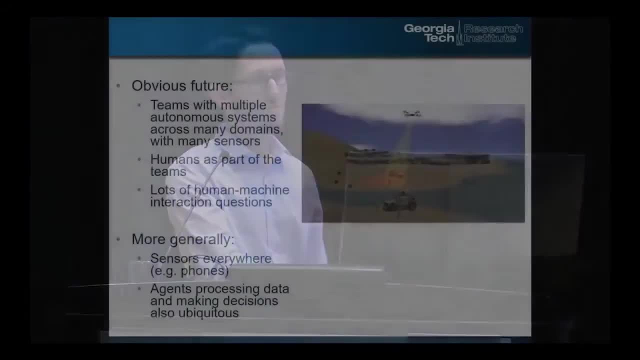 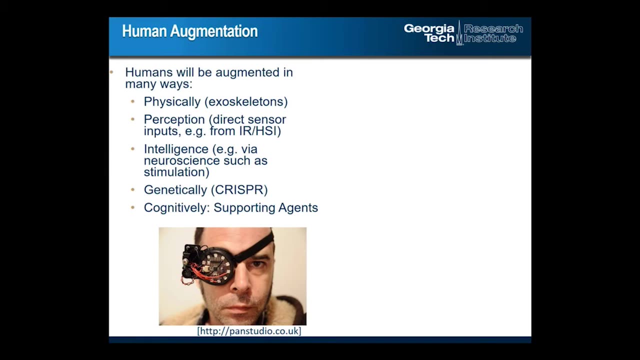 sensors to go to and process it and automatically give you the answer. One thing that hasn't been mentioned- I saw it on one slide- is human augmentation. So obviously the flip side of having fully autonomous systems is actually robotizing the human and a little bit scary, but there's a lot of things that you can do. 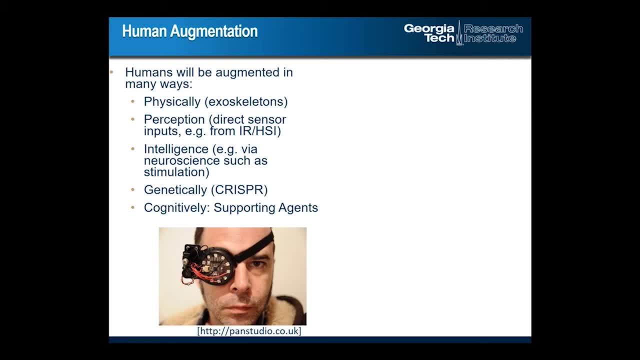 right Exoskeletons, perception augmentation, intelligence augmentation that other people are working on, And really again this cognitive support agents, such that you literally have an autonomous system, not a physical system, but something that's constantly grabbing data and information. 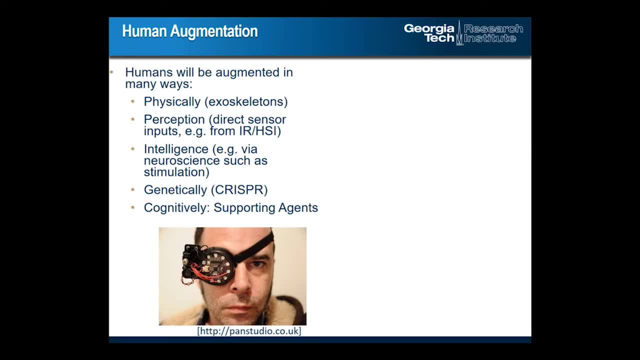 from different things, such that you can literally just focus your brain on the more interesting questions, And if you have a question such as when did a blue Ford go by this particular location, it can just answer that question for you immediately. You don't have to look through the data. 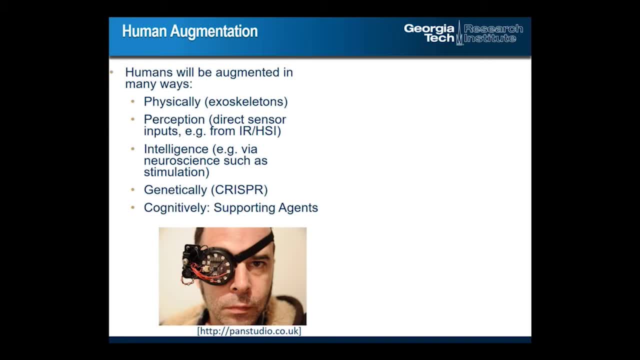 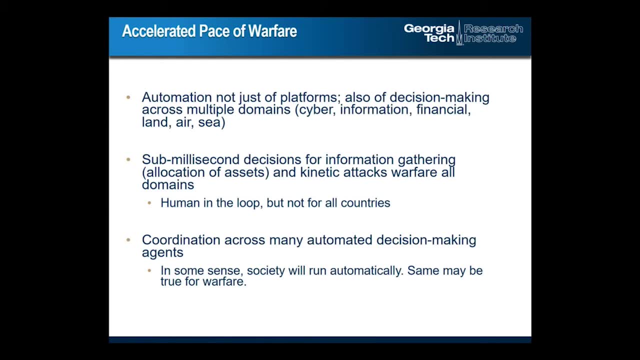 So you can just kind of piece together more of the higher level strategic cognitive things that you might want to. One thing that people have been talking about here as well is acceleration. So obviously once you go to learned and automated decision-making, then that decision-making- 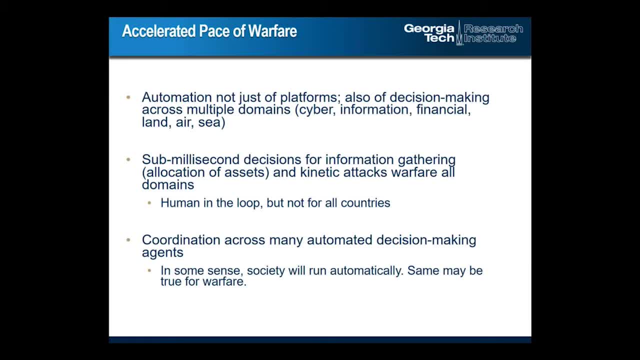 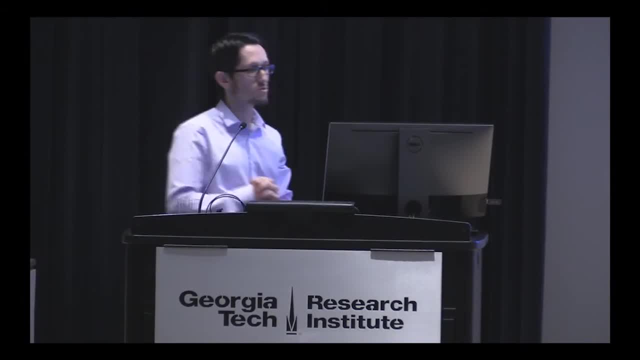 it's going to be faster, Yeah Yeah, Decision-making is very fast, sub-millisecond decision-making, And so really one thing is: humans will be in the loop in the foreseeable short-term future. However, in the long-term future, it's not clear, right. 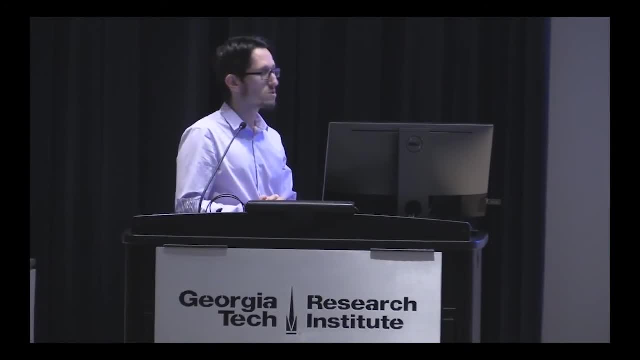 And one interesting thing is, different countries are probably going to make different choices about this, And really, again, coordination among many decision-making agents is kind of the next step as well. So, similar to how you'll have multi-robot systems out in the field, you'll also have 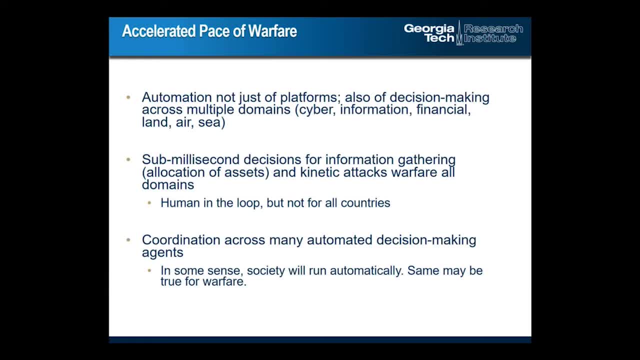 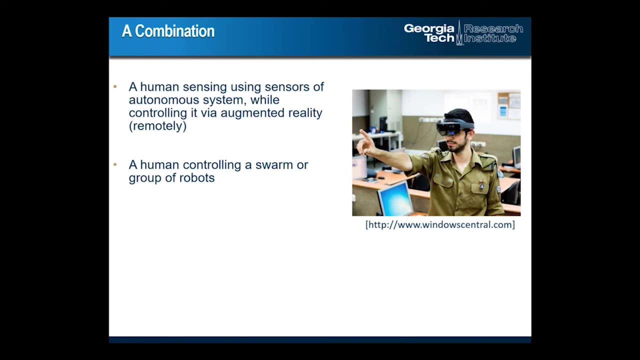 multiple Autonomous agents working on processing data and making decisions in an automated way, maybe perhaps in a coordinated way, to produce an effect that is more powerful than just a single agent that can do. And again, a combination of humans and these kinds of things is very, very likely, I think. 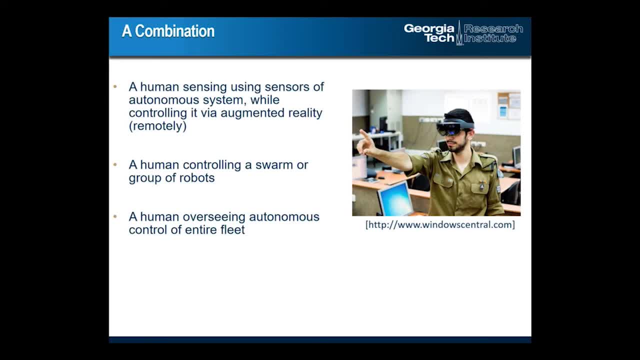 So, for example, a human controlling a swarm, a human overseeing autonomous control of entire fleets. This has been mentioned as kind of this Oculus Rift augmented reality type of things, where you may, for example, have the person actually looking at sensor data from the actual autonomous 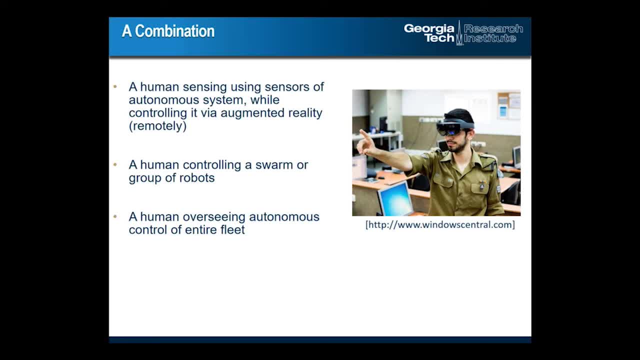 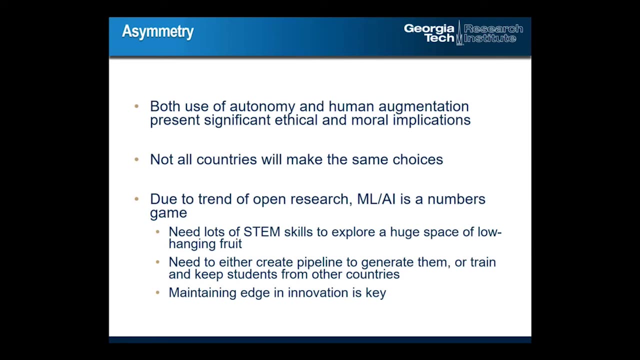 system and controlling that autonomous system simultaneously from a location far, far away, And then that's the ultimate goal, where literally, you don't have to think about anything except for the high-level objectives and goals and strategies that you actually care about. One thing that I do want to mention is asymmetry. 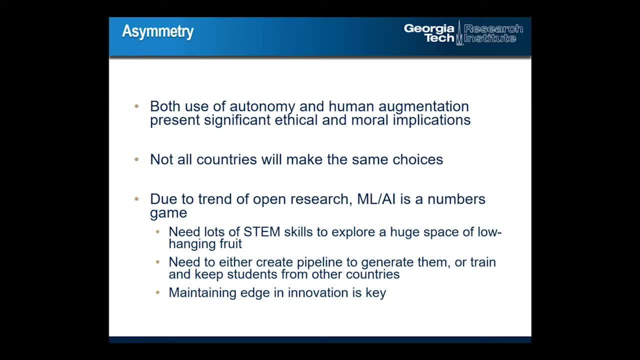 I'm not sure if you're familiar with asymmetry. I'm not sure if you're familiar with it In the sense that both use of these kinds of things. there's a kind of ethical moral blurriness to a lot of these technologies that are coming out. 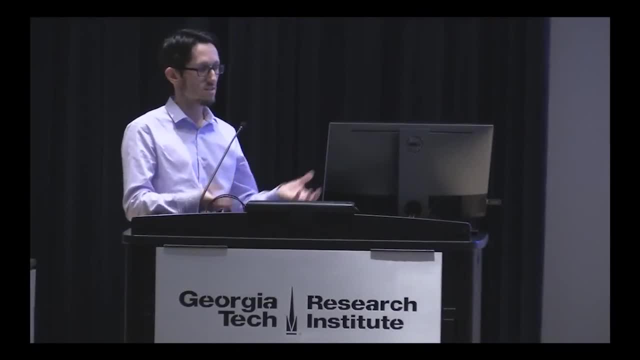 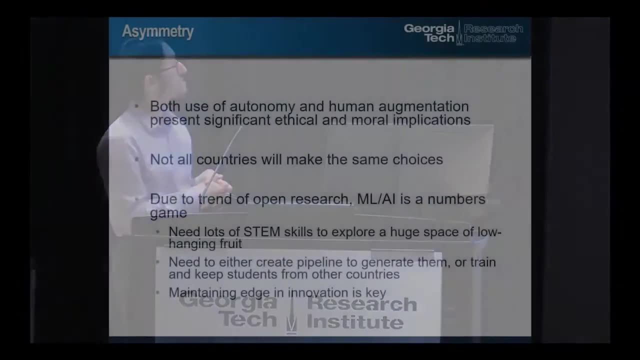 And obviously different countries are going to make different decisions And so that might present an asymmetry. And I really want to emphasize the bottom point, where there's a lot of articles where the US is right now ahead in terms of artificial intelligence and machine learning mainly. 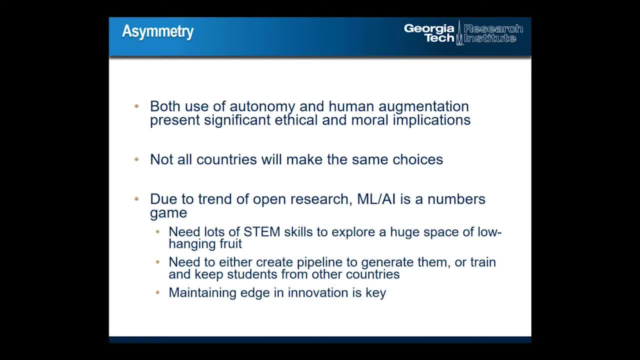 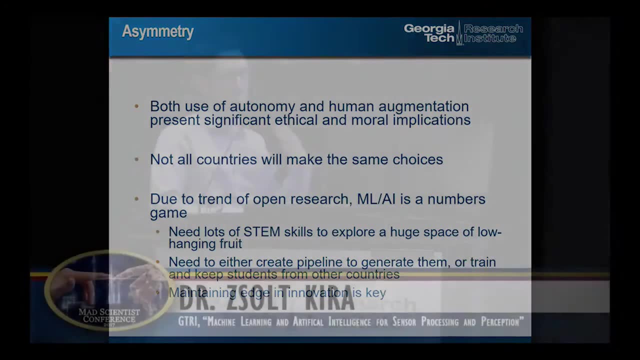 due to our universities. I guess I'm a little biased, though, But that might change. So a lot of these things are coming out open source, are published immediately, as opposed to at conferences, So literally anybody can take these algorithms, anybody can run them and expand on them. 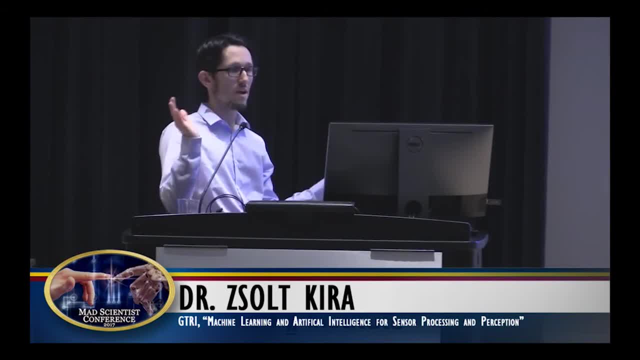 And a lot of this will be a numbers game- where literally there's such a huge low-hanging set of fruits everywhere for these upcoming systems that literally you just need to get your hands dirty. You need bodies, But you need bodies that know salmon. 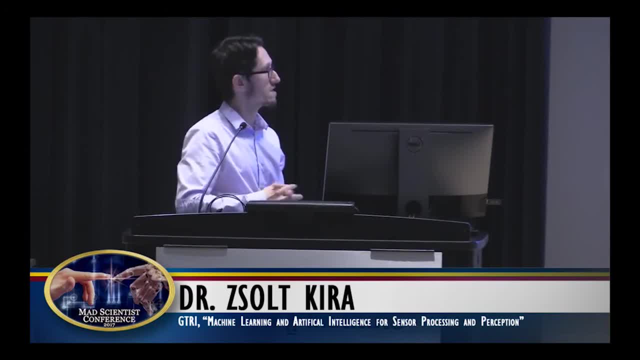 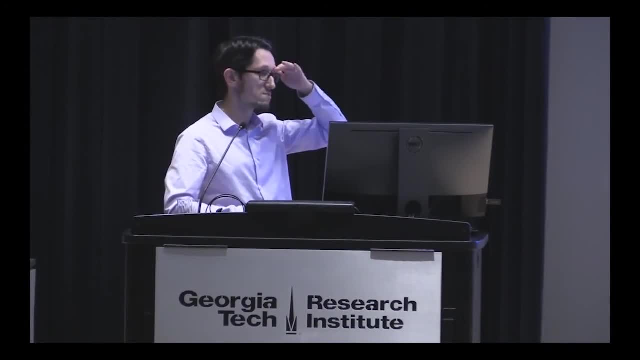 So I think one of the key things- and again I'm biased because I'm trying to hire people who are skilled in this area and it's really hard- And so I think definitely a lot of thought needs to be put into producing a pipeline. 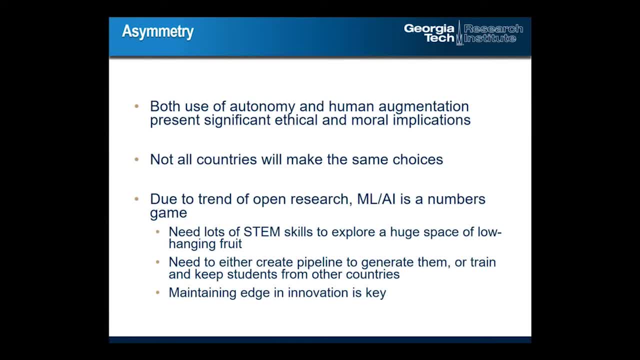 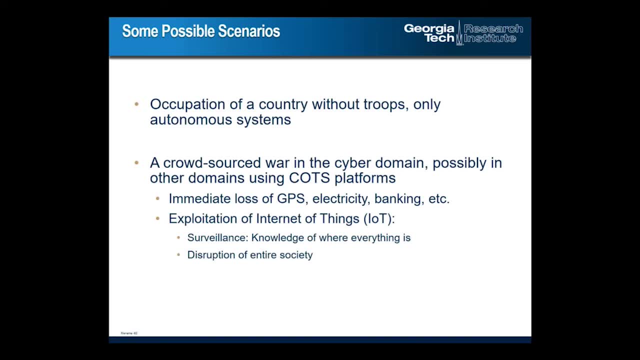 of people that are good at these kinds of things like information and data processing and machine learning and artificial intelligence. And then here's some interesting possible scenarios, Especially at the bottom- At the bottom, where a lot of this has been alluded to as well- where you can have effects. 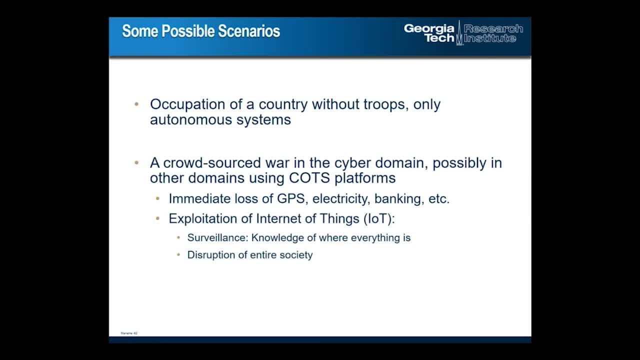 that a random person in the basement is actually producing- in terms of cyber, but also, eventually, in terms of physical things. So once autonomous systems and UAVs become cheap enough, anybody will be able to buy a swarm and deploy it and throw it and take open source software, put it on there and 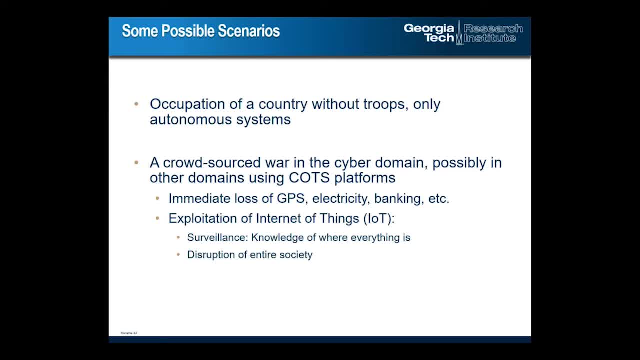 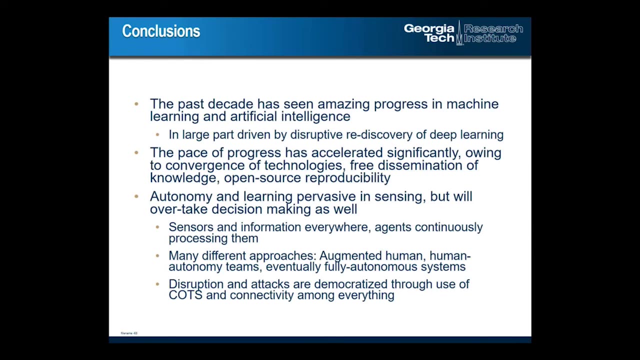 have it fly autonomously and do things that they want. So that's a very, Very kind of disruptive thing where anybody, any Joe Schmo- can basically create disruptions using a lot of these technologies. Okay, That's my conclusion. So basically, the past decade has seen amazing progress. 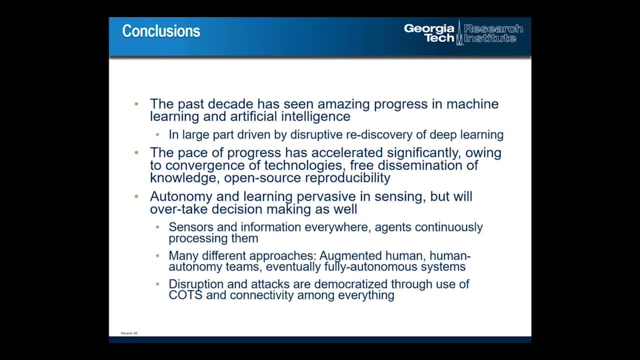 And again, I would have never been able- and a lot of people haven't- would not have predicted the amount of progress we've made in the past five years. in large part is driven by machine learning and AI algorithms, And it's rediscovery of existing algorithms, not really development of new ones. but there's 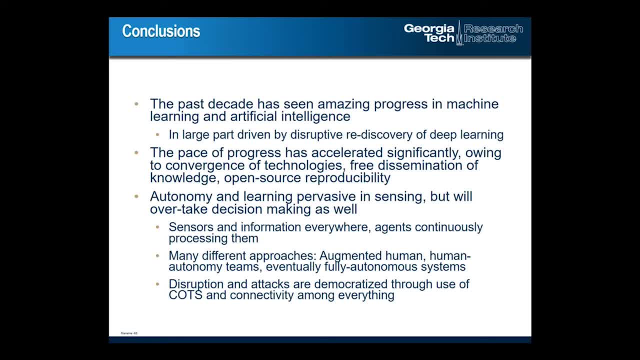 some additional understanding we have. The pace of progress is just immense. I have trouble keeping up with the latest papers myself because they come out 20 at a time every day And everybody's putting their papers online, everybody's putting their source code online. 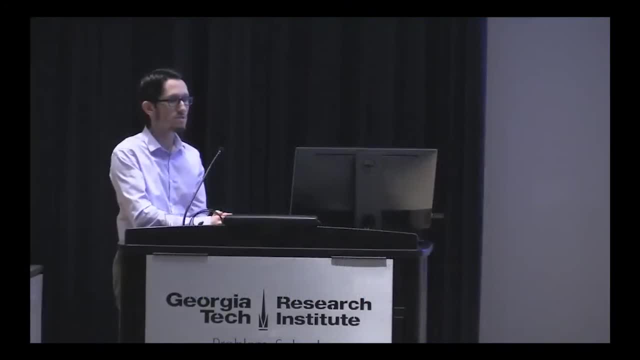 So literally it's not just restricted to the people, the labs that are developing them. Anybody can Across the whole world, can take these algorithms and do trial and error. So I think that's a great point, Thank you, And if you can do that, you can try them out. 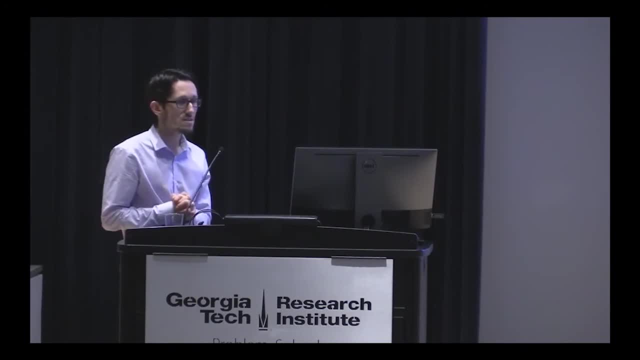 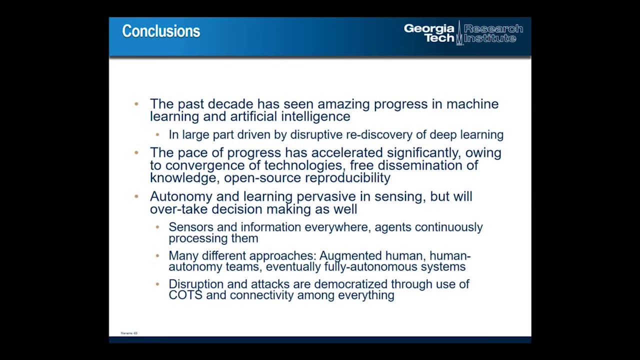 And then autonomy and learning is pervasive. It's sensing right now. however, it will be pervasive in decision-making as well, And so you're gonna have sensors and information everywhere, not just the assets, but across the entire society. You'll have many different approaches: augmented human. you'll have human autonomous teams. 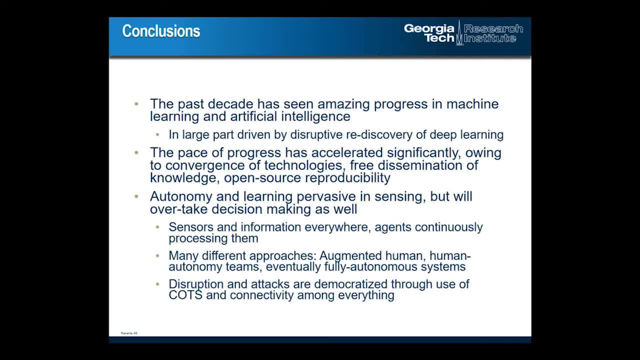 And then, eventually, once I think I'm a fan of basically proving out- Okay, Okay, Thank you- human autonomous teams and testing out autonomous, full autonomy, and demonstrating that it is better or safer than what the human can do. and once that becomes true- which i think, we're nowhere. 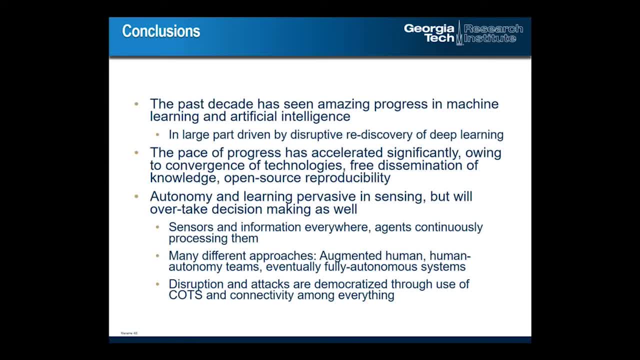 near right now. um, then we can think about fully autonomous systems. um, and again, this kind of disruptive kind of set of things where machine learning and ai is now democratized. everything is off the shelf. um, to some degree, unless you're getting research and innovating. it's just you. 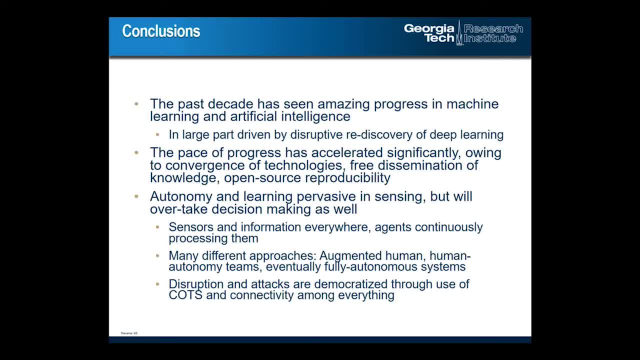 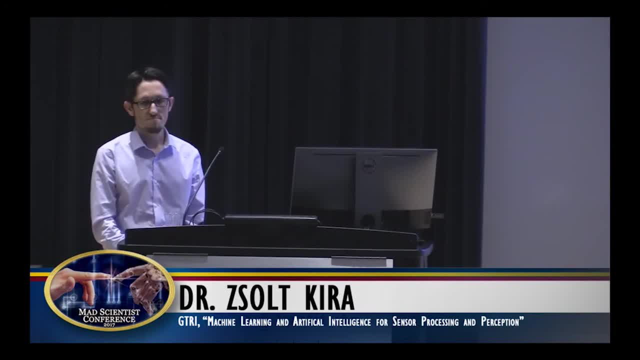 download it off the shelf and you can try these things out. so there's a lot of disruption that can come from that and that's my conclusion. thank you, if anyone has any questions. uh, yes, so you mentioned. you mentioned that nobody could predict in, say, 2005, 10 years ago, that neural networks suddenly the despised 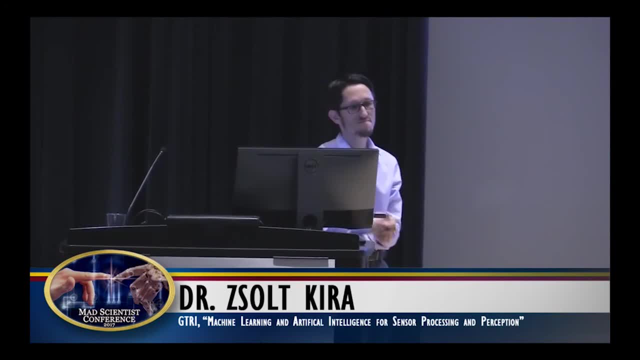 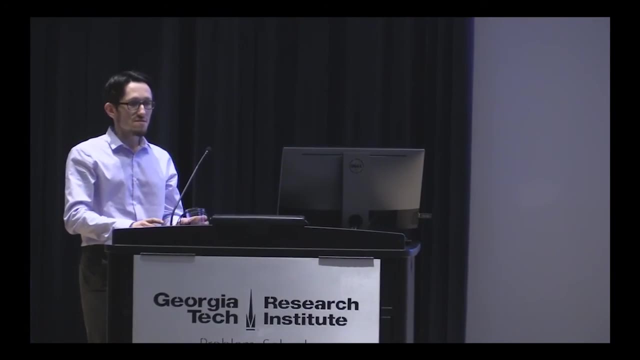 neural networks, which were. you know, the papers on neural networks were automatically rejected from many serious journals. and now it's the opposite: you can't if you have a paper without neural networks exactly, and so what is so 10 years? who could have predicted what happened in 10 years? 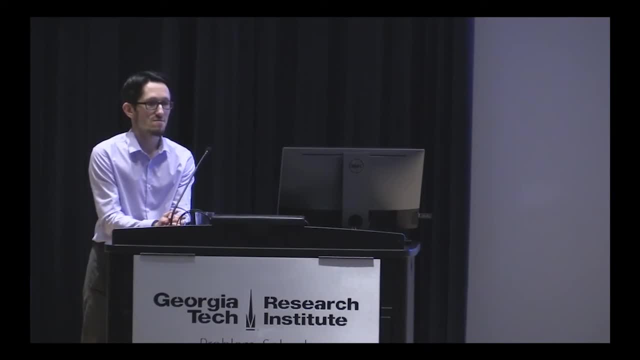 so could you take a guess what will be that despised and underappreciated technology of today that will make the breakthrough 10 years from now? um, that's a difficult question. so there is one class of algorithms that this kind of the sister to deep learning, which is neural networks, which is 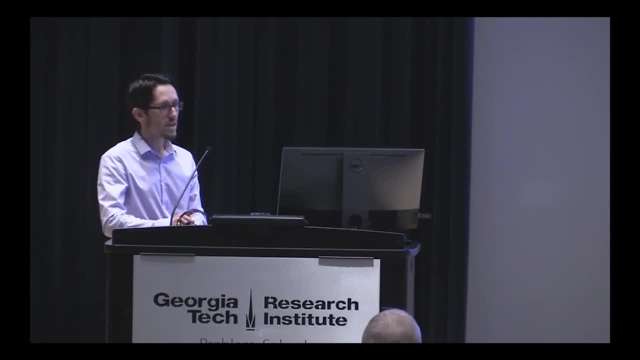 probabilistic graphical models. um. so deep learning again, is good at individual tasks, but putting together multiple types of information in a way that respects your uncertainty around that information, which is what probabilities do, um, is one class of models, and these class of models we use heavily, but they're 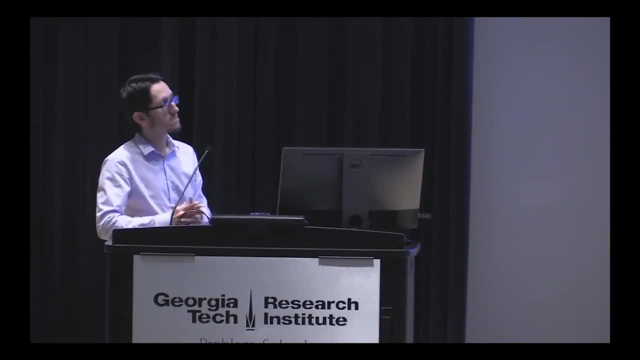 very, very slow, and so they're hard to actually deploy in real world systems. so i think there's going to be a lot of effort in terms of making those inference algorithms for probabilistic graphical models and similar kind of methods as well. another one might be, you know, there's another. 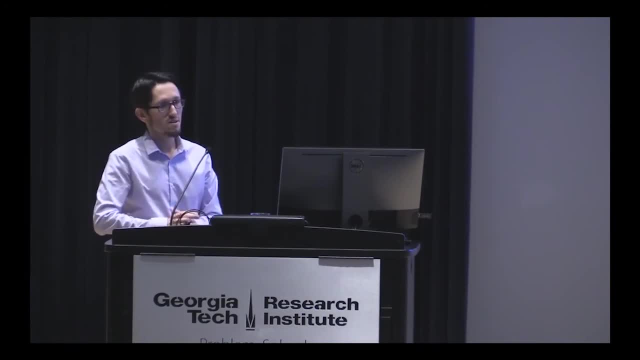 class of despised models which is kind of the more logical prologue type models which you know. now we have probabilistic variance and things like that. but you know there's a lot of work to be done to use these algorithms and things like that. right now i think they're still not, you know, very heavily. 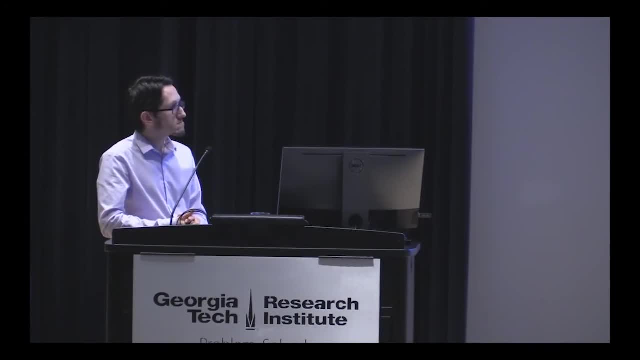 used. but you know, eventually i i think somehow, um, you know, there's a whole um kind of field now of understandable ai, right? um, so darpa is doing a project explainable ai and so on. um, and really, i think you know, one language that people can speak to is um logic and at least natural text. 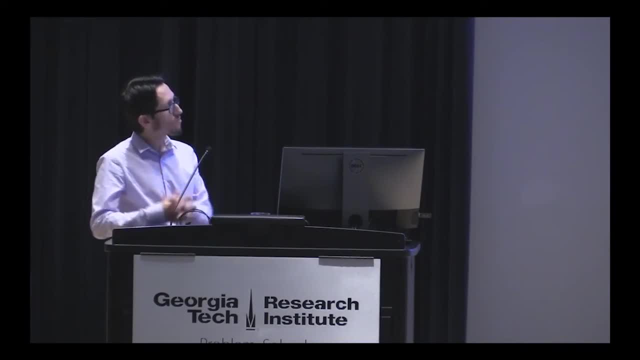 understanding in other kinds of forms these algorithms to those natural forms that humans can actually understand and trust. um that these methods are making good decisions, i think, is another area as well. a lot of these um machine learning algorithms rely on bayesian prior probabilities. so how do we? 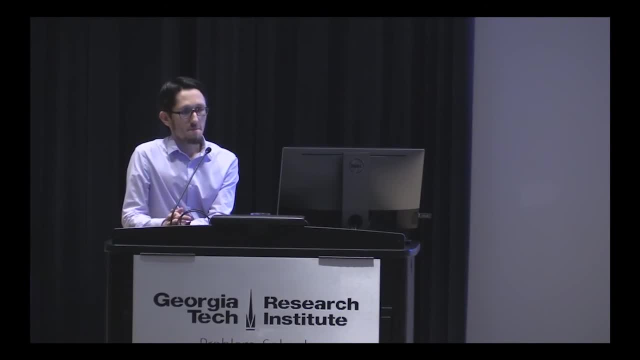 validate bayesian prior probabilities, especially for unknown situations? i do not have an answer to that. no, i i agree. so that's? i mean the problems, the graphical models? uh, yeah, a lot of them, and not only that: the priors are typically represented as gaussians and things you know you're making. 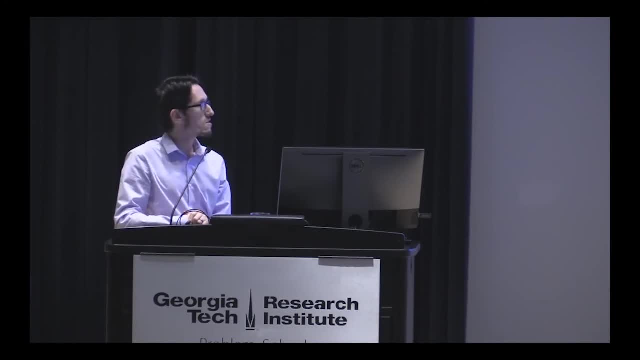 parametric actual model assumptions that are very strong, um, and how you learn that from data. i yeah, i mean, i think that's a very difficult question and that kind of also relates to the question of kind of how to do that using unlabeled data especially. um, yeah, so that's, that's a valid 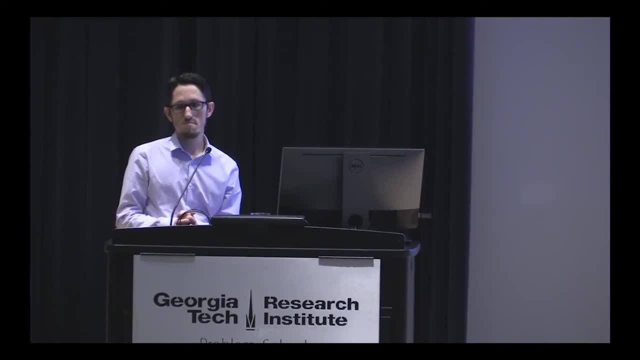 question: how do you take the uh situations where flippin has had denial deception aspects? so you have to use your algorithms and artificial intelligence to make either the human or the system think: instead of one soldier, they see a million, or instead of one tank, they see 20.. 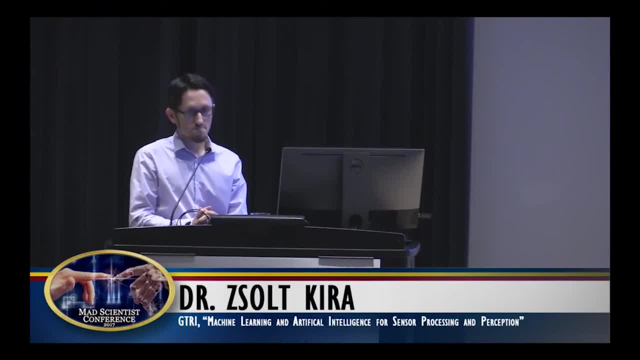 so that, basically, whether it's holographic or other types of projection, how do you, is there any research in that realm going on? i guess to, to given an ai how to produce data that kind of makes it think it's something other than what is the reality. 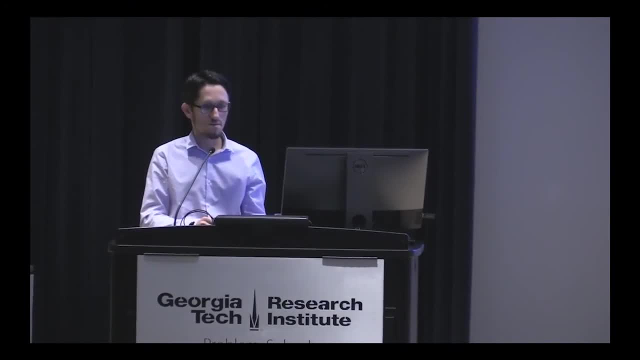 is that way. yeah, so there is a class of, yeah, um, kind of open, uh, literature that is looking at what's called adversarial machine learning. so pretty much again, neural networks are very good, but they're very they have their problems in that, for example, you can change the pixel data. 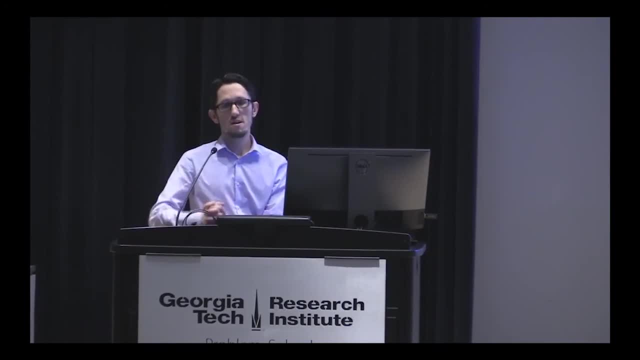 in a very particular way, such that you can make it. i think it's one object versus the other, um, so they definitely have their weaknesses, and people are are starting to look at that a well, and not just how to how to how to come up with examples that fool them, but also vice versa. 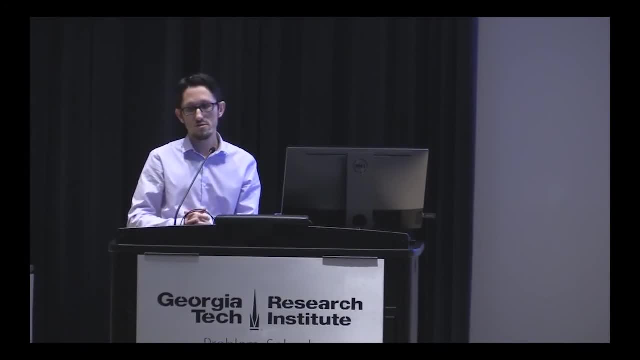 how to make them more robust as well. so that's definitely a concern. yeah, okay, you hear me. yeah, so i'm going to try to ask you a question and maybe offer my take on your question. uh, your question was: uh, what's not going to be over the what's if you submit today? what? 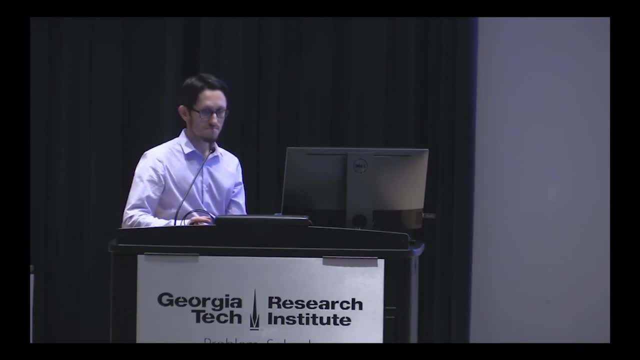 should be accepted that. my take is: uh should be considered the way neural networks were in the past 10 years, and i'd like to get your take on. it is, um, quantum computing, and particularly in a reach now, uh, kind of computing married to ai. what's your thoughts? 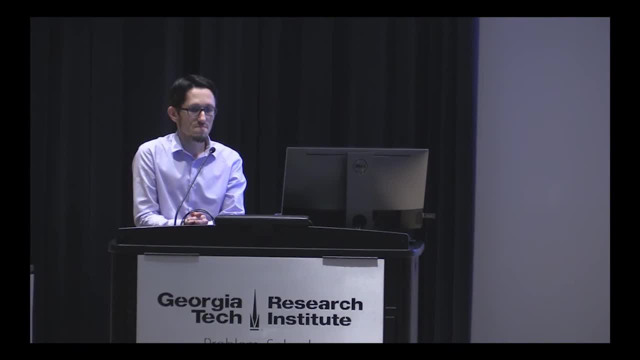 on that, because i'm posing that as a challenge for our, our 2030, 2020 or before, absolutely so i, i, I think you know, I think you mentioned this yesterday as well. I mean, there are, you know, recent headway made in quantum computing, including Google and a little bit D-Wave and those kind of companies. 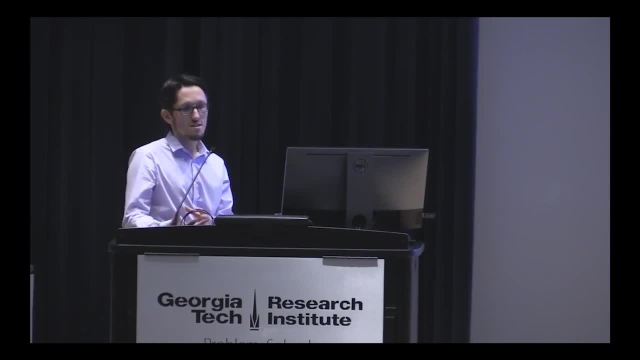 I think it's a little bit too early for me to be able to tell kind of which AI or machine learning algorithms will they actually be able to speed up right? So I think there's not really a compelling use, a compelling kind of case where right now the quantum computer can solve this X problem faster than a classical computer, right? 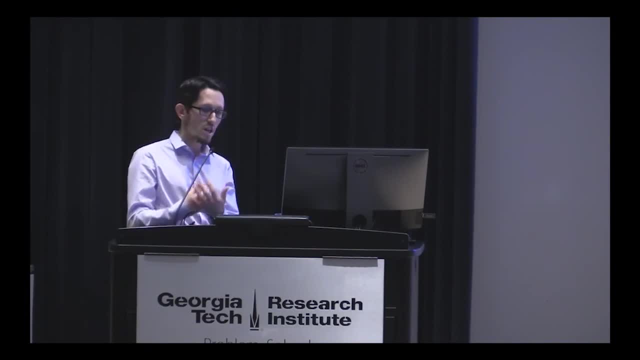 But I mean, I foresee that that will kind of flip and change. And then the question is really which machine learning algorithms you know? if neural networks aren't sped up by quantum computers, then we might be in trouble. We'll have to come up with new machine learning methods just for that right. 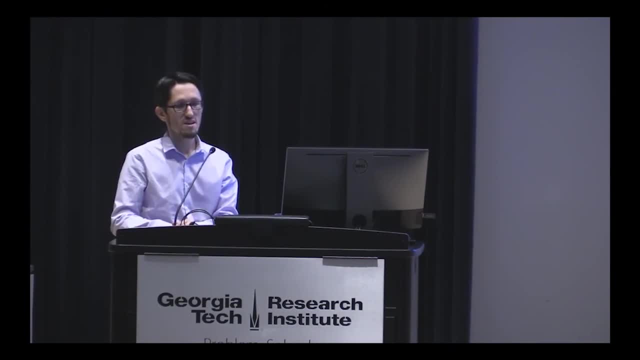 And also There's a whole host of implications, right Ranging from not just you know what algorithms should we use, but how do we actually program them. And you know, as a computer scientist, I know how to program current computers. 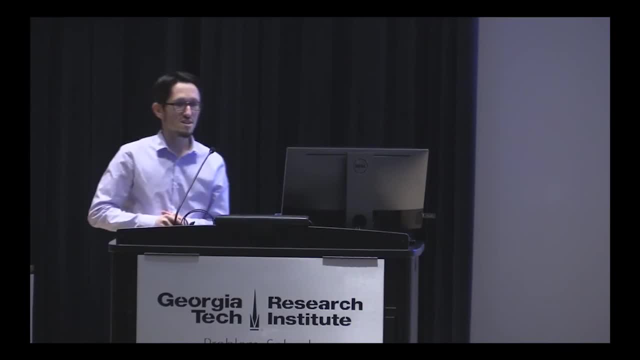 I don't know how to squash wave functions and all those different things. So you know, there's going to have to be a whole different like paradigm of how people actually program these things once they actually become. So yeah, I mean to me I don't know. 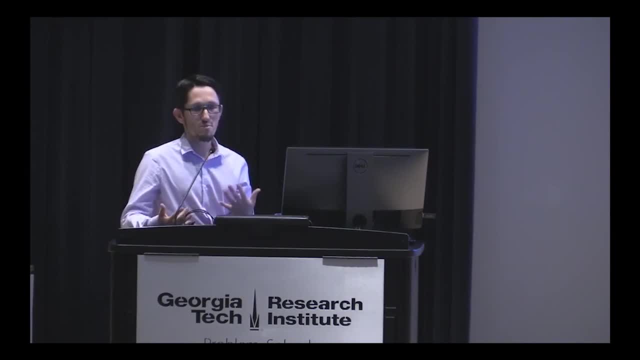 I would assign a probability or a chance to that, But you know it's probably more than 50%. Yeah, But I don't know that I can be very accurate. And what is the chance that quantum computers will actually come to fruition and actually show that it's faster than classical computers? 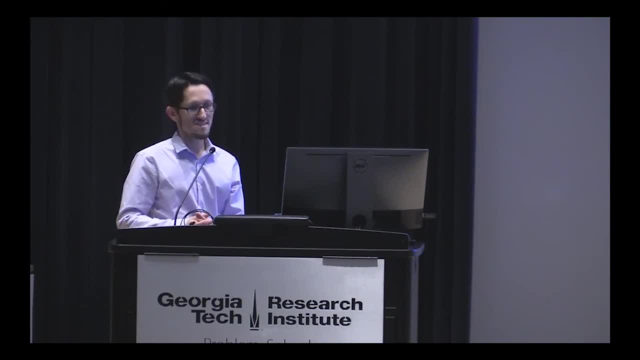 Yeah, Maybe. Yeah, That's mine, Sir, question over here. You mentioned some of the problems with the lack of label training data. I was curious if you had seen any of the Christopher Ray's group at Stanford. They've done distance supervision as well as factor graph. 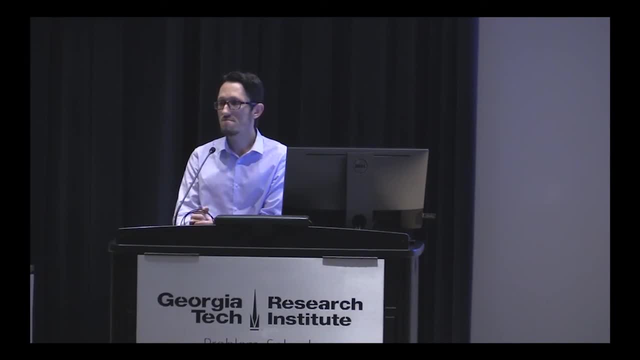 I know that's worked well in text. Do you think that could apply to? Do you think that could apply to imagery, video that really robotics needs? So that is what we're applying. Oh, okay, Yeah, So the example of what I showed you, where we have news articles with text and images and videos, and then also maybe satellite imagery, if you can localize the article. we are leveraging deep dive, which is Christopher Ray's group work, where you can use again probabilistic graphical models to basically integrate multimodal pieces of information. 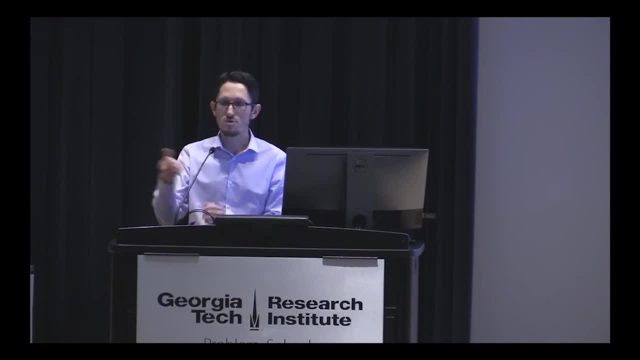 And that's kind of early work that we're doing. We haven't published anything, But yeah, I completely agree. And even in other domains- in computer vision, probabilistic graphical models and factor graphs, for example, for even just localizing a robot, factor graphs have also shown really their usefulness. 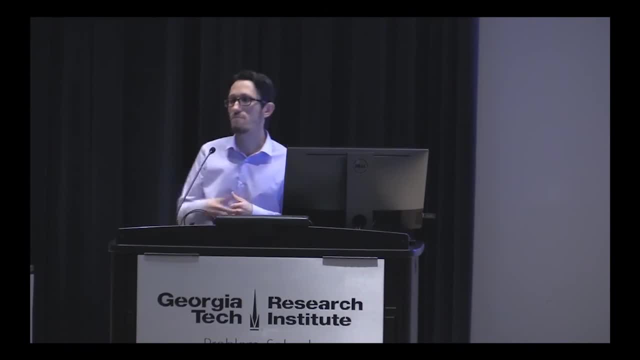 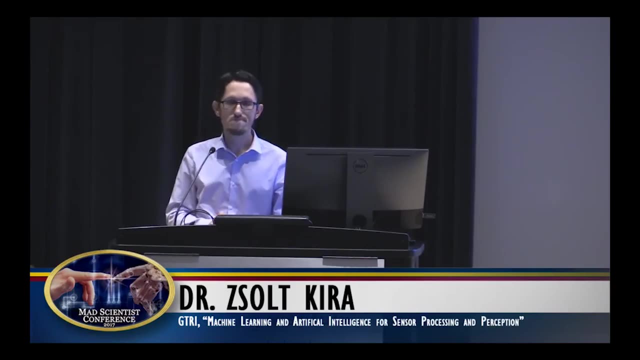 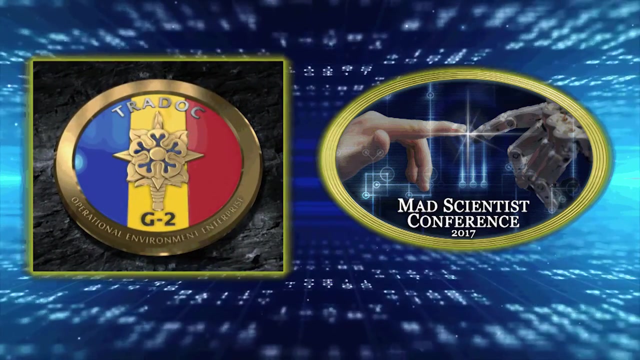